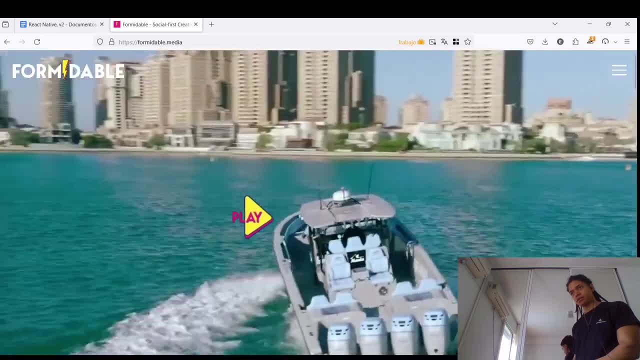 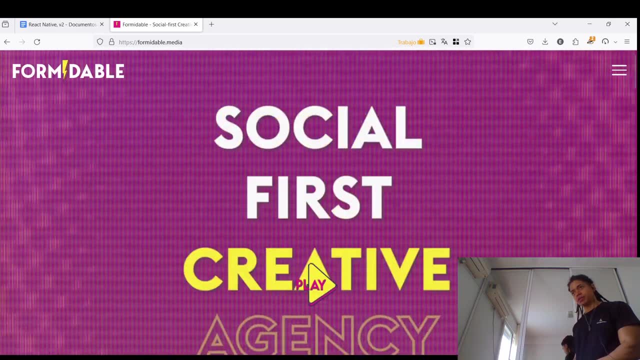 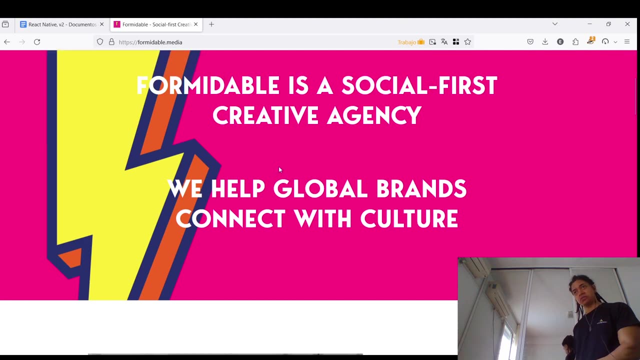 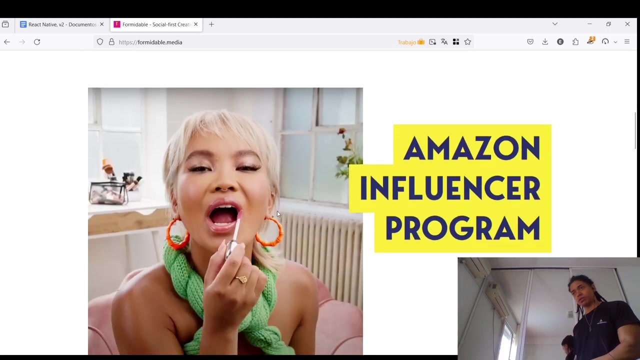 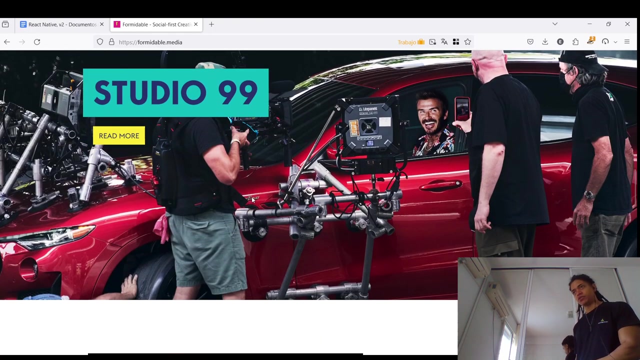 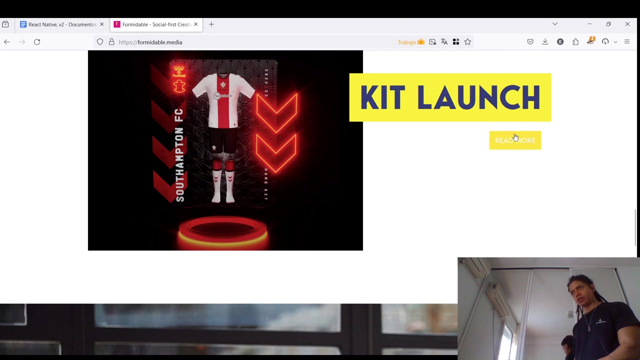 okay, like this, I think is this okay, like this, I think is this formidable, okay. so this agency that they have, okay, interesting, very, very interesting. uh, it's a social first creative agency. we help global brands connect with culture, uh, amazon influencers programs, uh. the other is studio 99. okay, and then you have keep launch here. i think this. 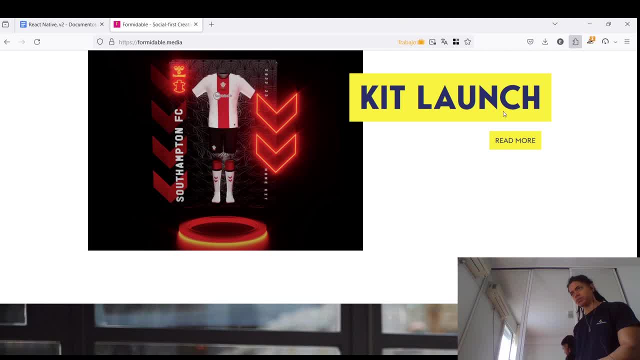 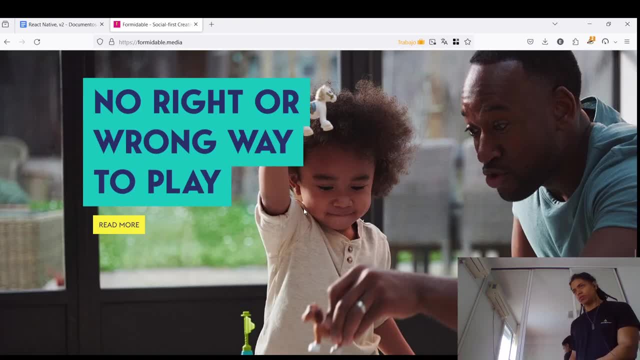 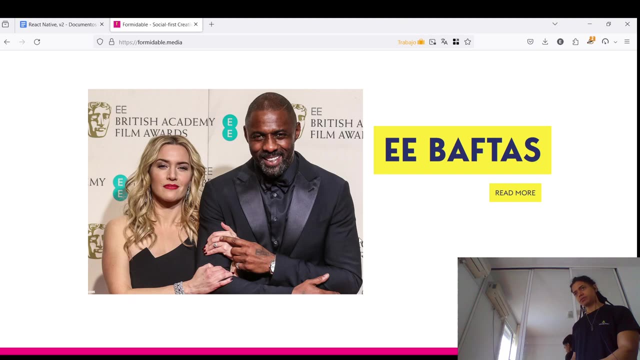 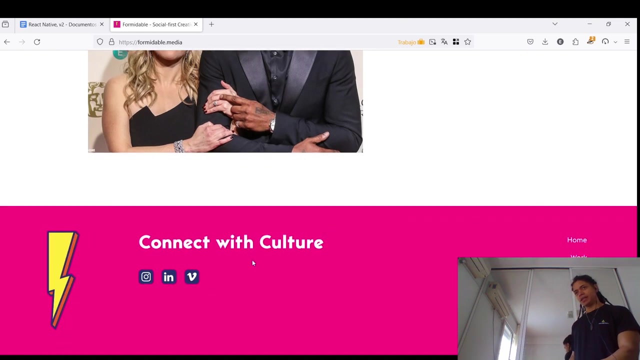 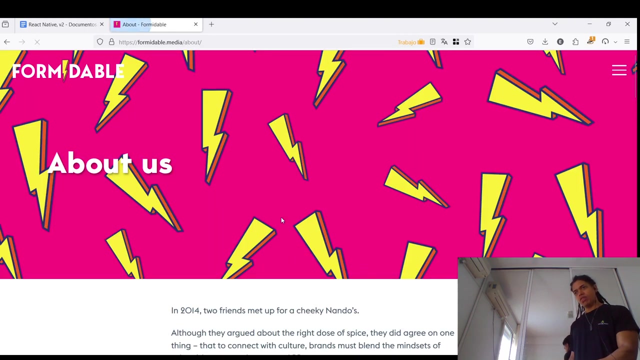 website must have been built on react or known wordpress maybe. yeah, wordpress, uh, not right or wrong way to play. like this. ee, bafta, like so, uh, he looks all, by the way, in connect with culture, right? so whole world about us? yeah, it's pretty simple. their website 2014 two. 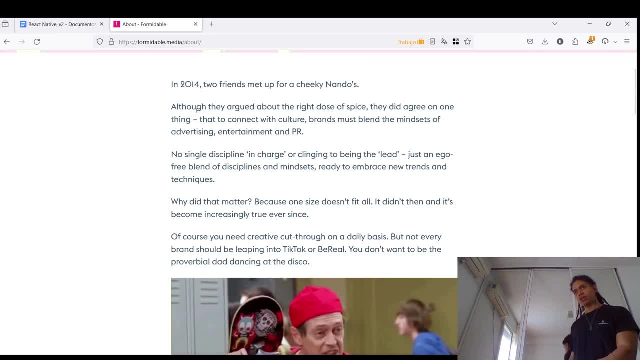 friends met up for a cheek nando's. although they argue about the right dose of spice, they did agree on one thing: that to connect with culture, brand must blend the mindset of advertising and entertainment. yeah, i'm, um, perhaps i'm quite more interesting in this particular field if i want to combine 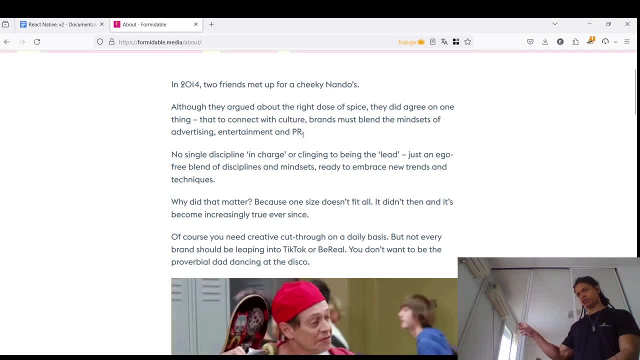 is not only my technical aspect, but with the social aspect, uh, and also, uh, talk about more polemic stuff or things that are relevant for anyone, any one of us. you know, in terms of the ai, how you use it and how i use it, and you know that i review these, uh, the some of the facts, and 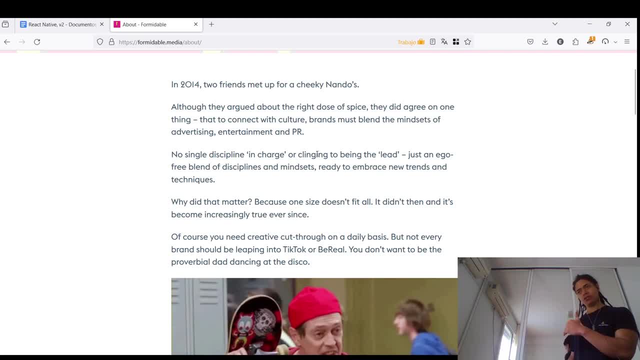 you know, i've been studying them for so long and that's just a yes. i think that that's true. yeah, we're going to keep up the pace. where are the things that we need to do, what our mindset and society must shift? uh, and also other existential threats, uh, like so, likewise, but yeah, so, no single. 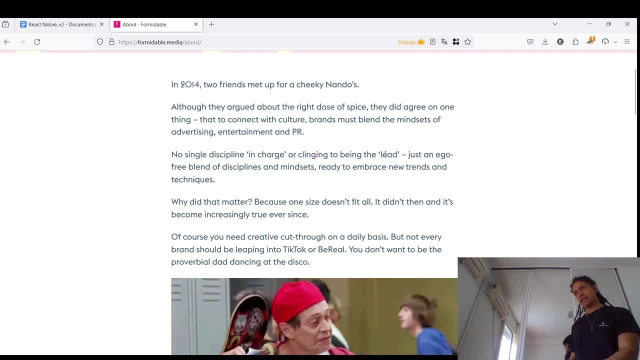 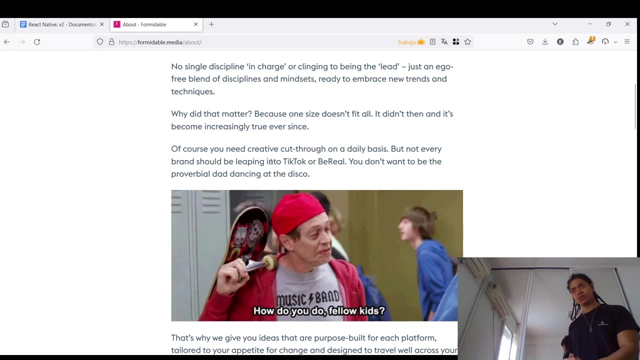 discipline in charge or climbing to be the lead, just an ego-free blend of discipline and mindset, ready to embrace new trends and techniques. that's one of the reason why i'm recording this kind of video is to recognize that not only, as for today's course, is react native, but also is the underlying technology. 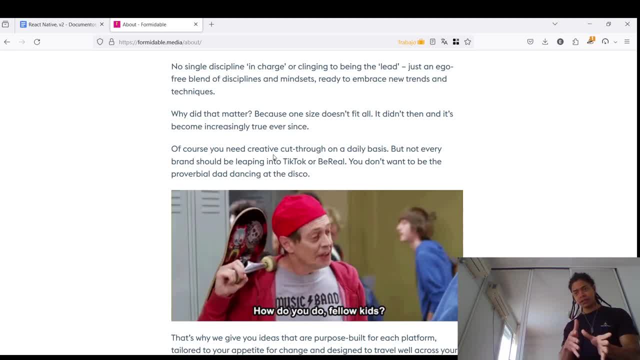 talking about is the hard skill combined with your soft skill. how important is to do this in your daily life, uh, and with uh spices, with a, with a, with a sauce of culture. because each one of those areas, the apartments, are important, so they are not isolated, so we share among that. they are blended as they. 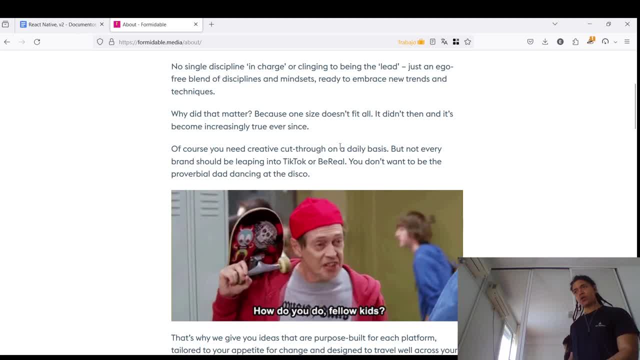 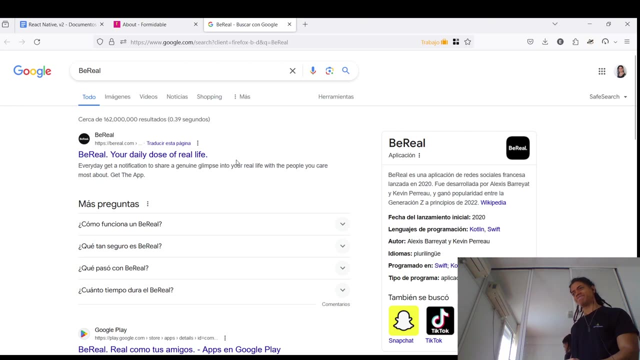 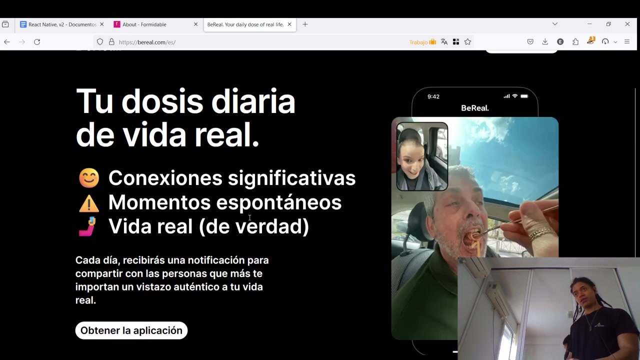 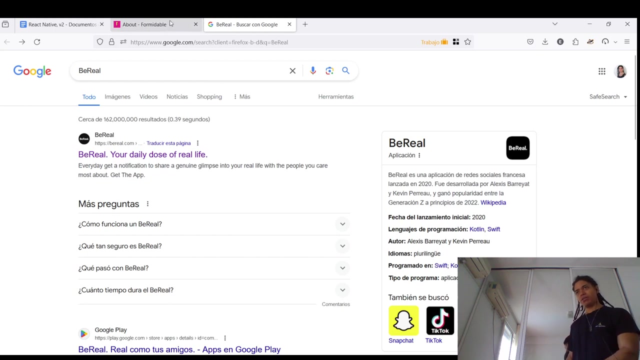 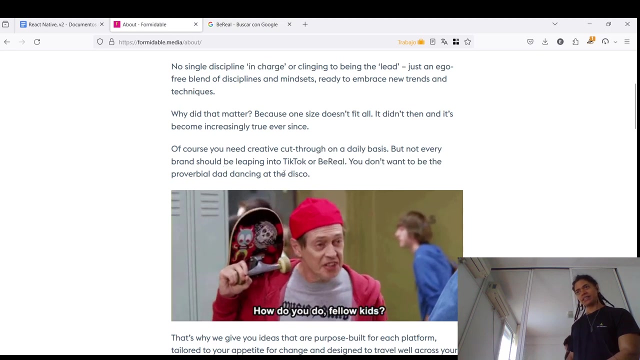 mentioned here. so of course, you need creative good throw on a daily basis, but not every brand should be living into tiktok, or be real. be real, oh my god. all right, what is french in french? okay? okay, they got this in spanish, french english. you know, what i want to say was cut short for a minute, so, but i take my word for it. 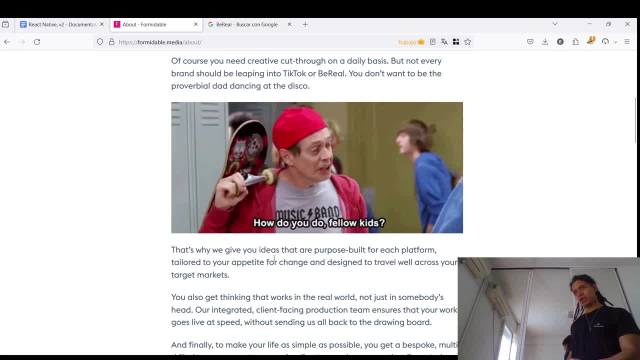 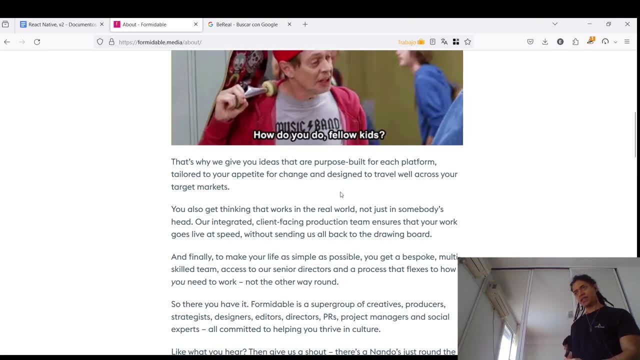 transverse. that's what we give your ideas, our purpose, purpose built for each platform. tell your time decade fresh this morning. the elections last. your target marketing is one of the reasons which drive this chart is that these are China heads is not a boutique who can do things same as channel projects, mode channels. the contכשels work for many in August. you're opening a market anyway. okay, so you don't want to be. you don't want to be, you don't want to be the proOUGH dands in at a disco. how do you get a fellow kids? that's why we give you ideas are purposes. 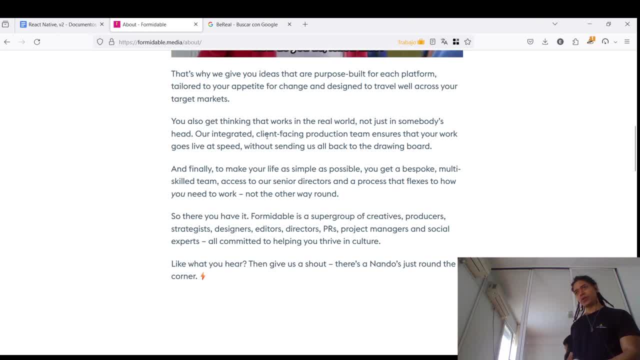 Work not just in somebody's head- or integrated client-facing proteins, ensure that your work goes live at a speed without sending us all back to the drawing board. And finally, to make your life as simple as possible, you get a bespoke multi-skilled 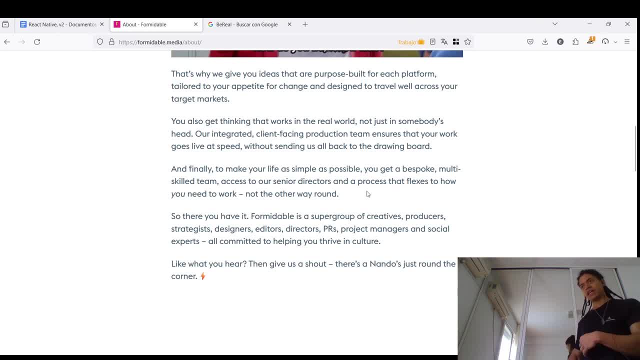 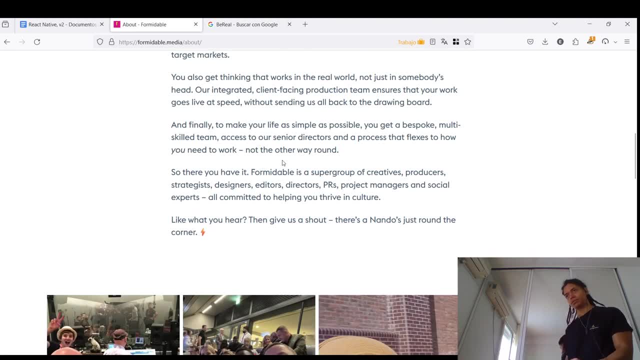 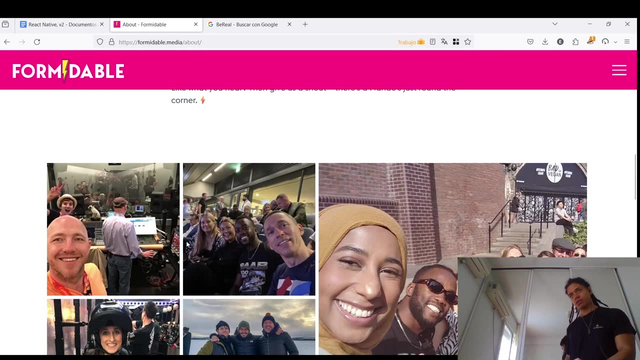 team, access to our senior directors and a process that flexes to how you need to work and not the other way around. So, yeah, there's a very multidisciplinary team here Interesting, Very, very, very, very interesting. 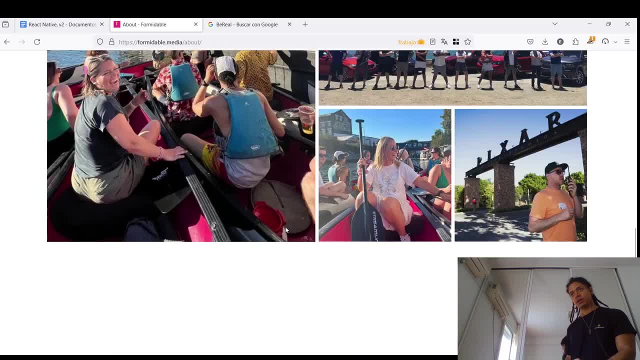 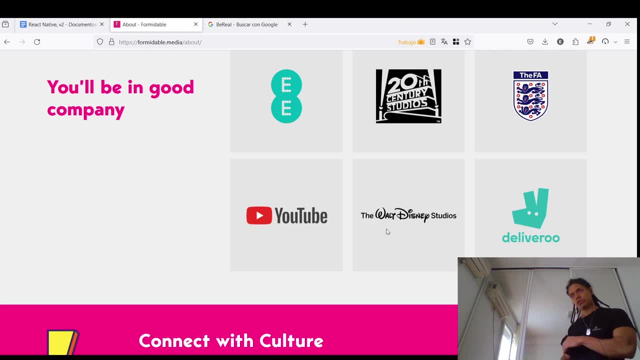 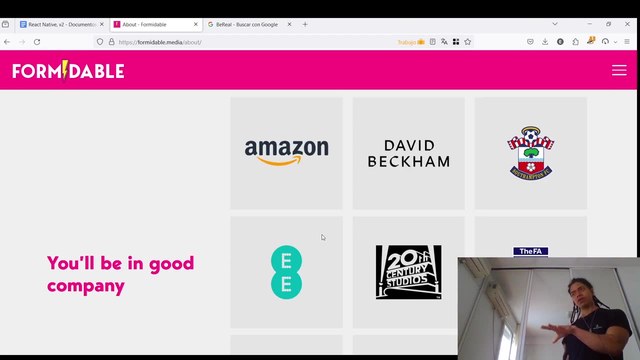 Totally agree with that. So, yeah, they're creating this. You'll be in good company, Amazon, David Beckham. So they manage this. they're um. okay, They're not responsible. What's responsible for managing is their um, their social presence, their image in. 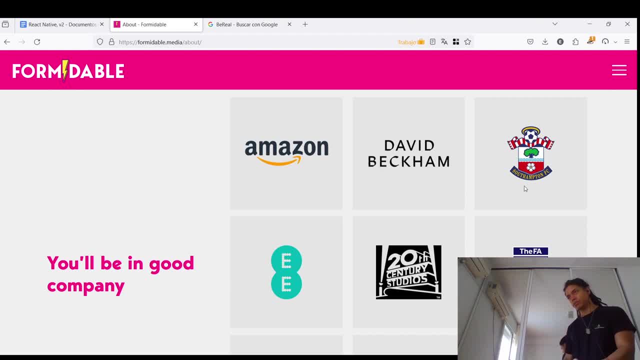 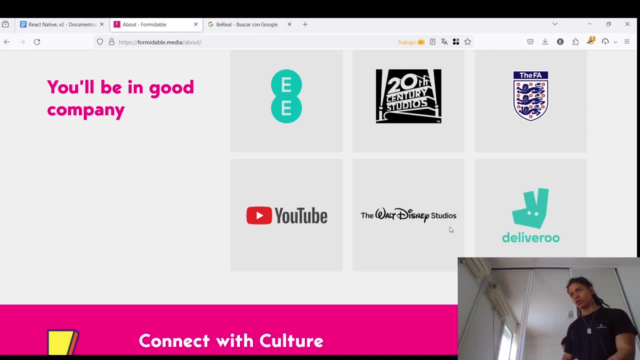 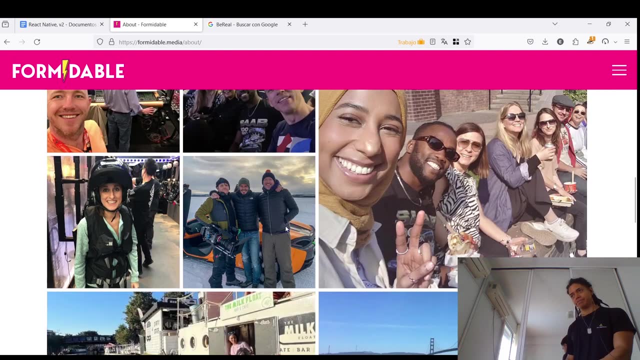 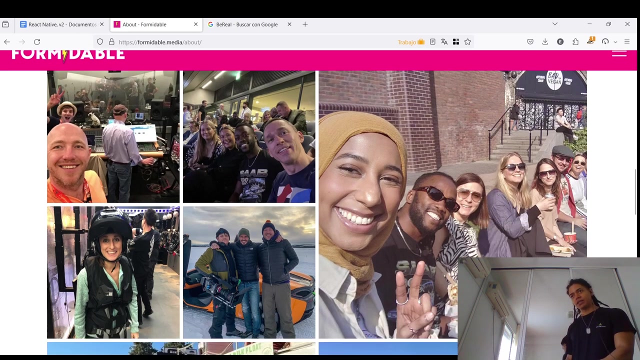 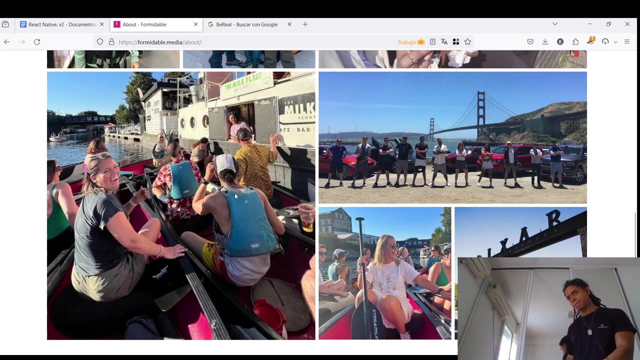 there, David Beckham, Southampton, EE, 21st Century Studio, DFA, YouTube, Walt Disney and Delibro Interesting, So they're quite busy. I must say, Right, They're quite busy. I must say, Uh, so yeah, in things like this, um yep, uh, so yeah, it's San Francisco, so they work. 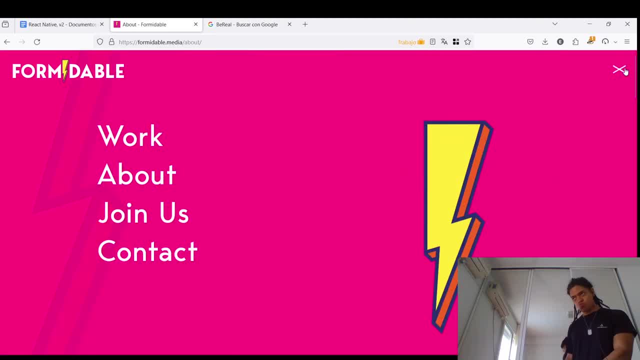 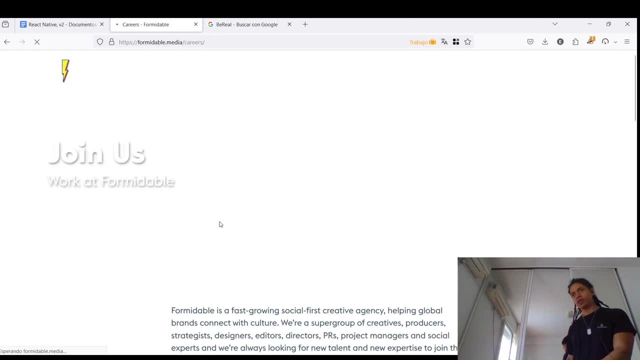 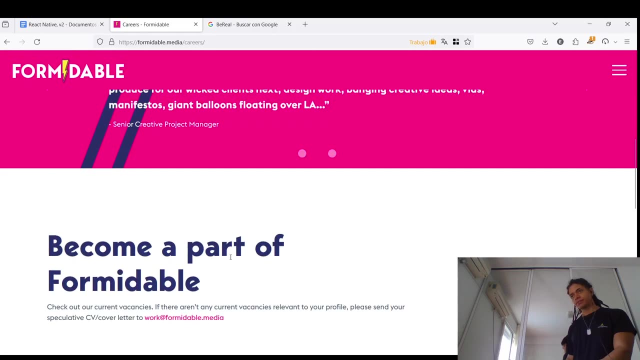 off all this Um so, so about us join us? Uh, she, they don't actually. I don't know if she's actually mentioning which kind of people are working with them. All right, Mm? hmm, Nope, they don't show which kind of people are actually working with them. 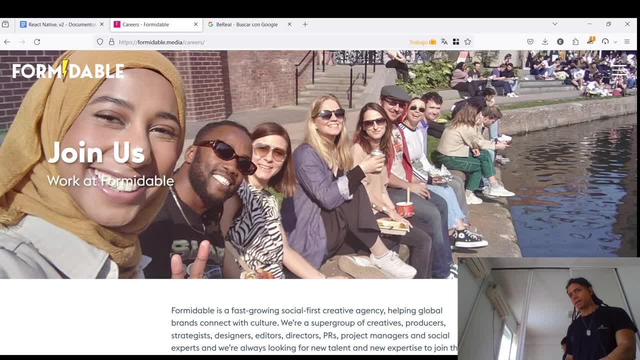 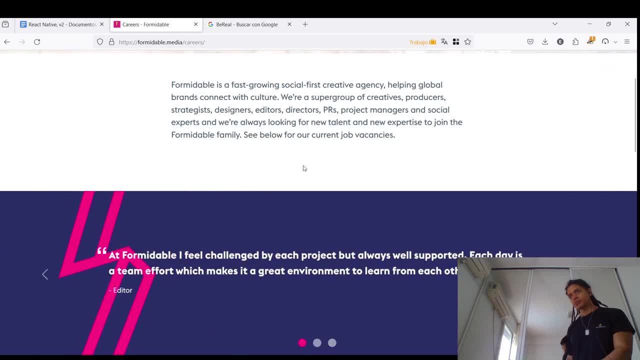 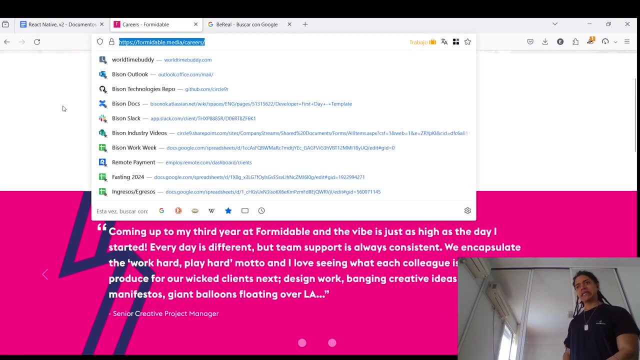 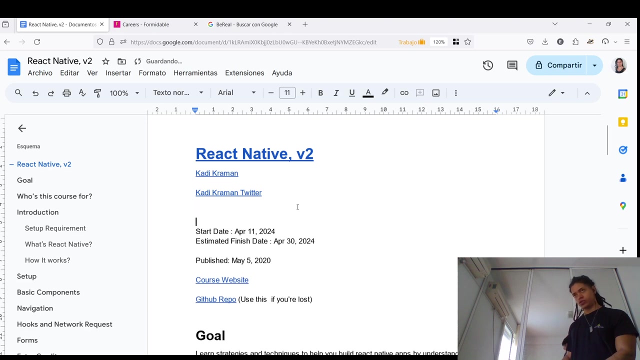 Uh, and I think uh, mm, mm-mm-mm. Formidable is a fast growing social media. uh, first created agency, Lemme, actually, take a look at the description. Uh, yeah, Mmm, now here, add this: okay, so credit, cut, cut. caddy Crammond, work, work at formula. 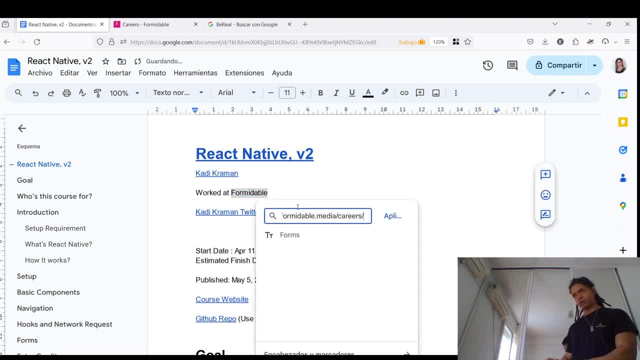 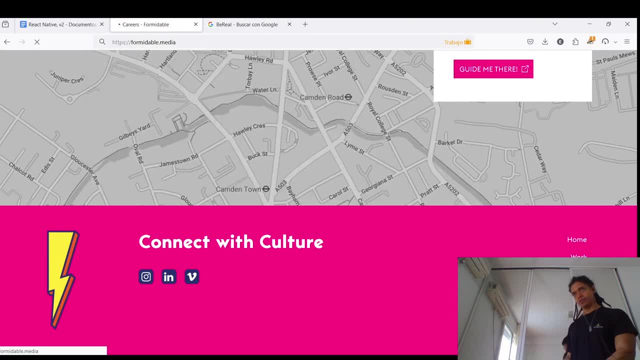 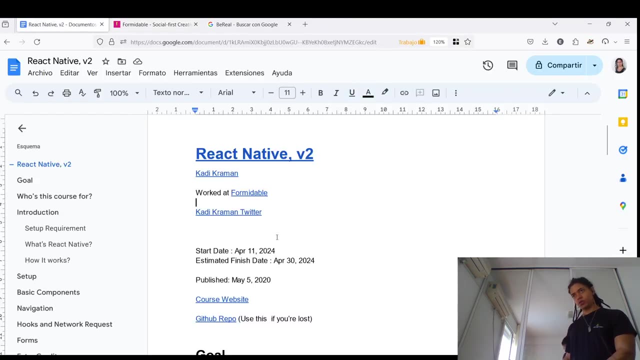 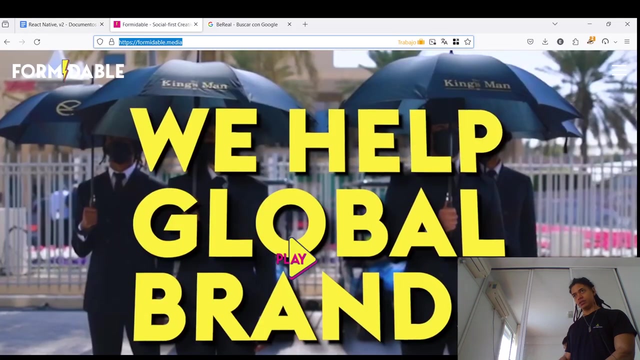 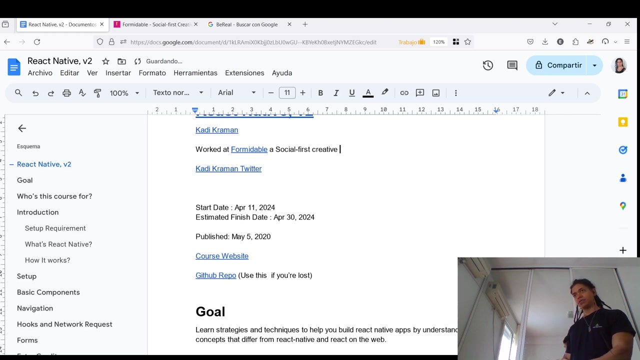 table: formula table: right work at formula table here and I just want to use the main URL. right, that's right. so yeah, so she worked at formula table. okay, like this, so she worked at formula table. a creative agency- a social is so a social first creative agency. so they actually thriving to capture the user's. 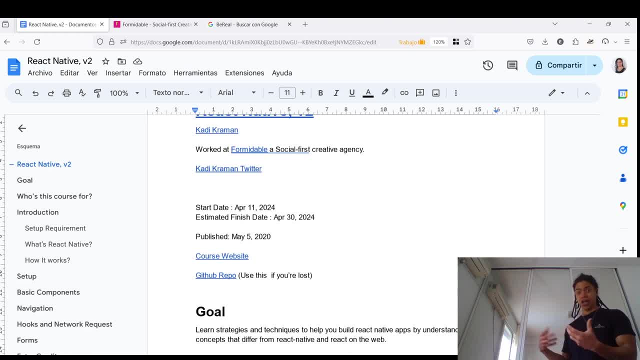 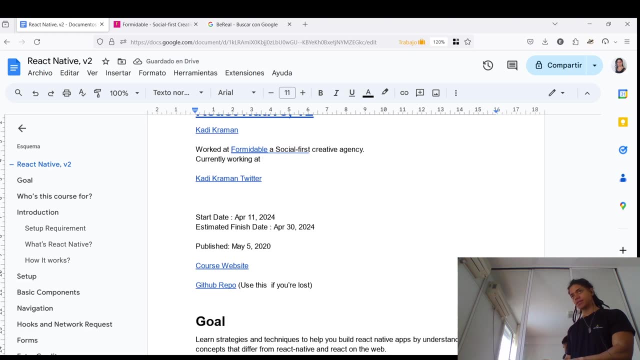 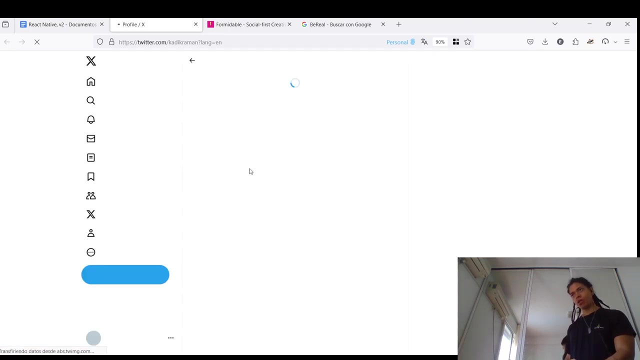 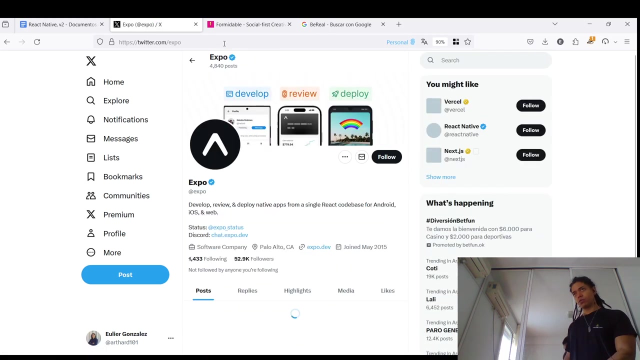 attention as much as possible. and now and now there are a lot of people actually out there competing from that and currently currently working and, and, and, and and but but. so she's currently working at how they put accordingly the expo effectively. currently working at expo. you may wonder what is expo? glad you ask the software company. 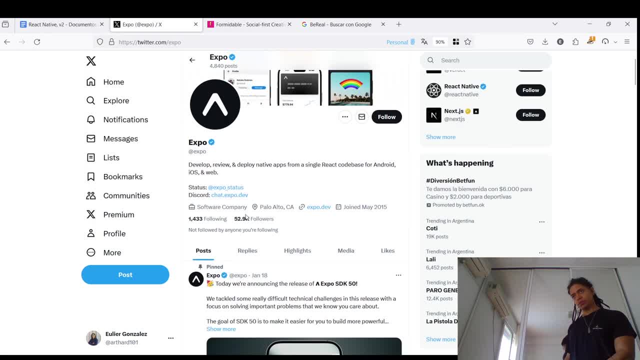 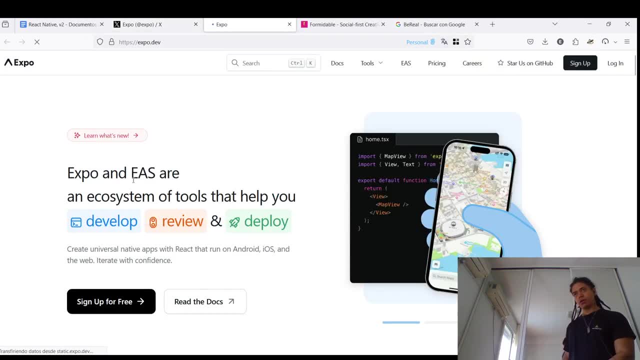 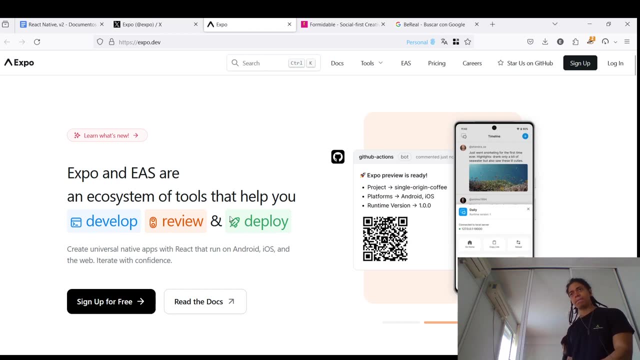 now you got expo and ESA are an ecosystem tool that has a very well aussie default API, but you get set up. once you have set up the 78, to also set up 3M, and now let's that help you develop, review and deploy. 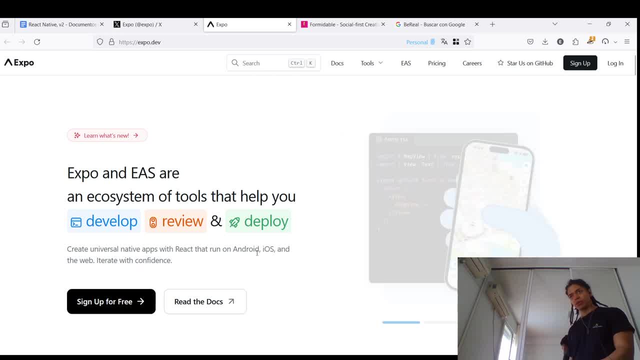 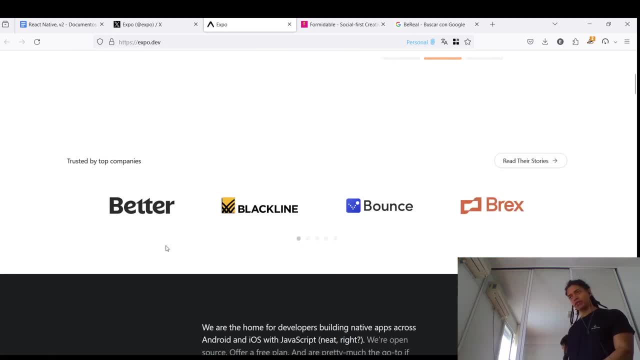 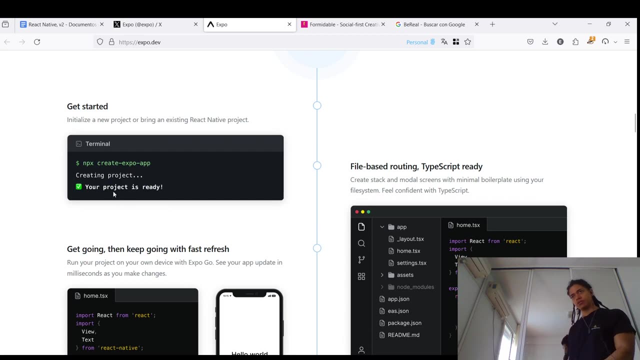 Create a universal native app with React that runs on Android, iOS and web, interacting with confidence. So I'm assuming here that this is the build tool, something that I'm quite new to this, I must admit- And get started. your project is ready. 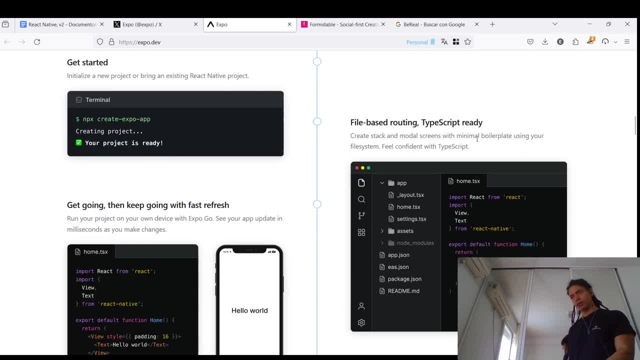 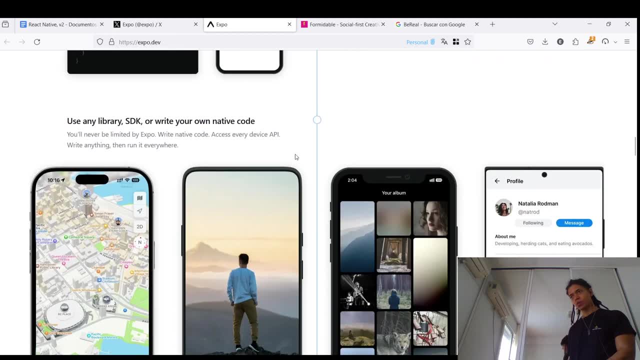 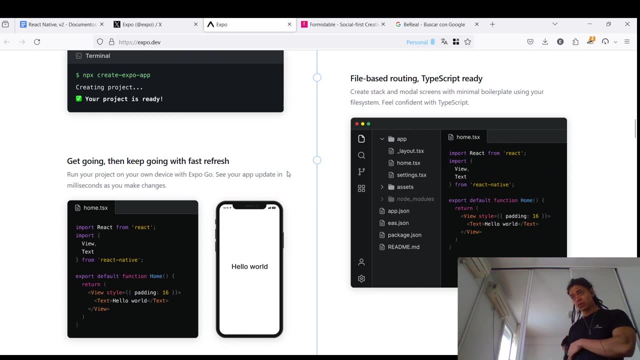 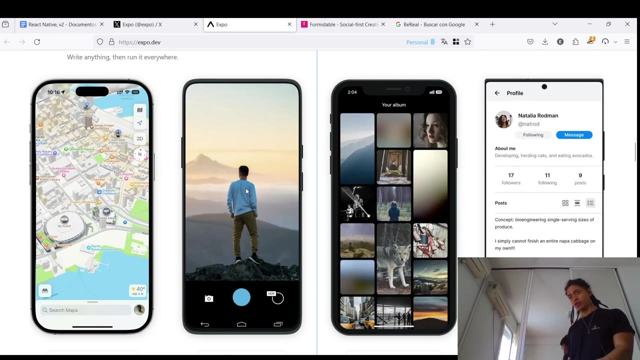 And okay, this is the development file-based routing Going get. then keep going with fast refresh. Okay, can we develop inside of Expo? Okay, because if it is, that'll be great. That'll be great, by the way. 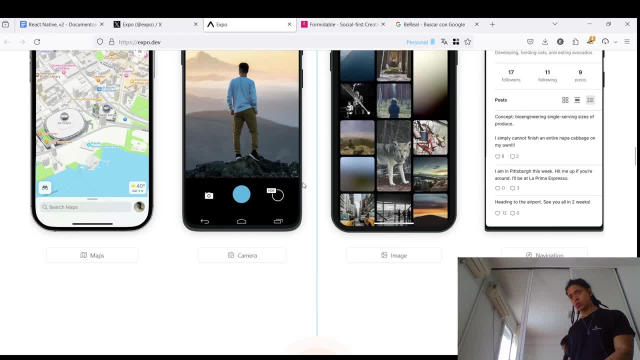 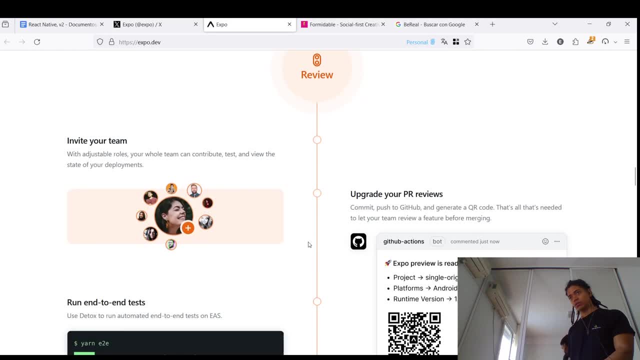 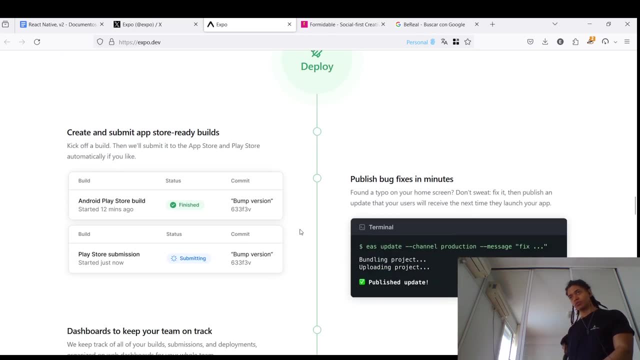 Use any library as you can, or write your own native code Exactly from maps, camera, image and navigation. All right, invite your team, upgrade your peers, run end-to-end tests and, when it comes to deploy Career, submits published book-fixing minutes. 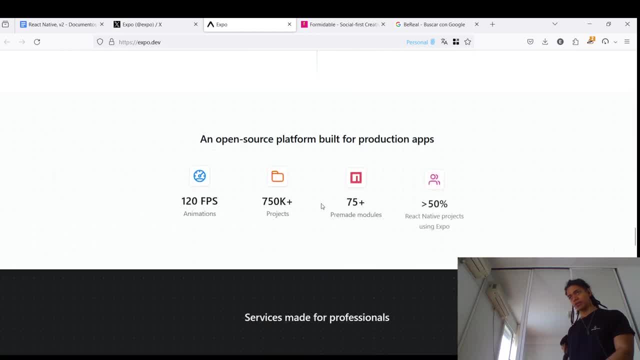 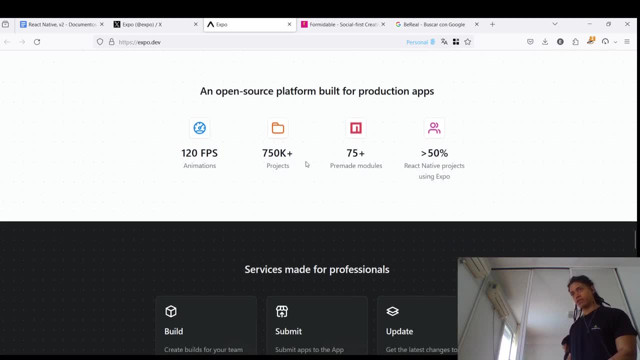 dashboard to keep your team on track E3 with confidence. And open source platform view for productions Here, 100% online. 120 sda animations: over 750k. over 750k uh plot product, uh projects. more than 75 pre-made models. over 50 percent react native project using. 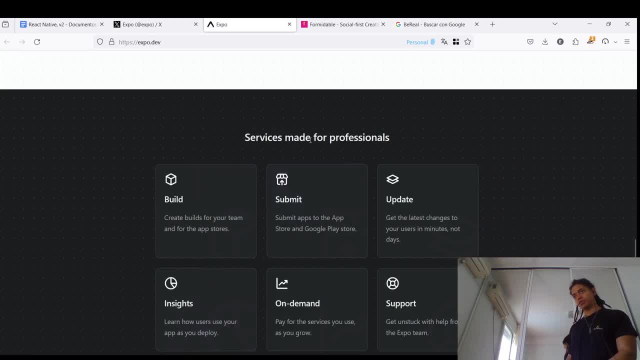 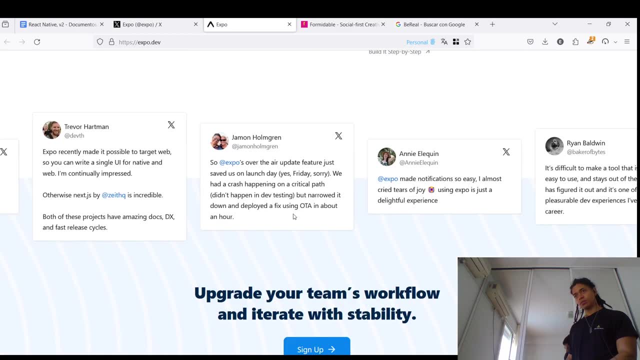 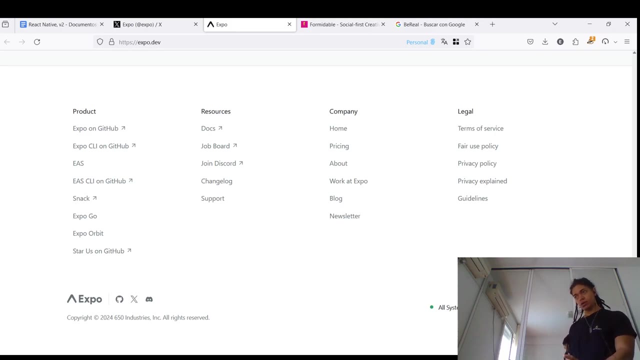 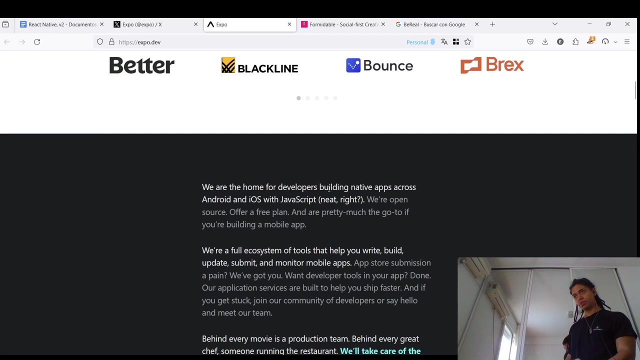 expo okay service made for professional. so, yeah, try it for yourself. little step, uh, but yeah, the idea here is that because she is working now at expo. um, this build tool- we are the home for developers building native apps across android and ios with java- neither right. we're open source, offer a free plan and pretty much they go off if you're building. 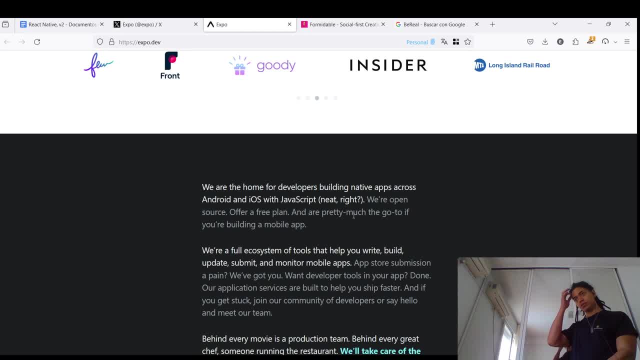 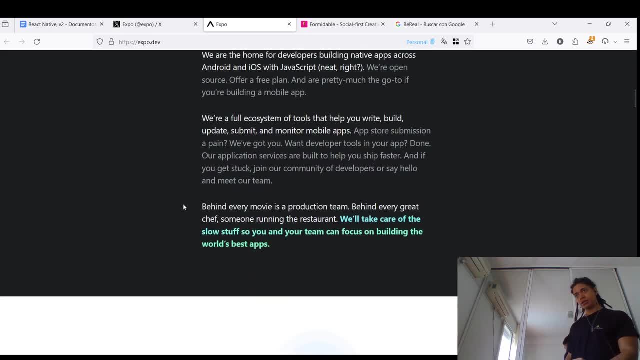 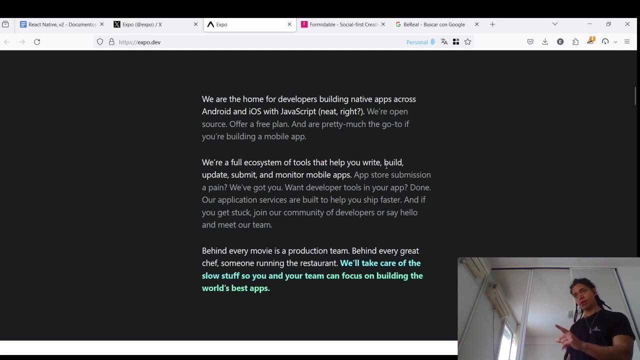 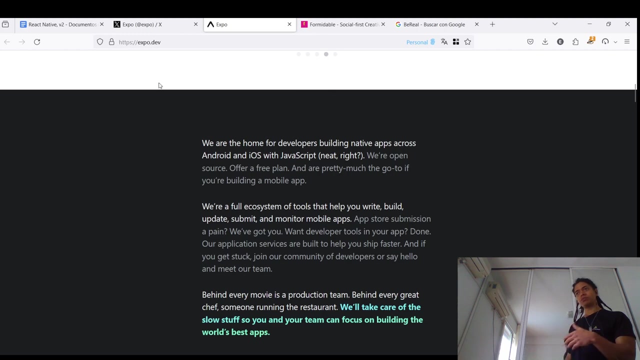 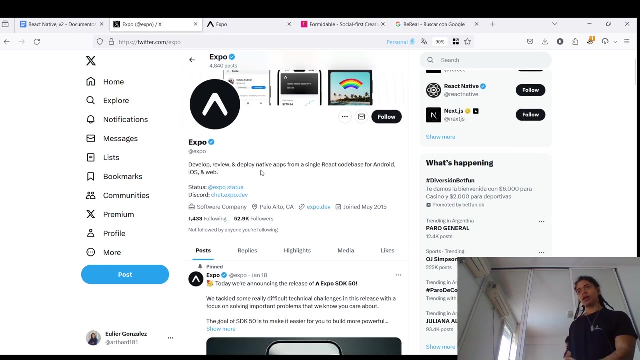 a mobile app. so we're full ecosystem of tool that help you write, build, update, submit and monitor mobile apps. exactly so we're a full ecosystem, that of tool that help you to write, build, updates, submit and monitor mobile apps. interesting, so all right. okay, so now she's working at expo and that makes a lot of sense, yep. 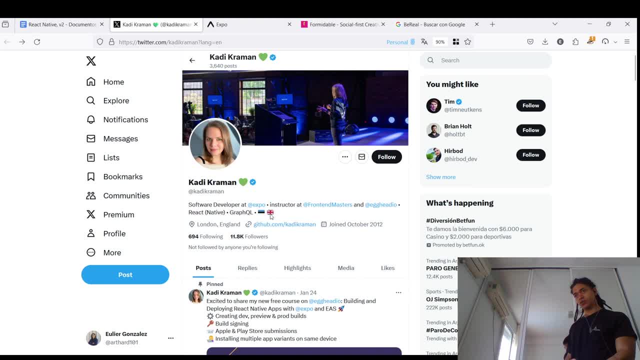 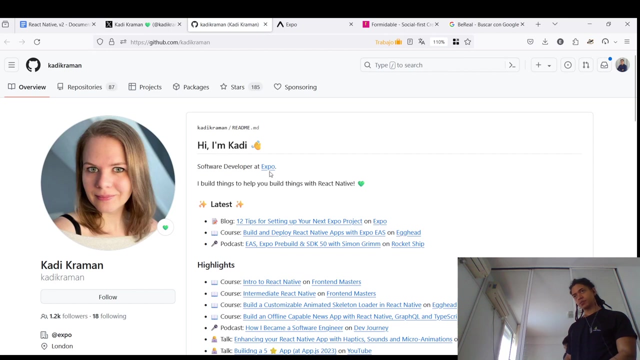 that makes a lot of sense that she's working at expo and now is living in london, england. caddy kraman- okay, she comes from slovakia, and stonia- my bad, my bad, stonia. uh. so yeah, i built things to help you build in with react. 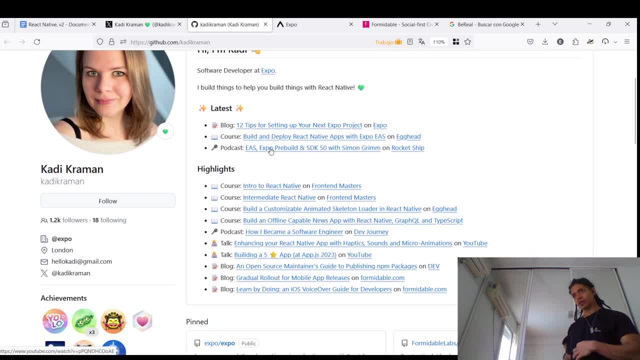 you know, uh. so yeah, blog course podcast, oh, and also in egghead, like so, CSS expo preview in SDK 50 with simon grim. that's interesting and there's a lot of things to do. thank you, i'll stop there. thank you, guys, and have a great day. bye. 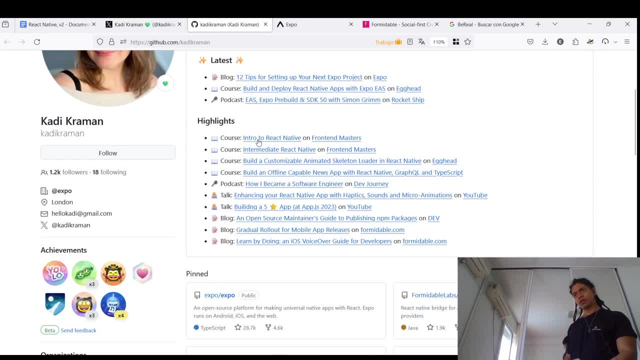 also very, very important, completely, of course: enter to react native intermediate to react native build and customize animated skeleton loading react native and heck, build an offline kebab capable. new news app with react native rafael and typescript. okay, how i became a software developer- a death journey. okay, talk, enhancing your react native building, five star. 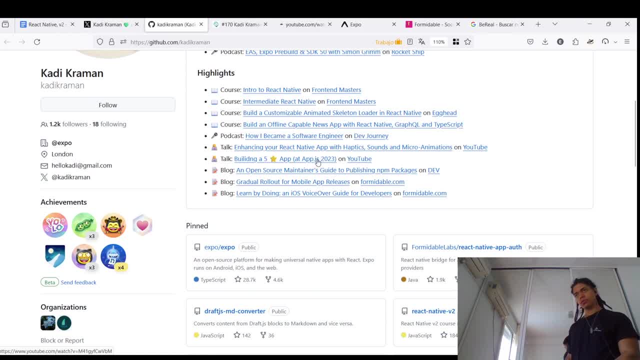 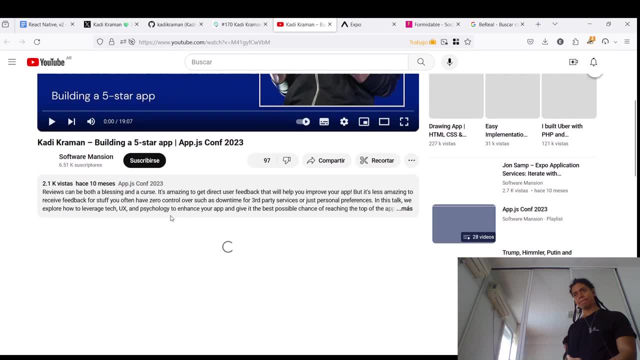 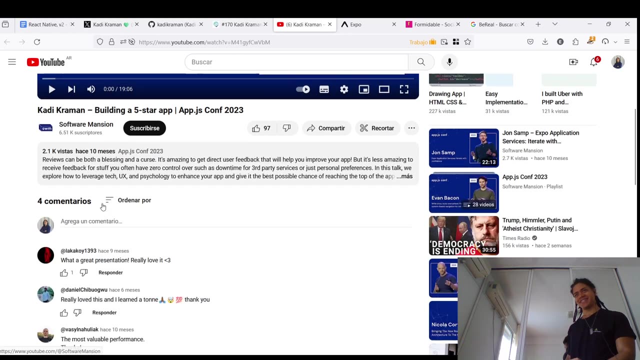 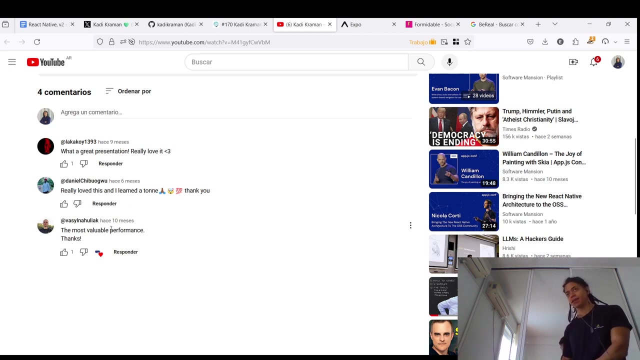 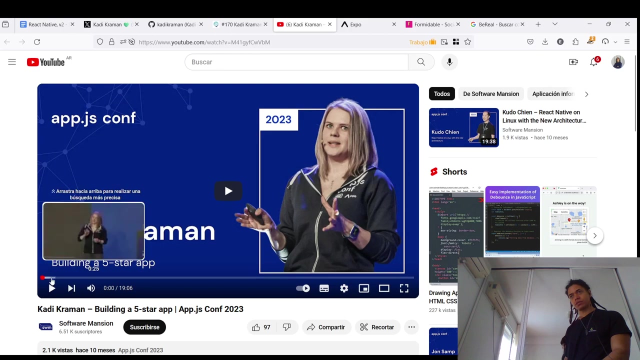 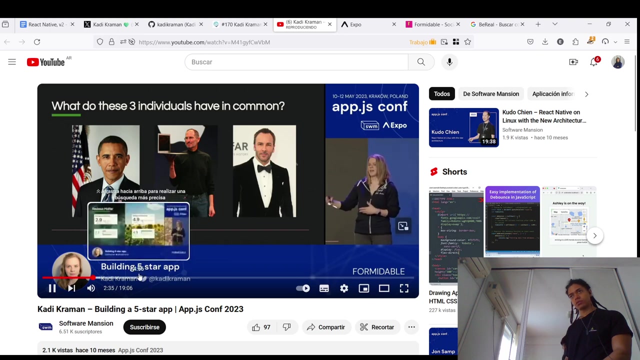 apps on youtube, okay, but that that's basically what we are going to do, right? yeah, but interesting, software mansion. you know what they talk about. you know what they say about software machines. the most valuable performance here- okay, so that's interesting. so they do this- is to take the choice of what to wear. 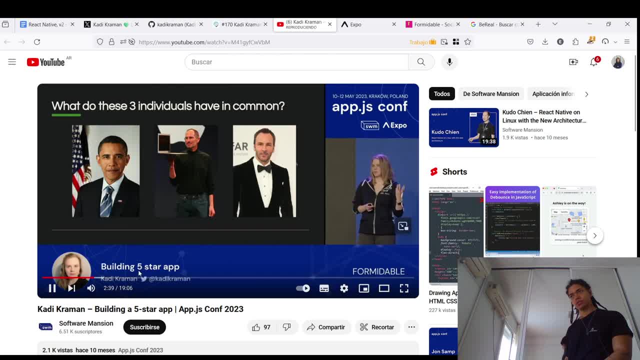 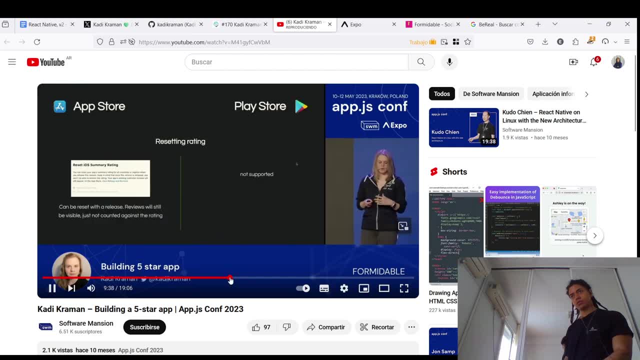 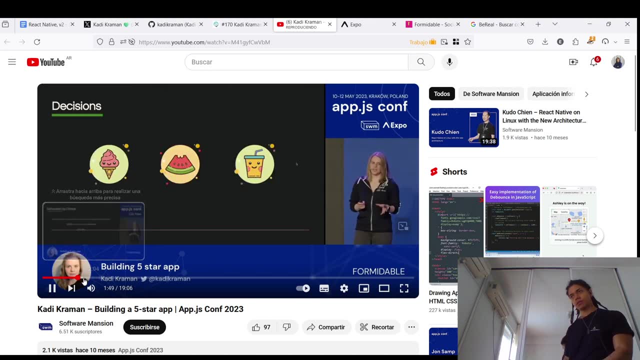 out of their day so their decision-making fuel could be used on more important decisions, such as so orang was introduced and have a treat day on friday. so on friday, spoiled for choice, but really we are exhausted by all these choices. there's been a lot of studies on this and a very 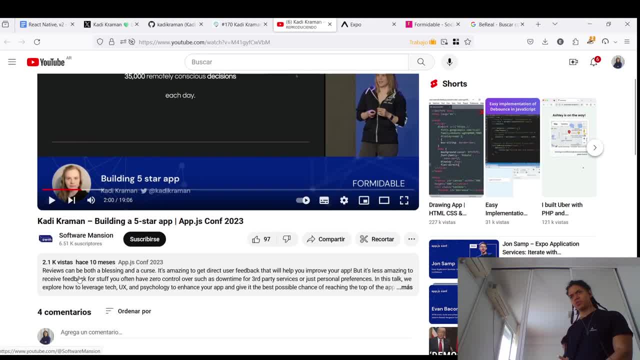 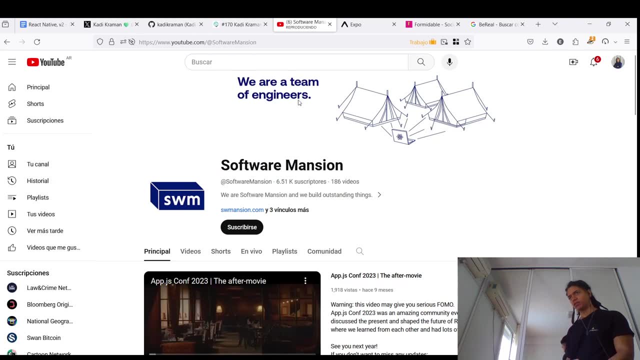 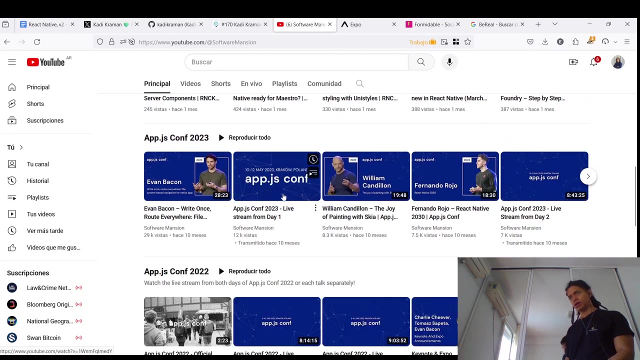 his researches have found that actually, this is something interesting, because this was like 10 months ago, oh my god, software mansion. okay, interesting, we are team of engineering. okay, we are a team of engineers, team of engineers where they're now recording this kind of video. okay, that makes a lot of it. 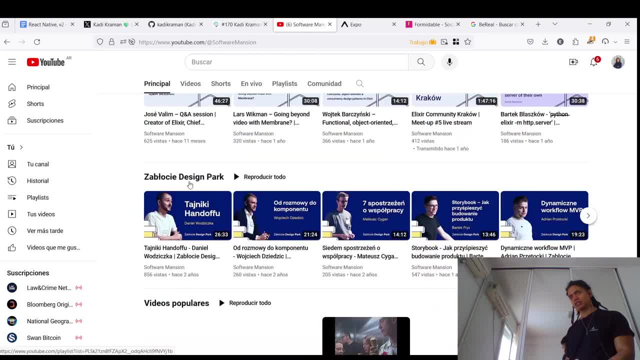 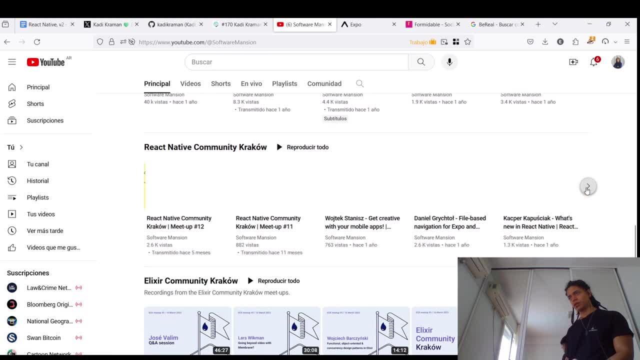 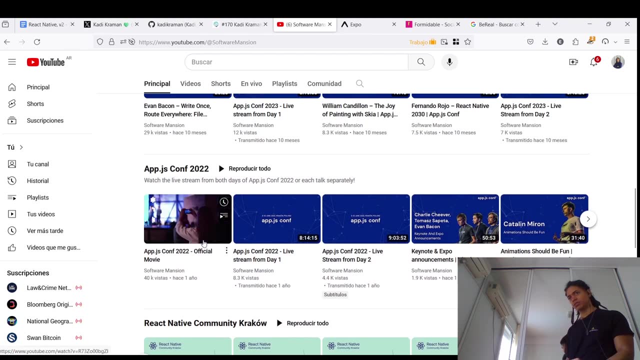 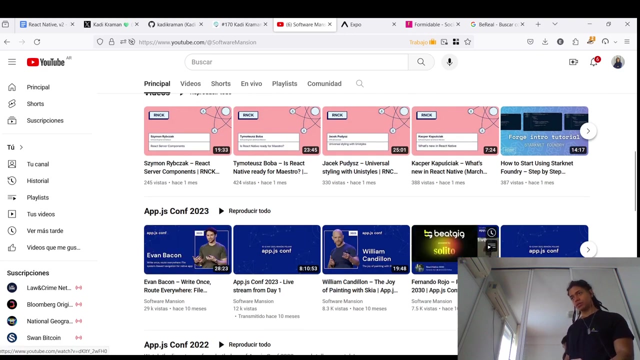 okay, okay, in the skills of that elixir, uh, interesting elixir. react native community with that interesting in, very, very interesting at the yes concert conference 2022 and 2023. okay, that's, that's very, very, very, very, very important. oh my god, okay, okay, react. native fernando rojo. 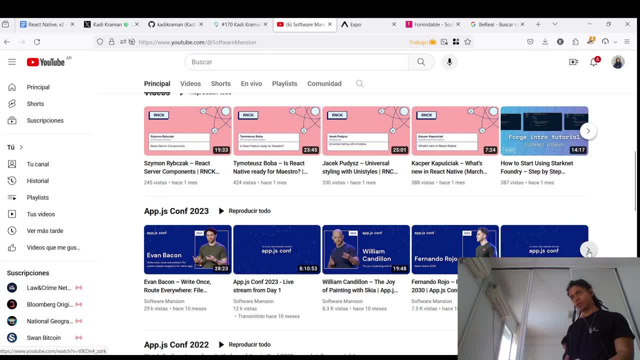 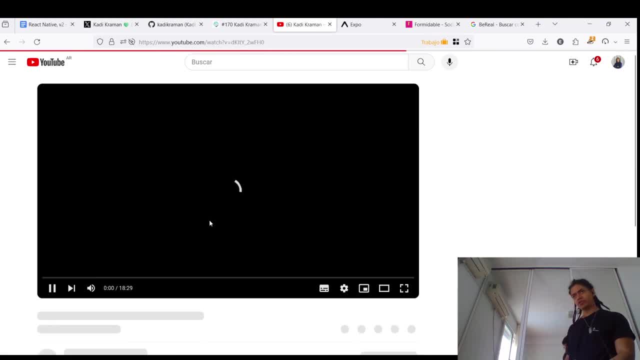 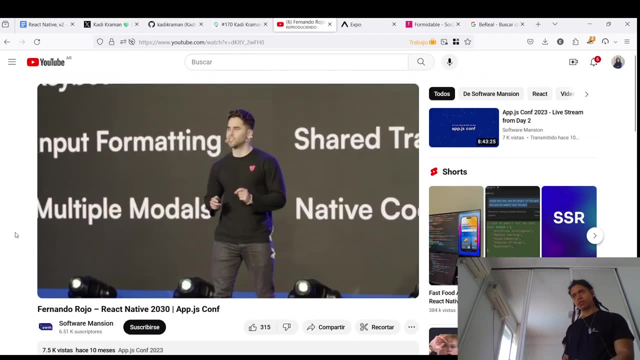 but, yes, the joy of painting with skia, that. that last name is quite interesting to me. it's like where are we now and where are we going? okay, did you know that? i had a lot of fun with that? so great into the future. so that's what i wanted to ask you to do. 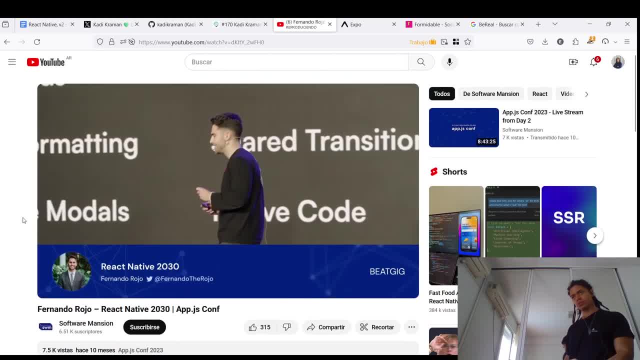 yeah, exactly, it's like. it's like: well, i don't know if you've been um, it's not like i'm gonna be able to do it, but do you know how to do it? i mean, like i am really glad i've been able to do it. 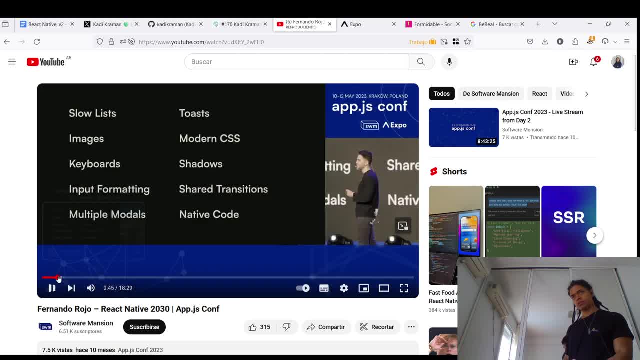 this is my favorite part about it. i'm like i get to live here. it's like i wasn't really able to do it. it's like i don't know if i would have made it if i wasn't able to do it. i mean, i think that's what it is. 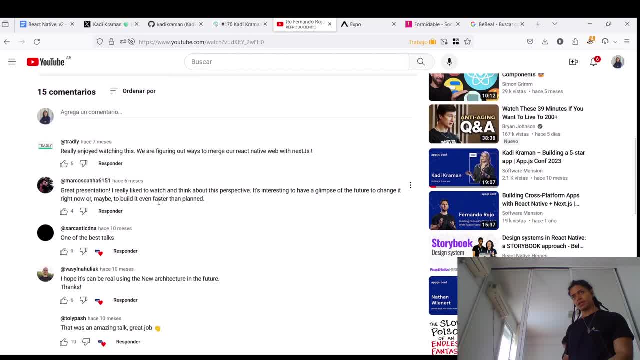 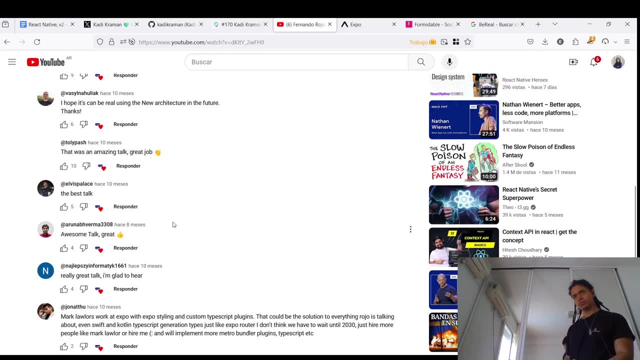 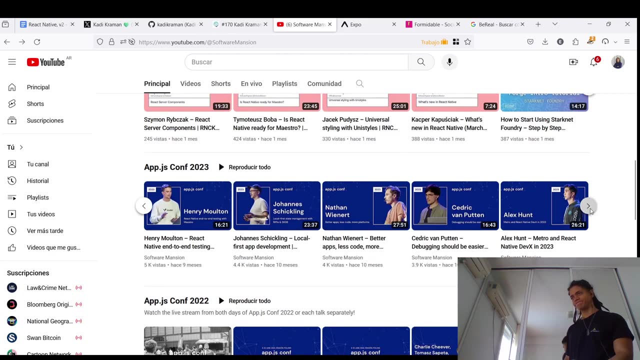 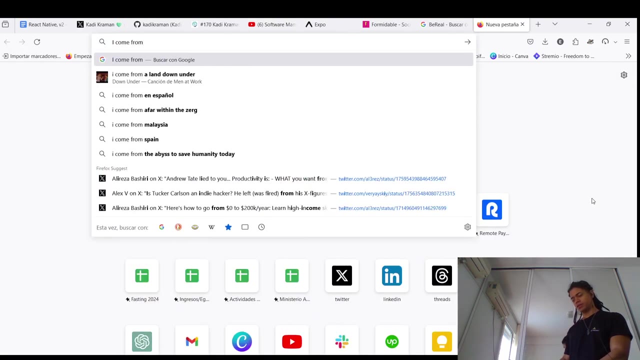 it's a very interesting to me. it's like i've been able to do it. it's a really great experience. um, i mean, i'm really glad to be able to do it. but, yeah, okay, mm-hmm, okay, oh, that's, this is mm-hmm, mm-hmm. I come, I come from copper, then I 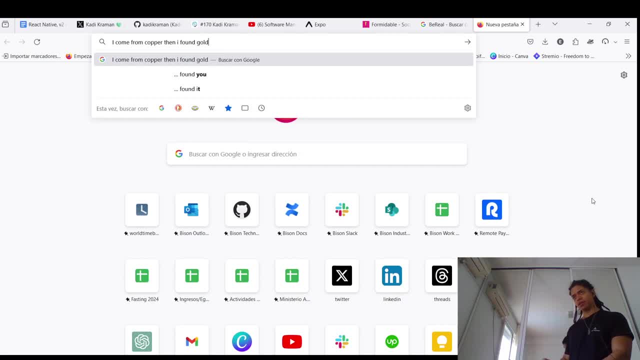 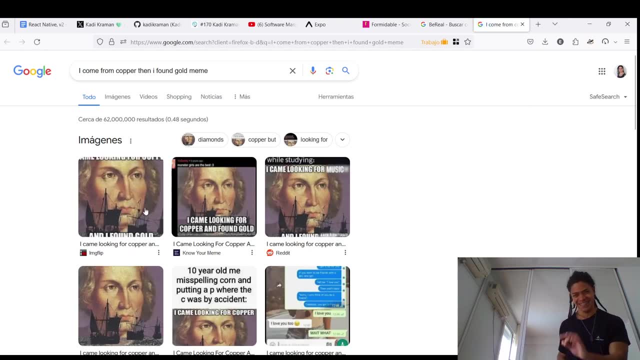 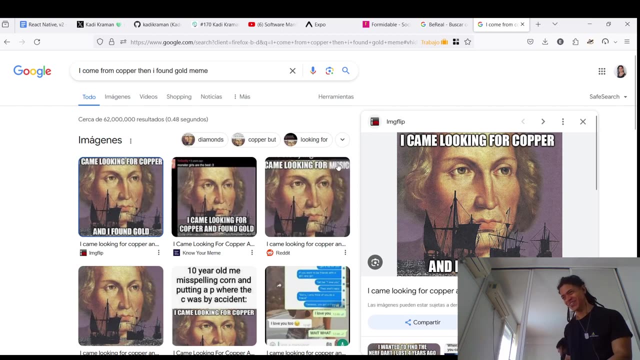 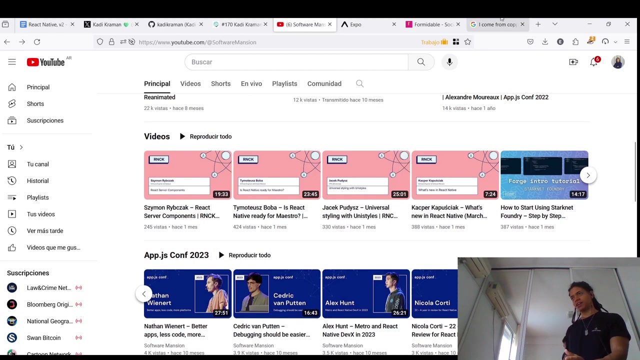 find, you know, found gold mean I think I don't know if the US use that me. yeah, exactly exactly I came looking for copper and I find gold. oh my ah means rough, means, yeah, it encapsulating a lot of polemic stuff behind the thing, behind the scenes. but yeah, yeah, okay. so exactly I came looking for copper, Jesus. 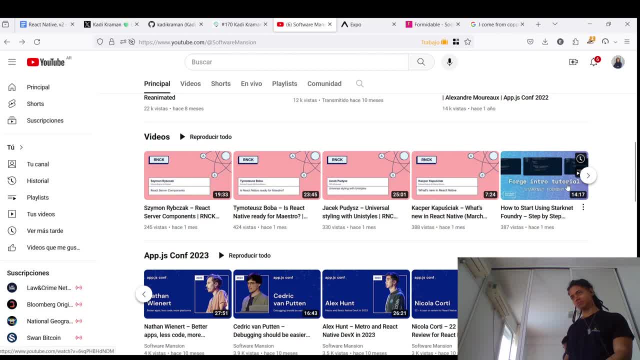 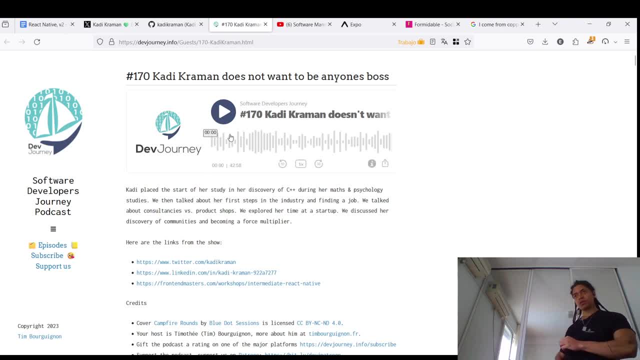 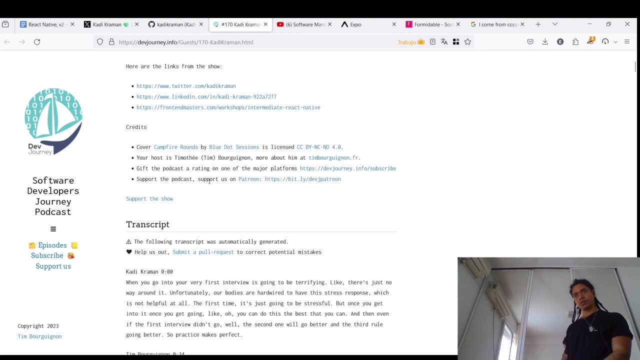 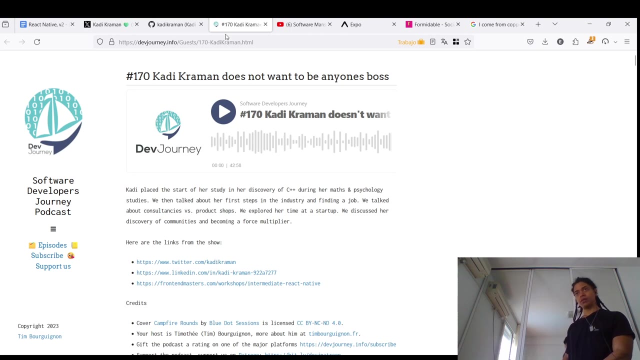 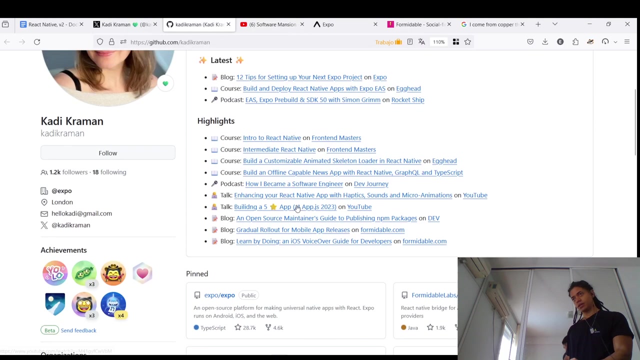 I came looking for copper and I find, oh my god, okay. so software mention exactly software mention okay, in part of their pot hair. yeah, this is her podcast, but it's like learn by doing an e-voice voice. a guy on that formidable account is interesting, is also in their blog for that, but that's the whole point. 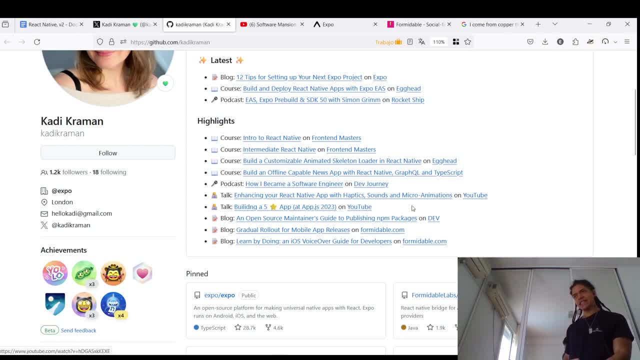 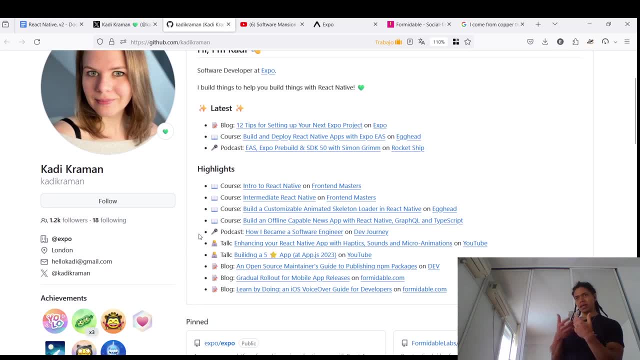 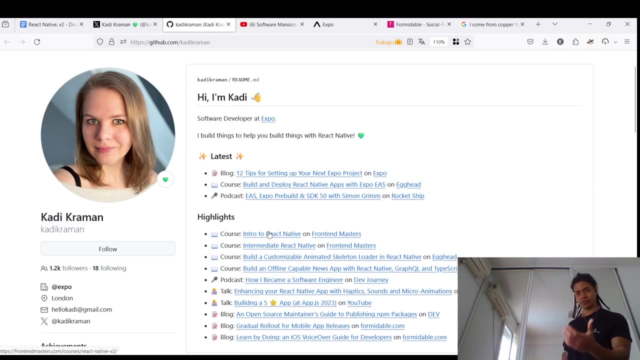 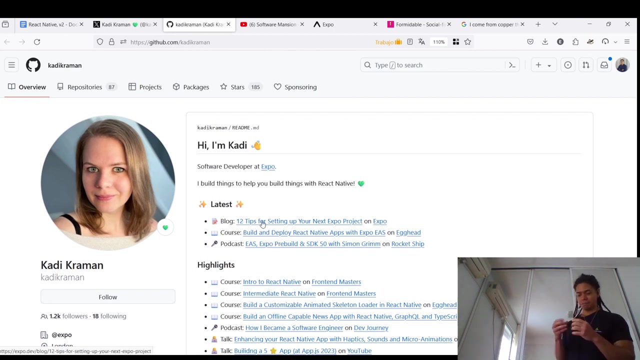 of this you know is that she's not in London. is that? look at this, this look at the way of how you are actually building your own life, because that's what you're doing here when you look at caddy, or so, when you look at caddy, or Scott Moss, Brian Hall, 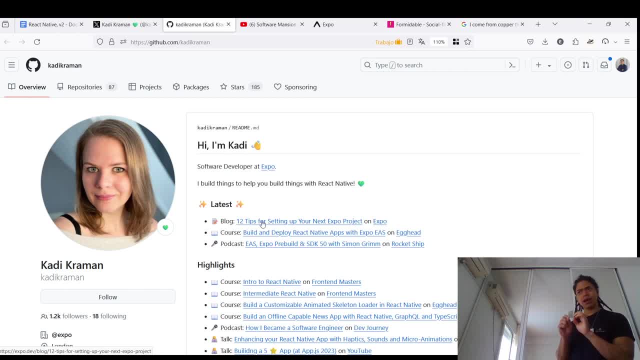 will sentence, just will sentence. just to mention a few names okay in how they join they. they to mention a few names okay in how they join they. they keep their shit together, sort of speaking, as a way to say: this is how we are getting to this industry and 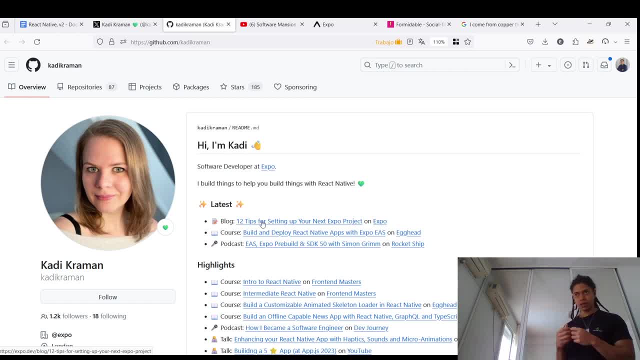 we come from different backgrounds and then we align ourselves to what the markets mean, whether it is on know the yes or react native, or in the case of caddy, or in the case of no, like Scott Moss, okay- by building knowledge of applications and this API design node, or 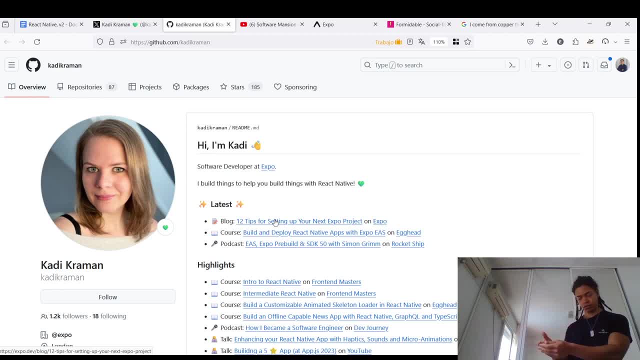 in the case of react from Brian Holt, from react or react production, great application inside the few elements we'll Olá for will sentence when and Aaron will sentence when comes to talk about is just be the her parts. so the idea here is: you a, you can see. this particular pattern is: look at what they. will sentence when it comes to talk about is job screw the hard part. so the idea here is you- and you can see this particular pattern- is: look at what they have done, see what you can do with your live as you build this in college, the software industry and share a lot. 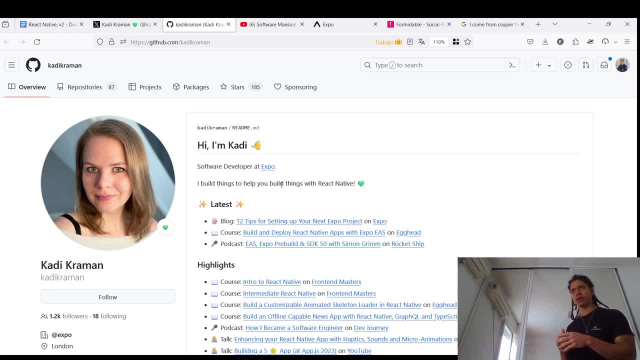 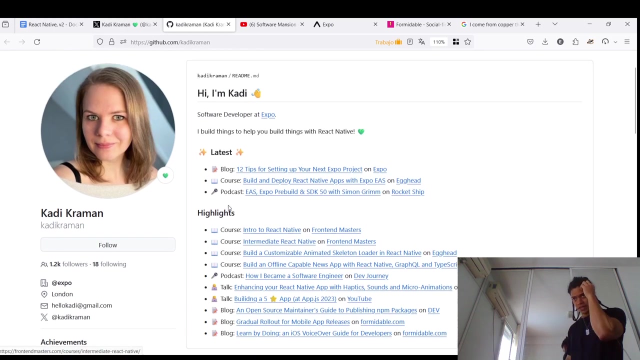 there and the software industry and share our that, share how you reach to this, while you actually learning more about how you live your life, how you are a professional, and the new challenge that is ahead of us in the 21 Center with the AI. so okay, so now things caddy, I'm also. 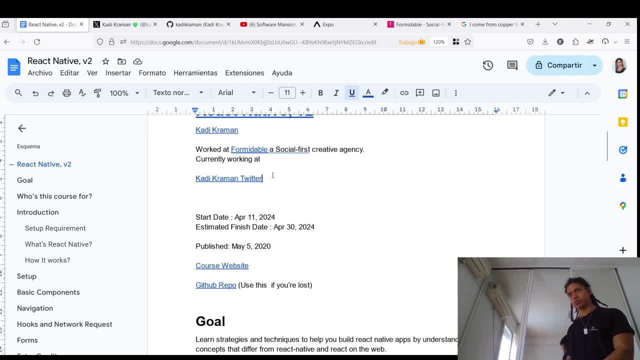 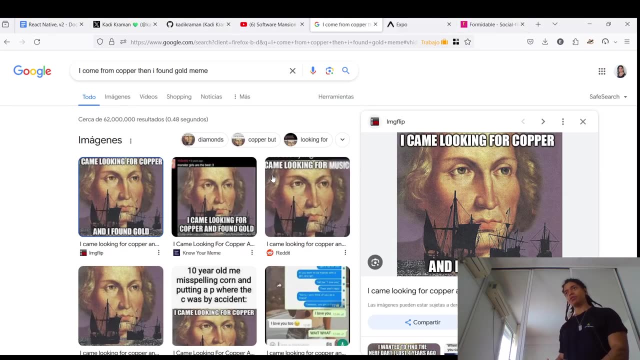 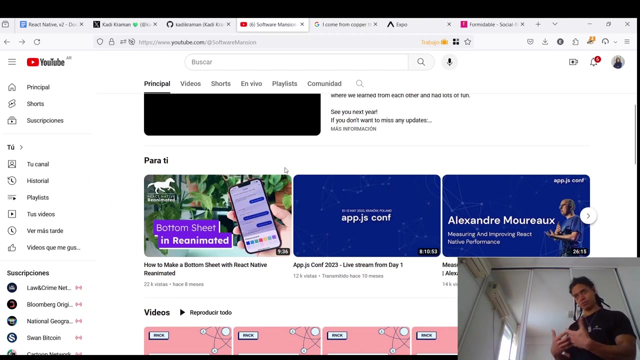 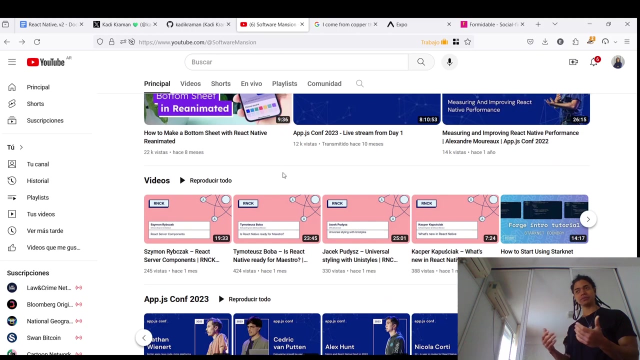 going to keep up there. you can, not only the Twitter, but also Caddy Crammon, github, okay, and I look. this is completely. I came looking. I came looking for copper, I found and I found Goldman- oh my god, in a Spanish, because I come from Spanish background- is pretty much like that. I came looking for. 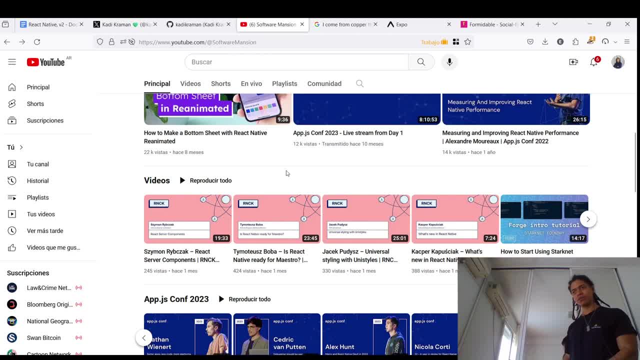 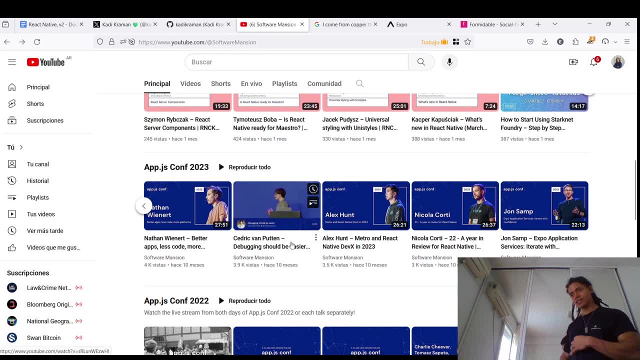 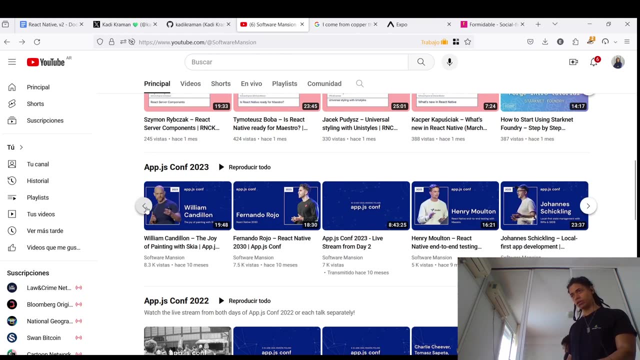 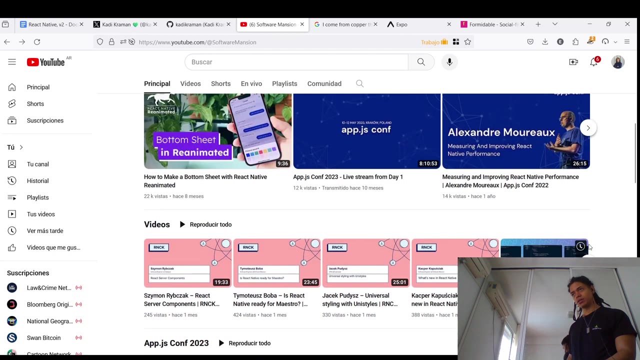 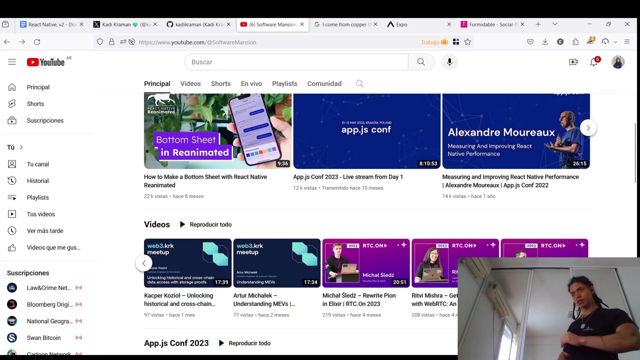 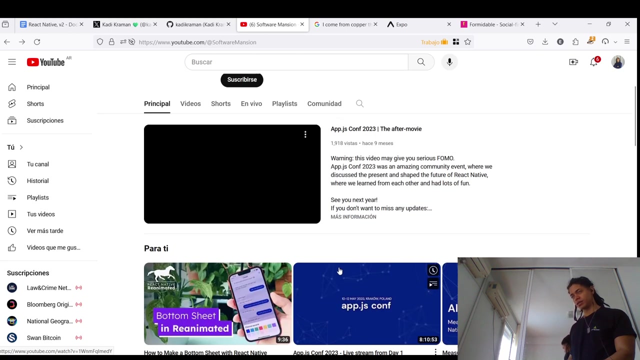 copper and I found gold, okay. so that's quite interesting. I didn't expect to find this, not at all, not at all, not at all. completely I didn't expect to find. I definitely didn't expect to find this. yeah, I definitely didn't expect to find. okay, holy. 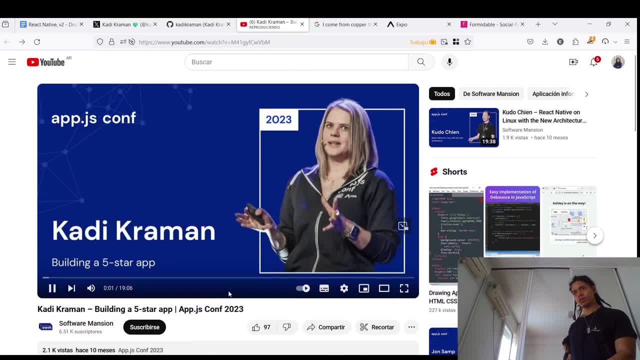 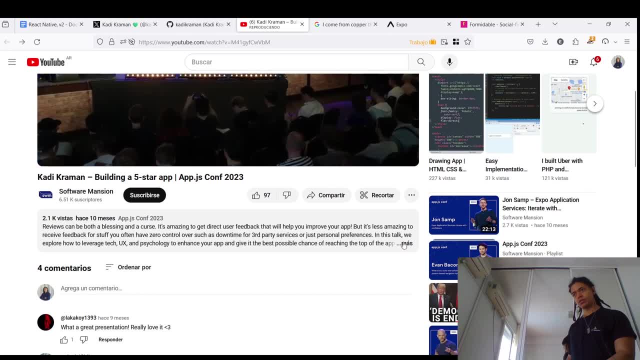 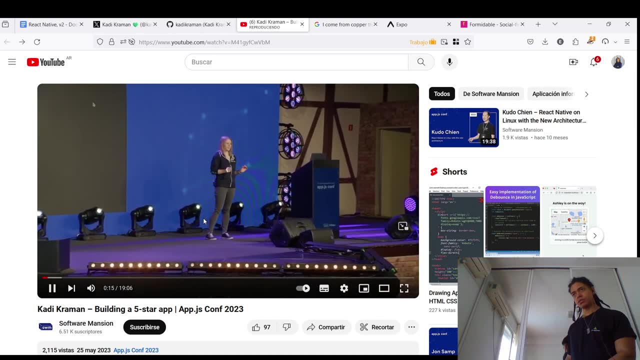 yeah, hey, thank you. I am so excited to finally be here at FGS this year, so we excited to give you the talk that I was meant to give last year. thankfully, my topic is timeless. I'll be talking about building a five-star app. in particular, I'm going to talk about why app reviews are. 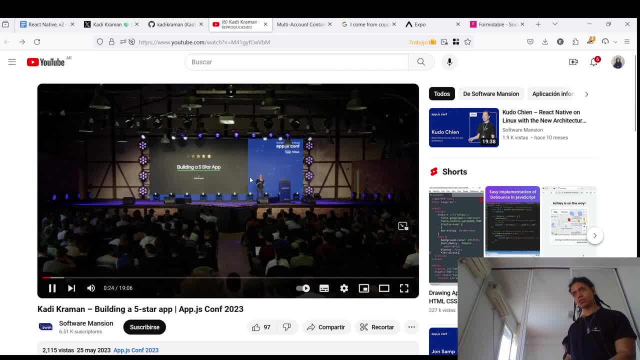 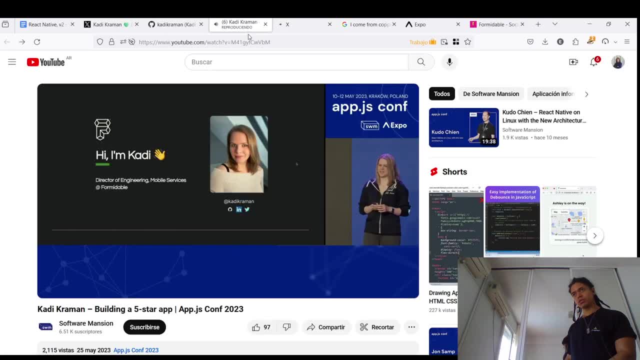 important and what us as engineers, what we can do to nudge our app reviews in the right direction. so just a quick intro: hi, my name is Cady Perman. as Yanni said, I'm currently the director of engineering for mobile services at exactly. she's not the director of engineering mobile service. 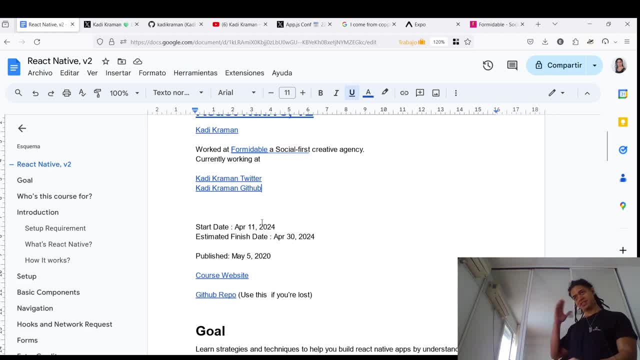 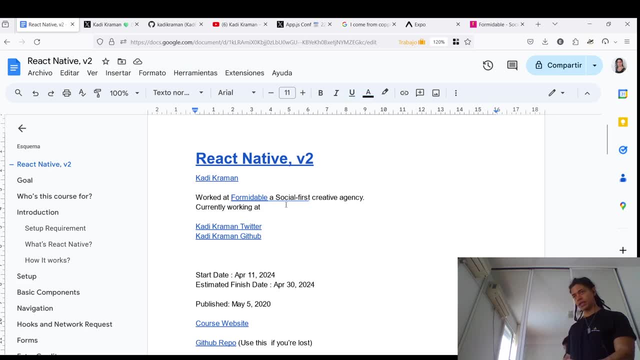 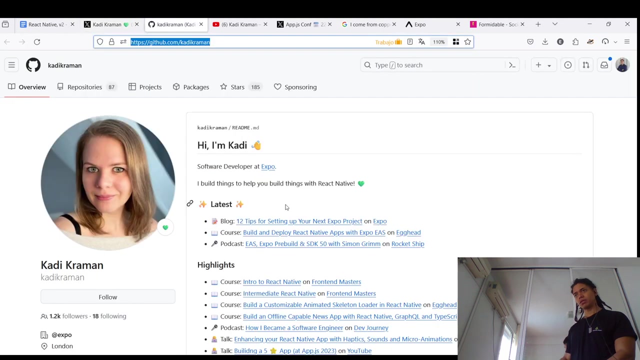 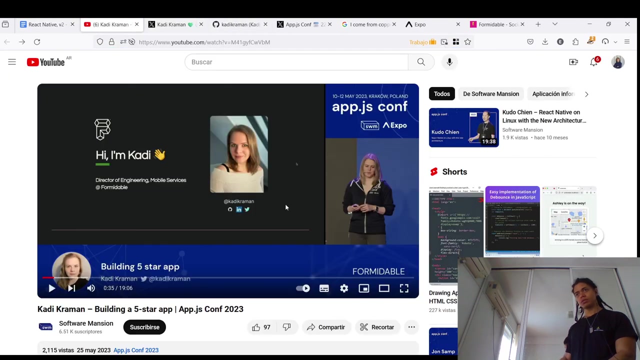 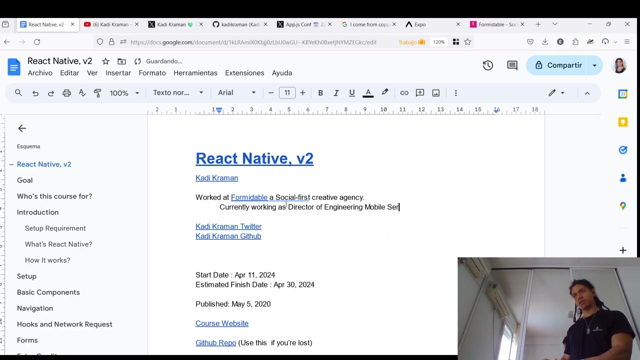 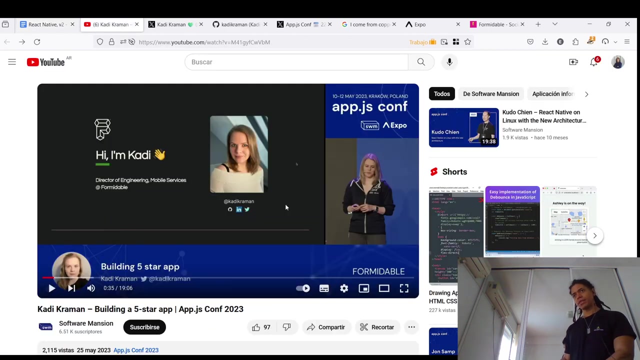 director of engineering: holy moly. okay uh, work at formidable and social first creative agency, including working as director in in engineering. okay, director engineering, yeah, director engineering, uh, director. director of engineering. director of engineering- mobile services. I think this is a very good niche. by the way, at formidable, you can find me on the Twitter if you want to connect um under Cady Perman, that's. 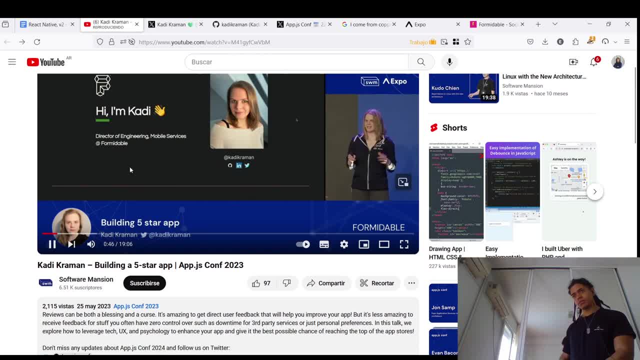 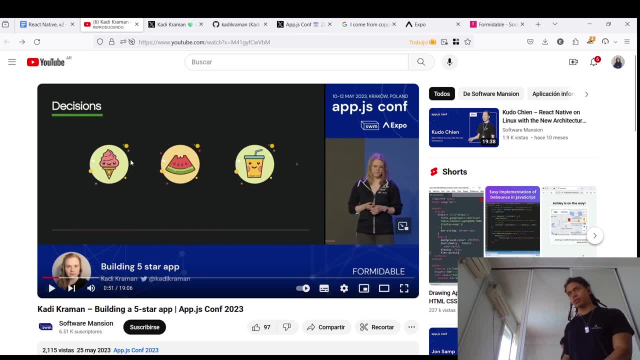 usually my handle. so I built a bunch of mobile applications and I'm excited to share some experiences. but this is interesting, uh, back then, so when me and my sister were little, our parents had this rule that we don't get any treats throughout the week. we have a treat day on. 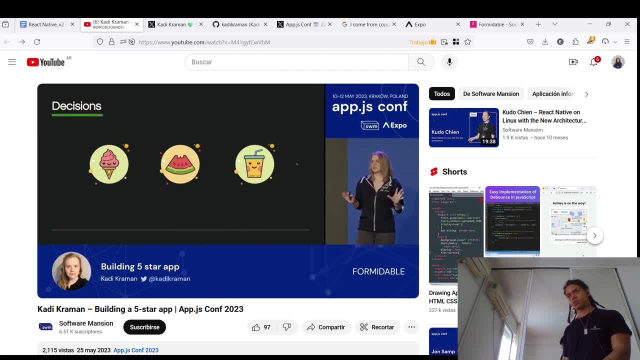 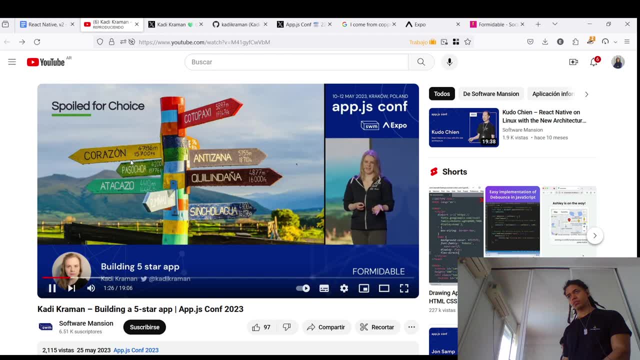 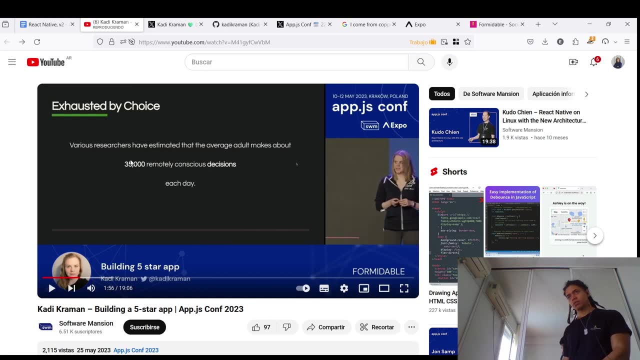 Friday. so on Friday we can tell our dad anything we want from the shop: any ice cream, any chocolate. it was a very difficult decision, making decisions each day and every single decision, and YouTube channel spoiled this. there's been a lot of studies, so I'm a antique which you might have heard of, and it's the idea that the more decisions you 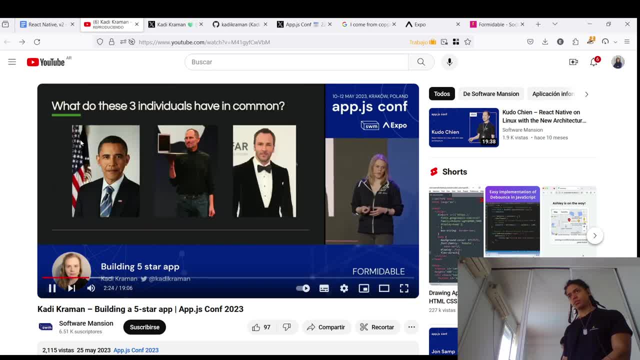 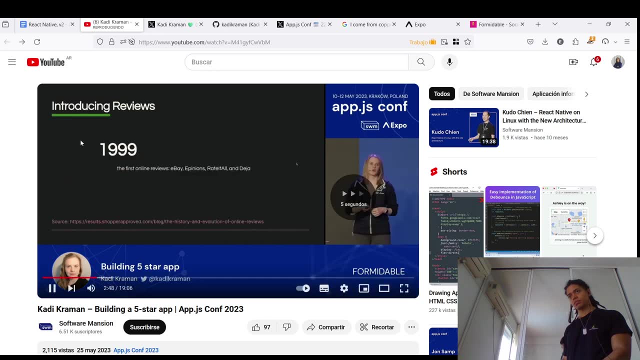 make the worse you are at making those decisions. I don't was. a bunch of well-known people who have a lot of responsibilities, wear the same outfit every single day, and the reason they do this is to take the choice of what to wear out of the day. so, when the reviews are something that we, as humans, 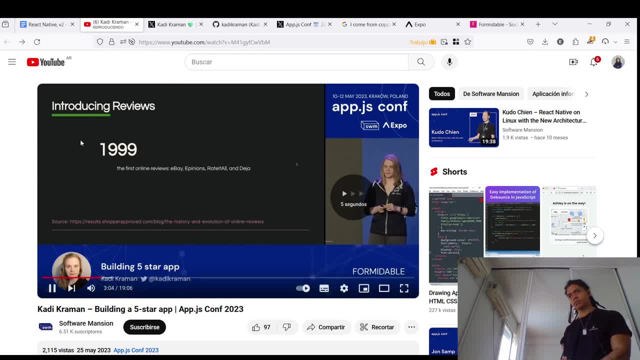 have created to help us make these decisions. the internet became mainstream, okay, so now she's explaining a little bit of the background, okay. okay, it's explaining a little bit of the background, and okay. but remember earlier, and whoever is looking at this video, the goal of this is. 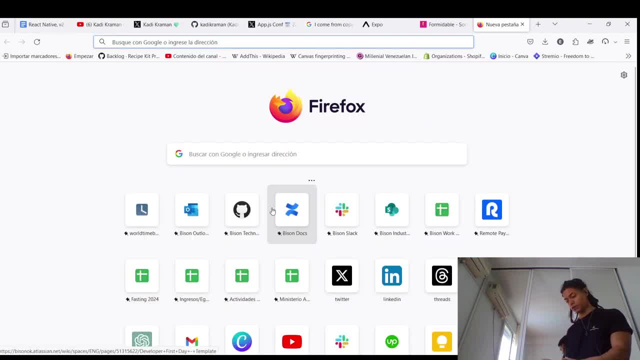 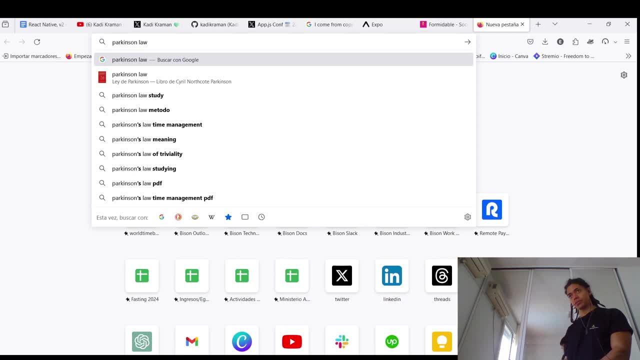 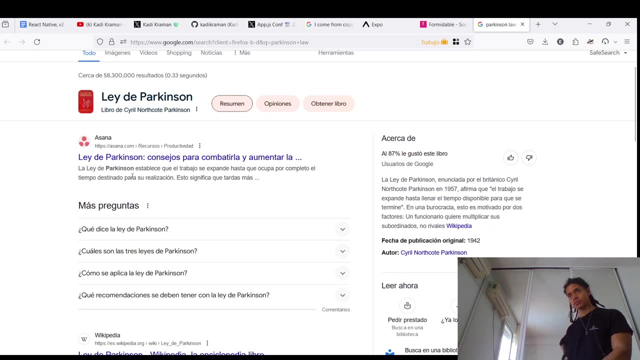 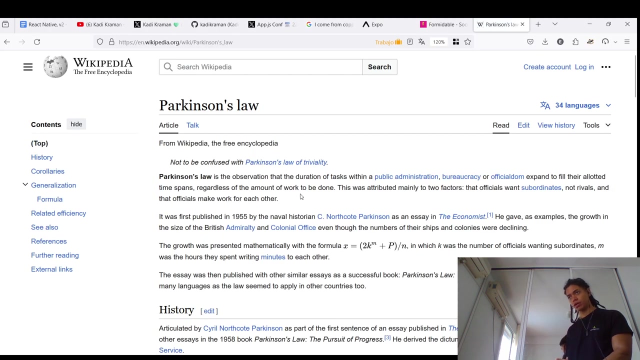 uh, which is one of the things that we can suffer from, which is the parkinson park parkinson law. okay, and the parkinson law here? why is now in english? so the parkinson law here, especially during a task within a public administration, bureaucracy and office of. 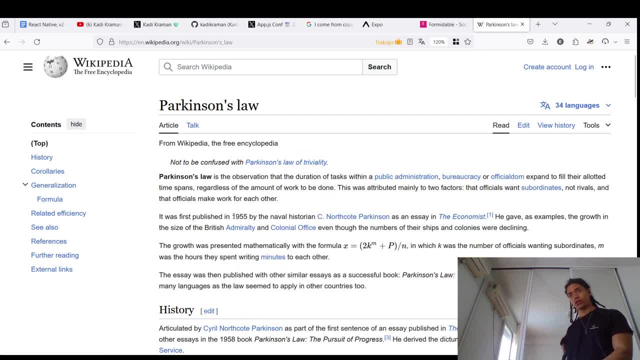 law is the same as the legal law in the parkinson law, so the parkinson law is actually used to define the time spent and the amount of time is done expand to fill their at all times spent, regardless of the amount of work to be done. this was actually. 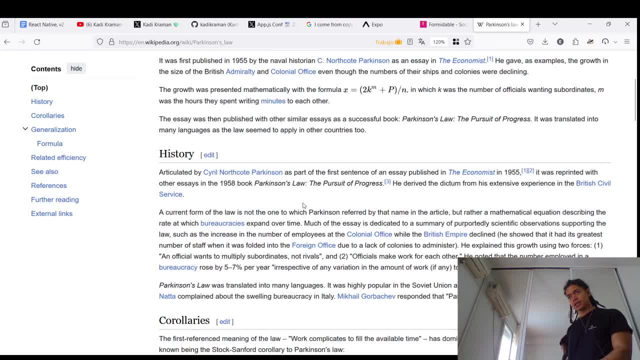 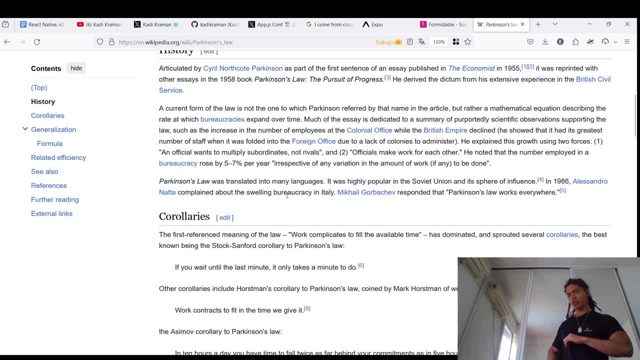 related to two factors: that official one subordinates, not rivaled, and that officer make work for each other. uh, so i need to also look at a little bit more about this. uh, work complicates to fill the availability, the available time. hear what it wants to brought up here from the wiki article, here from: 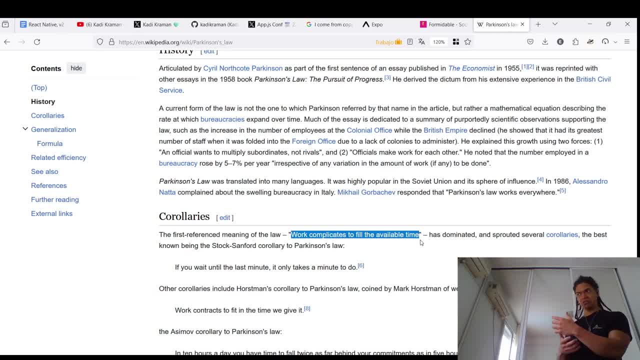 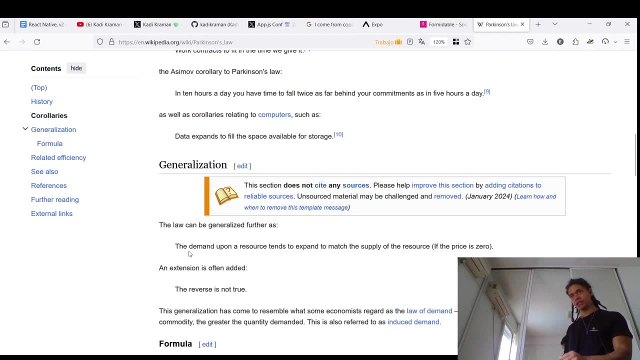 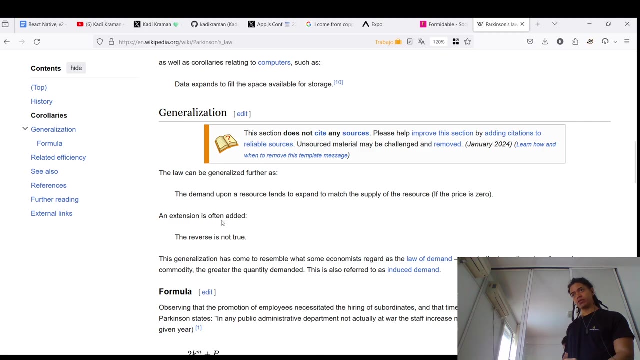 Parkinson Law. it's like as you work on the test you realize that it becomes more complicated than you expect, and now it's taking up your free time. so the idea here is to the generalization that the men upon a resource tend to extend to match the supply of the research, and essentially it's often added the 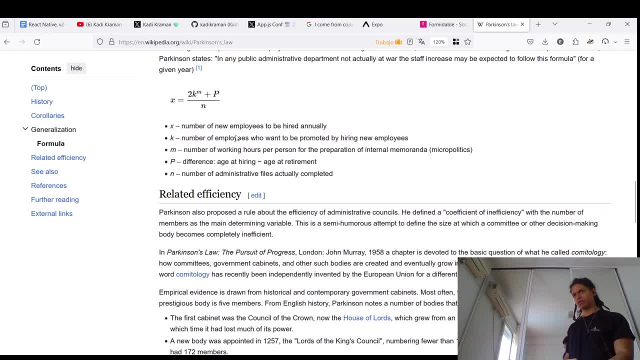 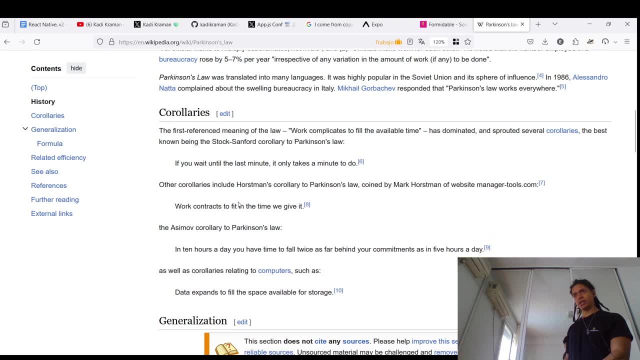 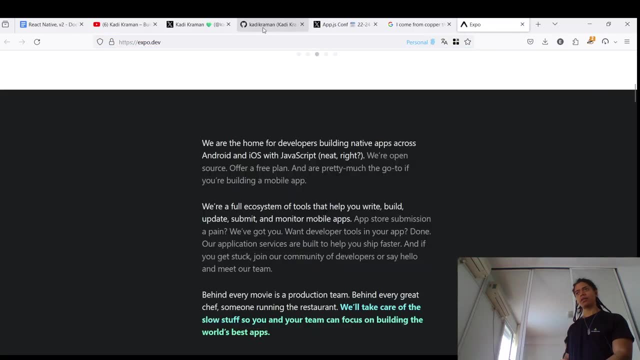 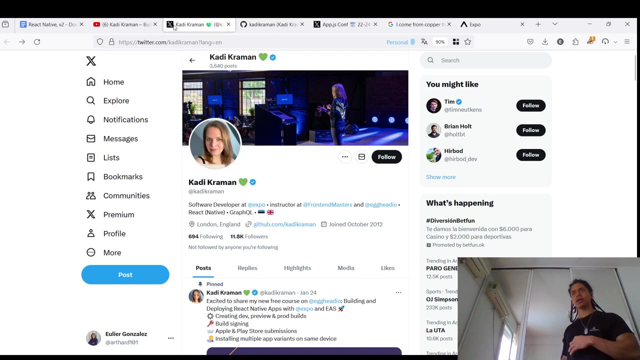 reverses is not true, and they even also create a formula here. oh yeah anyway. but yeah, this is Parkinson Law. the amount of work or content, especially if you talk about, you have to deal with the huge amount of data, in our particular cases, with react native as a way to make sense of who who 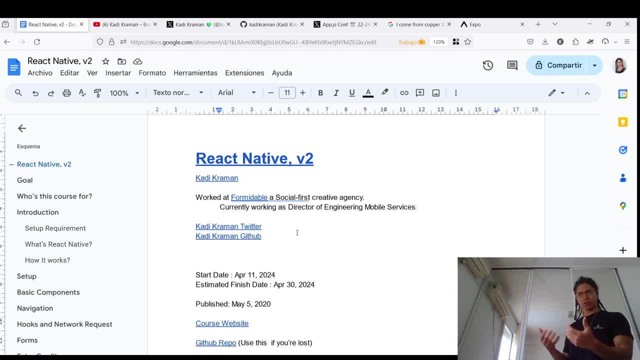 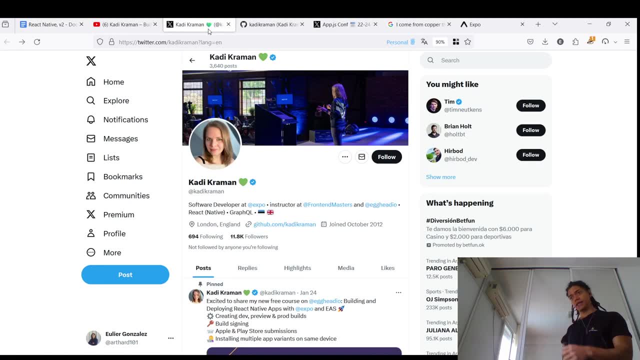 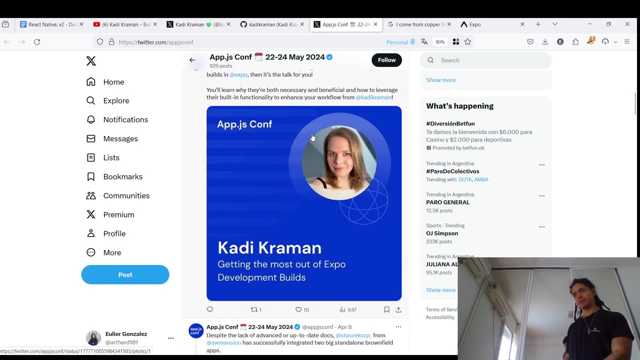 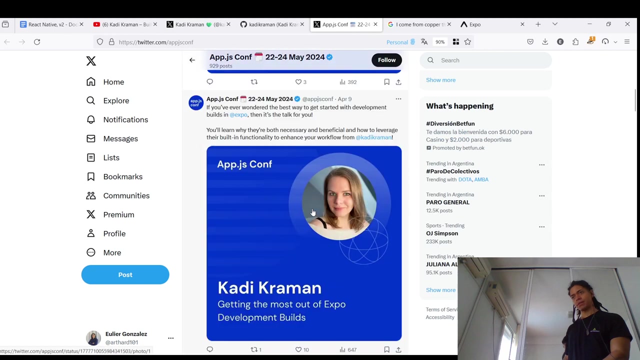 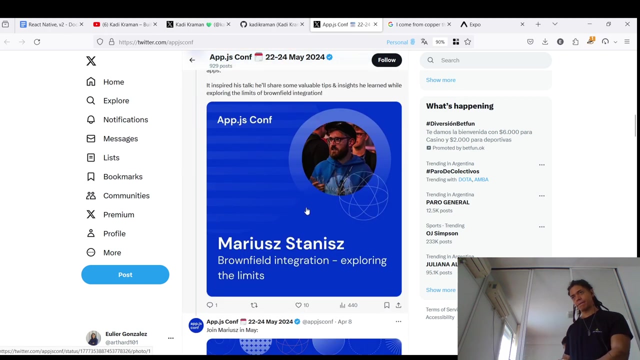 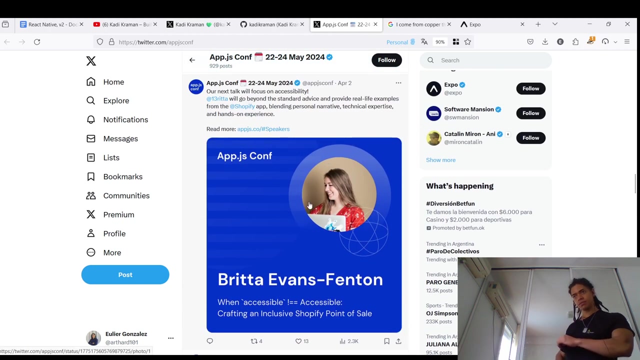 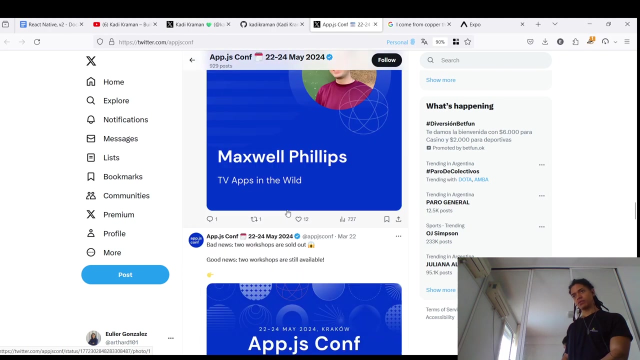 are you? what are you doing, why it is important to know what you have to say, what you have long in the past as well. so again, April on. okay, you know. alright, now for fella to be happy, and also- and I can't look in- for gold, that's. 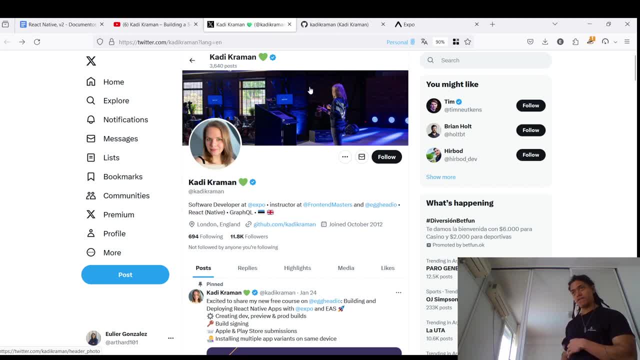 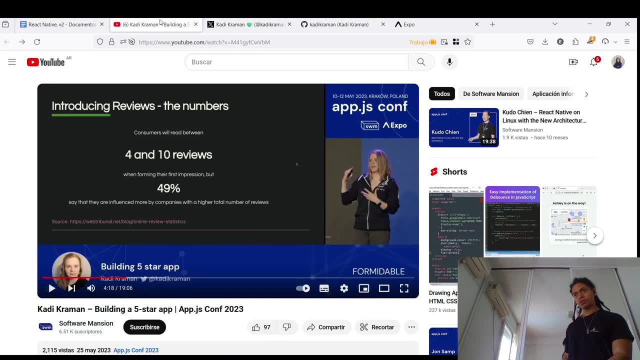 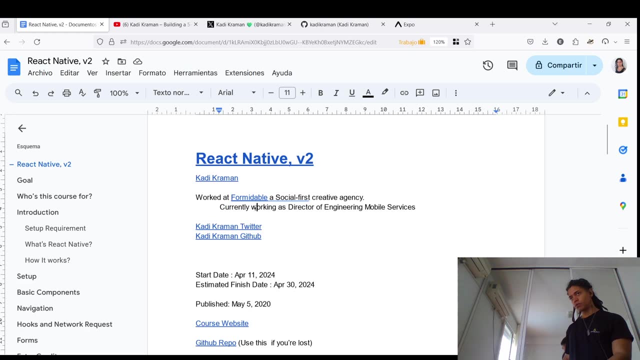 what happened here. I came looking for gold, you, And I found. I came looking for copper and I found gold. That's exactly it. So she is now working at, so work at Formidable, a social first creative agency, as director of like this, so as director, as director of engineering mobile service. 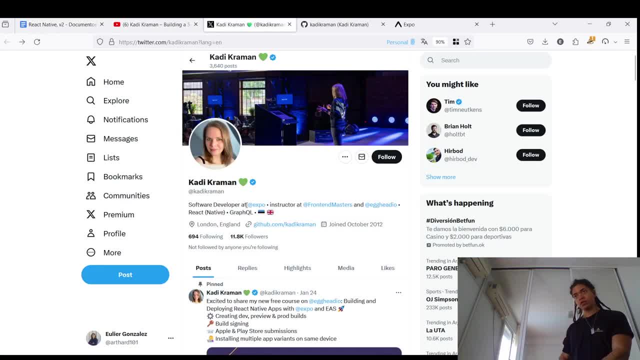 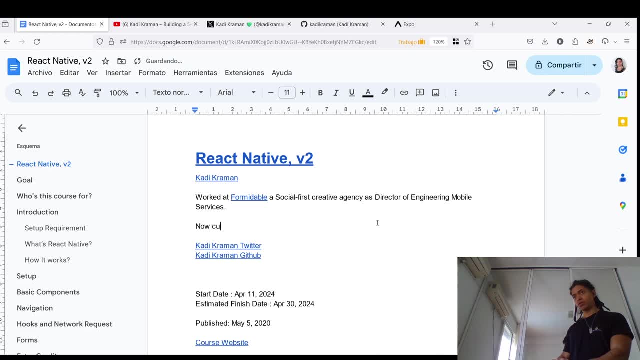 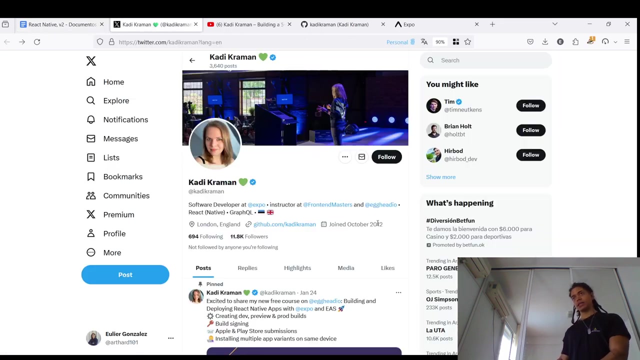 And now she is currently working as software developer at Expo. Okay, And now currently working as software engineering engineer, software or software developer, software developer, software developer at Expo. You may wonder: what is Expo? Expo Is this build tool for React application. 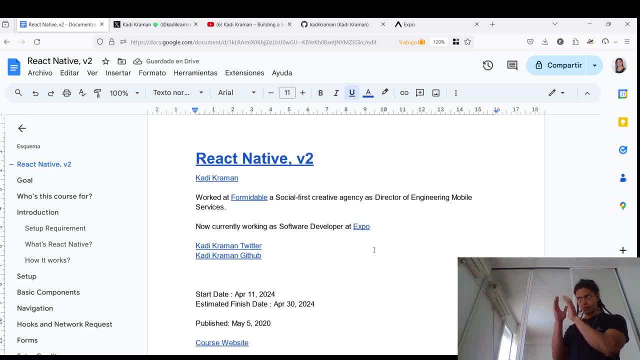 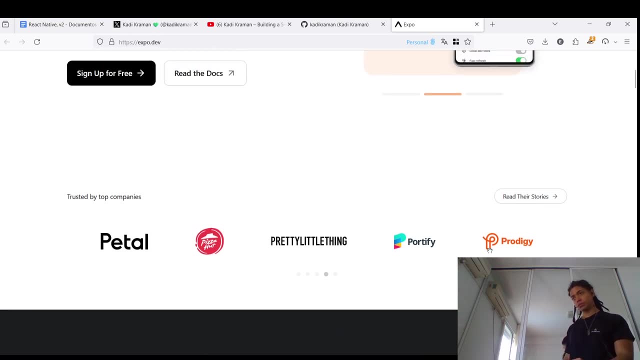 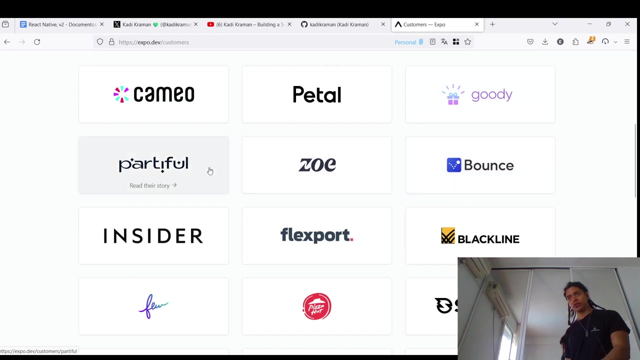 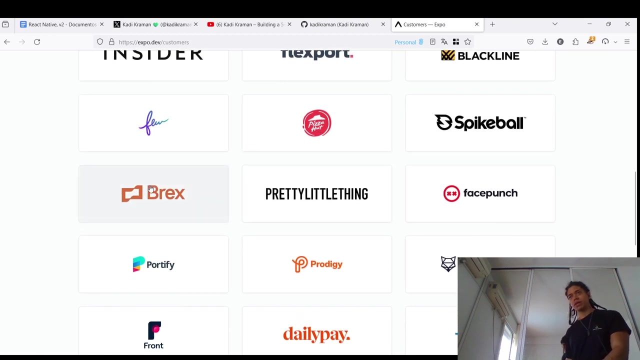 Is this ecosystem of tools, from writing, building, testing, deployed and monitoring mobile apps. Okay, It's interesting because this is also something that has been widely used. Okay, That has been widely used by all of this, all of their stories here: Cameo, Petal, Goody, Bounso, Portable Insider Blackboard, even PixaHut. PixaHut is still alive. Oh, anyway, Brex, PagePunks- I've never seen a lot of this. 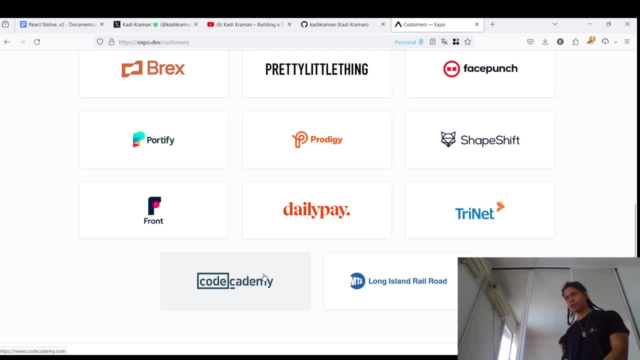 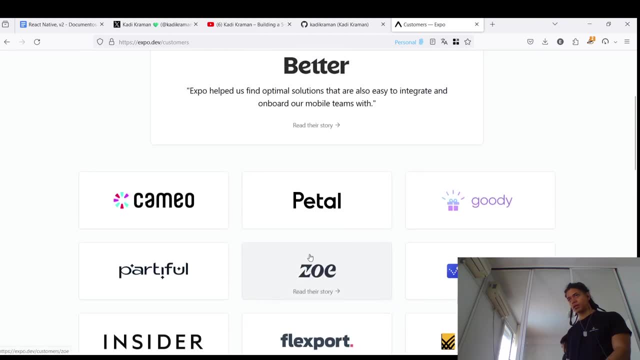 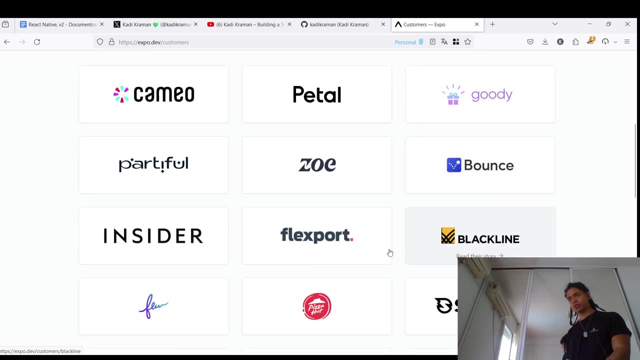 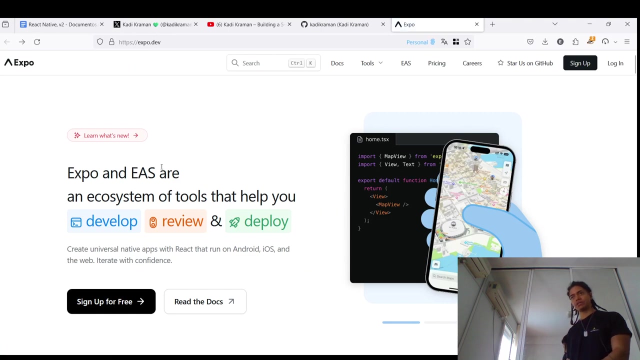 Cogacademy: Interesting, Cogacademy is using this. Okay, Cogacademy, This is just their use case. Interesting BlackLine, And there you go. Okay, so, But yeah, Is this Expo and ESA? 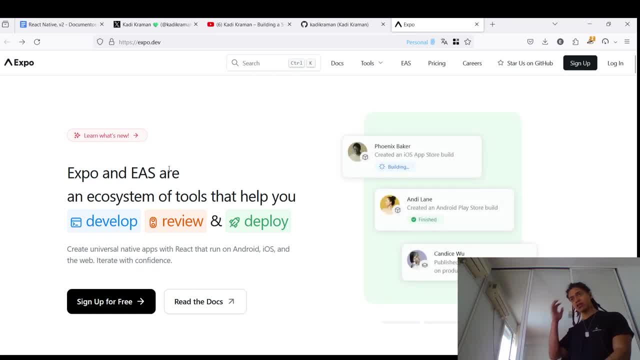 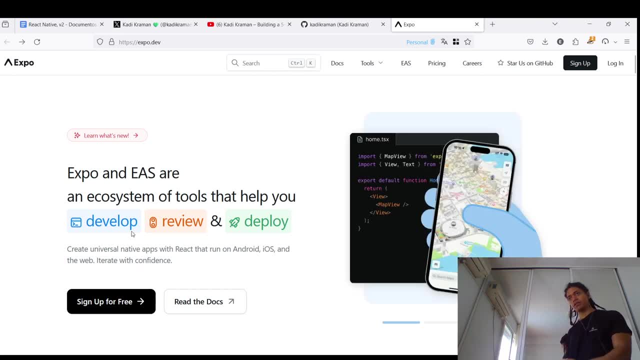 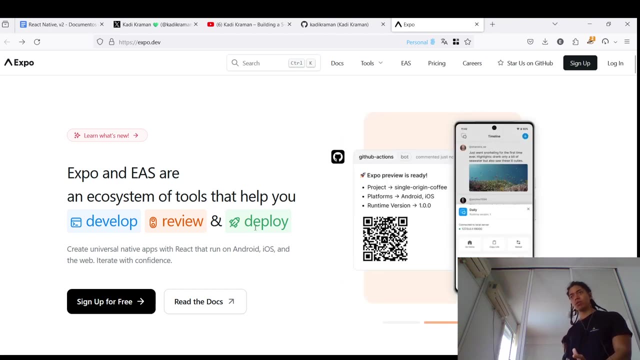 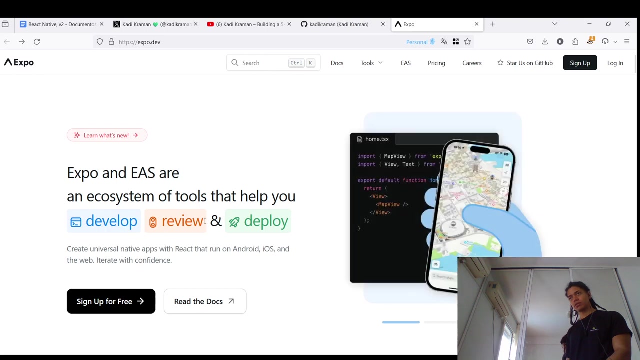 So I don't know what ESA mean Are an ecosystem of tools that help you to Develop, review and deploy- Yeah, develop, review and deploy What Mobile applications? Or create a universal native And deploy- Okay, and deploy. 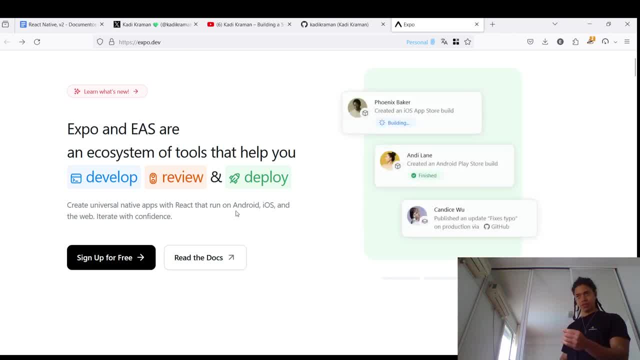 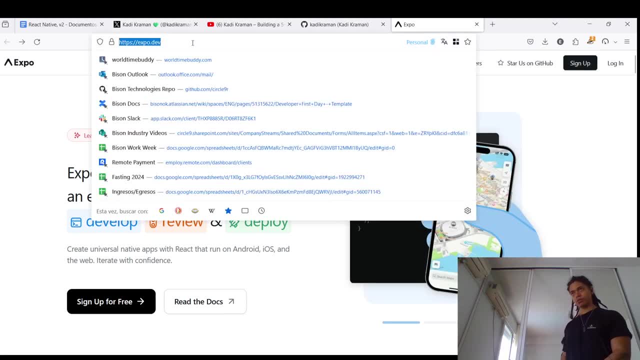 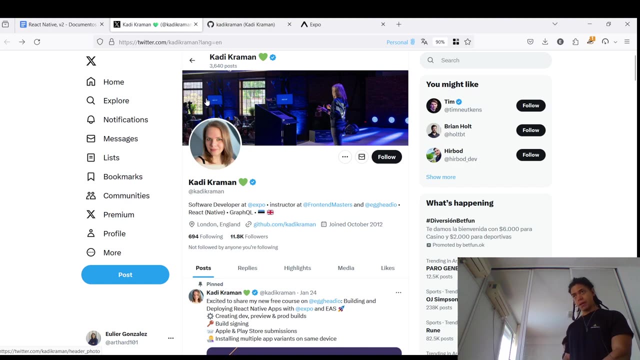 Jesus, Anyway, But they don't tell you what It's: Android and iOS application, I'm assuming here. So that's Expo. Okay, It makes a lot of sense, All right, Okay, cool, Cool, Cool. Cady Crammond. 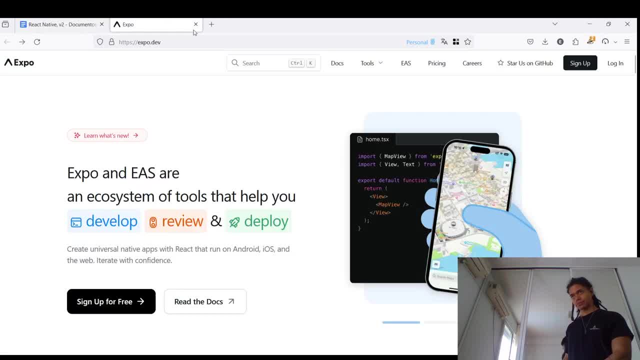 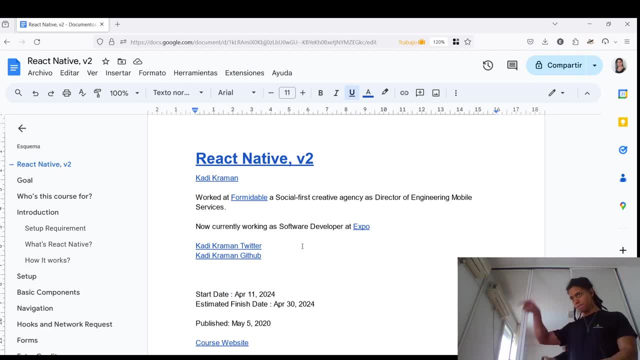 So Cady Crammond. she previously worked as director of engineering mobile service at Formula One, A social first creative agency, And now he's currently a software developer at Expo. So that's great, That's interesting. So with that little bit overview, okay. 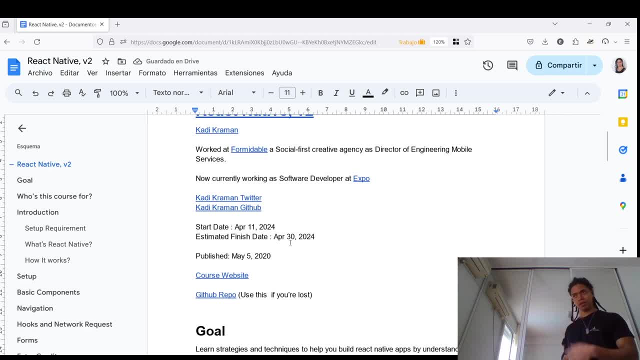 I have an estimate to finish this by April 30. right now We are in April 11th. We might or not reach that. perhaps, maybe i need to try to do that in the next 10 days. in the next 10 days i can. 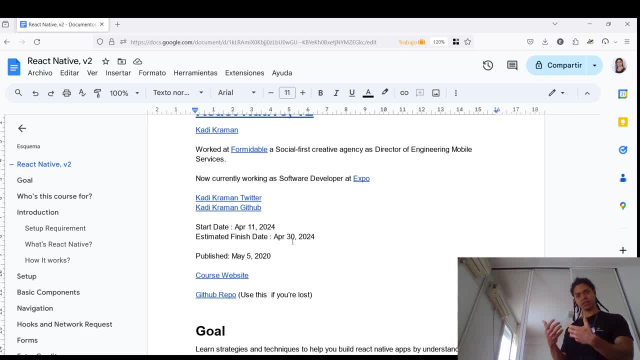 actually be able to articulate all of these ideas and what i need to express, what i need to explain myself, uh, to other college, whether they are tech savvy or not and be capable to understand those requirements, uh, and translate it into code. so that's the idea here. 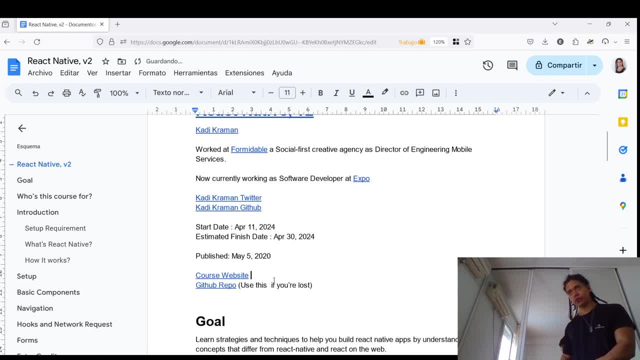 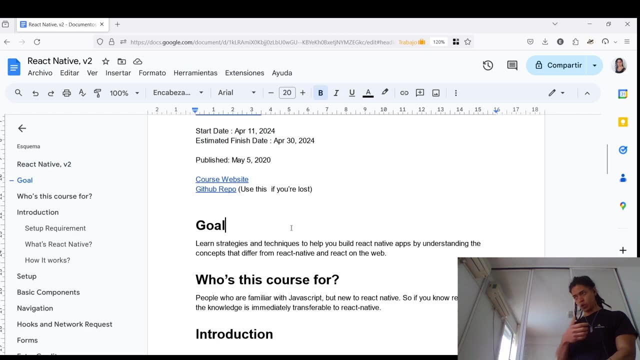 all right, that's, that's great, that's interesting. uh, and yeah, this course was published, uh, my, in may 5, in 20 to 2020, so the goal of this is just to learn this already and totally build that. we need to build react native applications by understanding, is there? 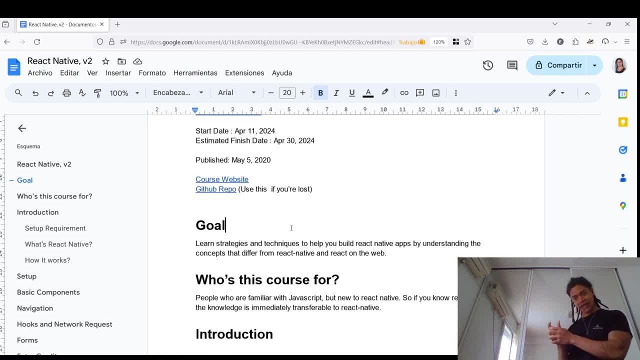 concepts that differ from react native and react on the web. okay, so, in order to build this kind of, in order to build this mobile applications, whether it's from uh, ios and android, we're going to use react native and also uh react native applications. so that's the goal of this course. 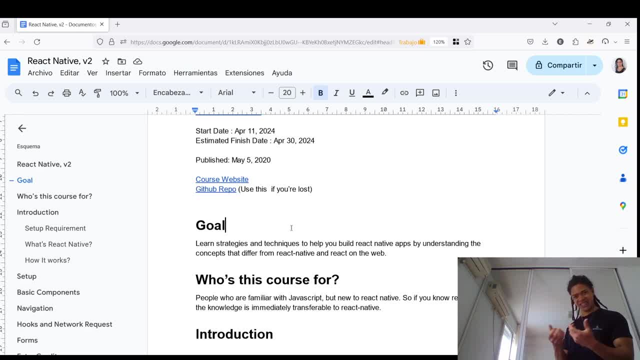 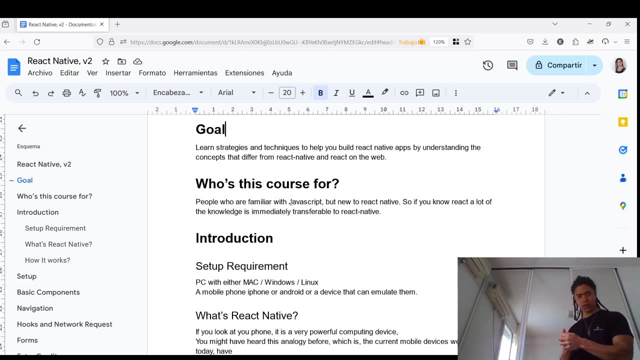 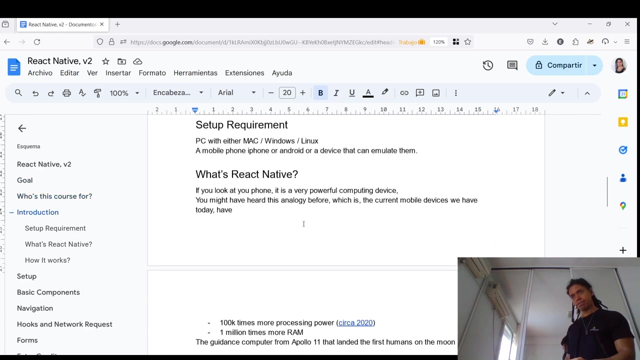 also the thing that we need to understand the jargon, the concept that defer, is react native from react on the web. okay, so who is this called for for? any task with developers that wants to build react native applications, whether it's for their job or because they actually want to do that out of it. and 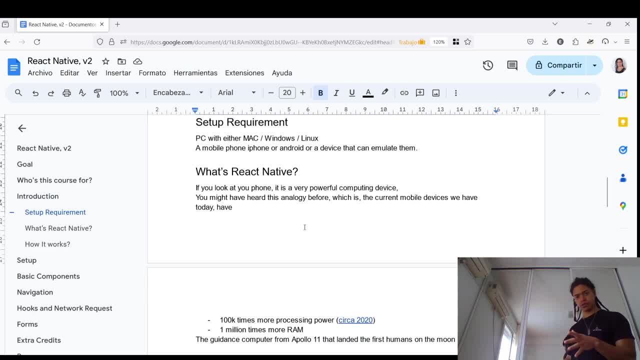 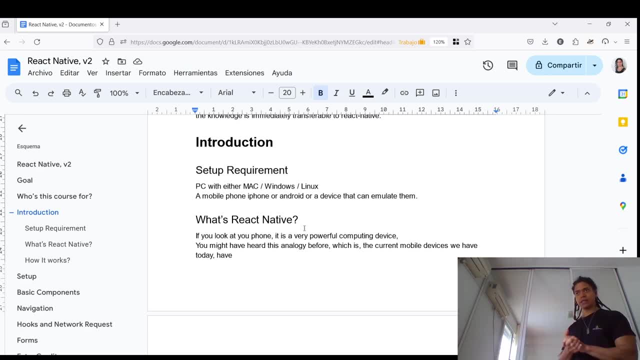 here's some couple descriptions and a little bit of introduction. here is a way to understand: is the setup that you need to, especially for running your application, and a little bit of history for context of react. why is it? this is important because I thought you're going to need is an old you need. 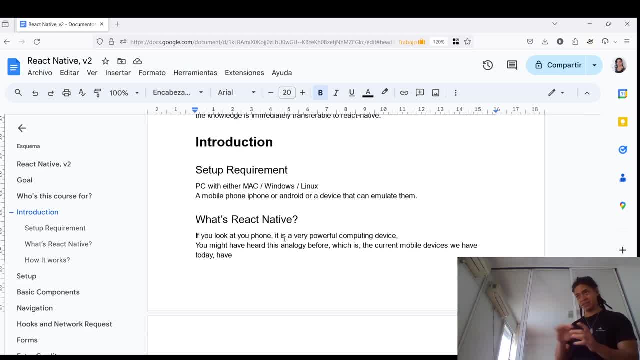 a Mac or Windows or Linux, IPC and a mobile phone or iPhone or Android. most of the time I am why heavily exposed to Android, because I'm come from Latin America and they think you need a Mac or a Windows or Linux or a PC and a mobile phone or whatever you. 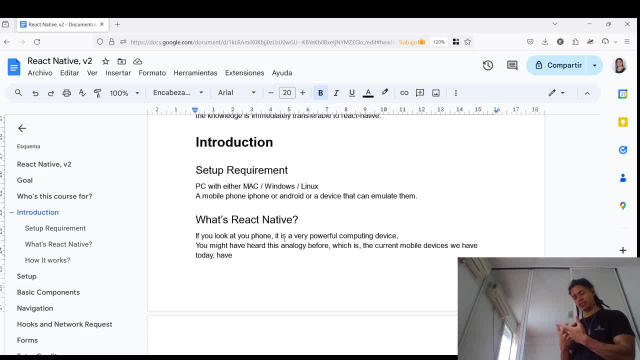 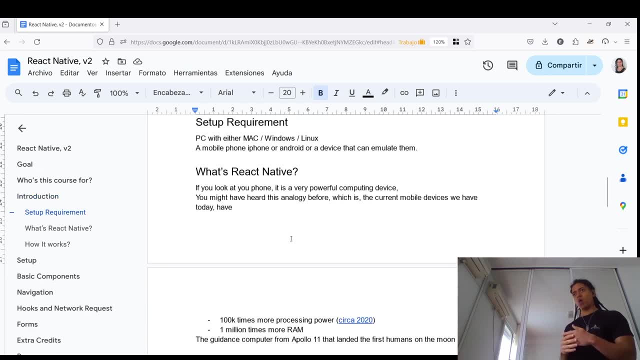 most of the time I am why heavily exposed to Android, because I'm come from here- is that it is time to take a look now at the iPhone ecosystem. so why, what is react? then we're gonna look why react. why react- native, okay. so, because our mobile device, or mobile device right now, has massive computer, has massive 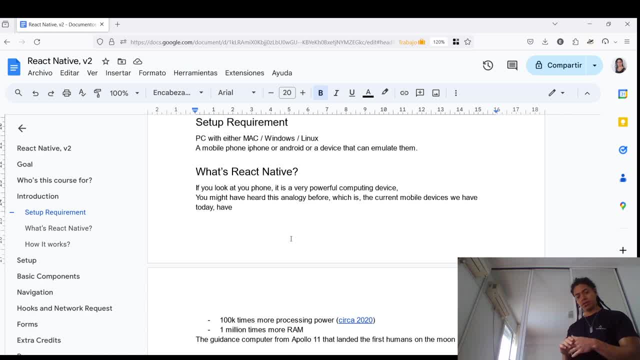 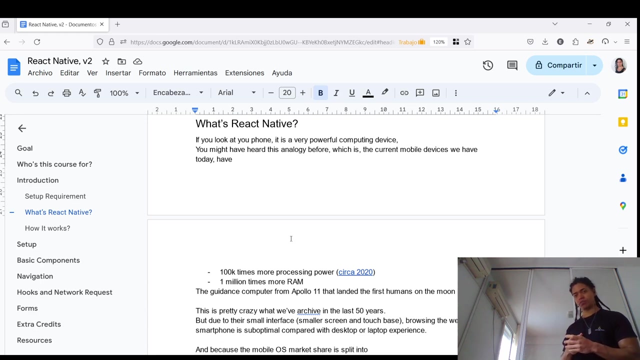 computer, because now our mobile device has no massive processing power. you might have, you my her, you might have heard of this analogy before where, like the green mobile device has now more than one hundred thousand, the green mobile device has now more than one hundred thousand times processing power and one million times more. 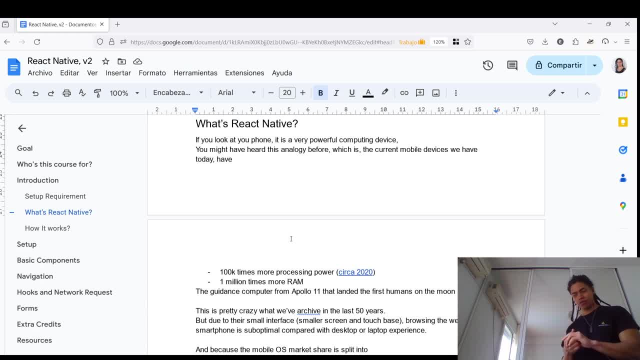 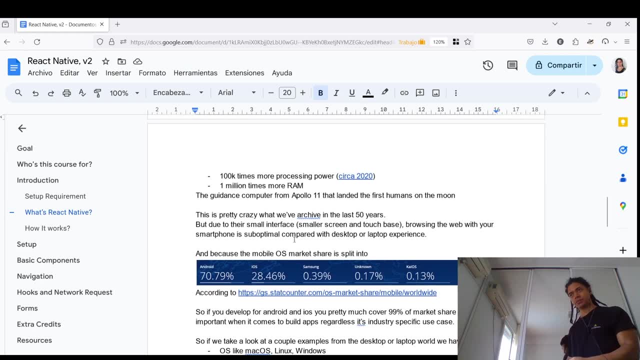 times processing power and one million times more ran than the guiding computer from Apollo that land the ran than the guiding computer from Apollo that land the first humans on the moon. and now the US can show up and first humans on the moon. and now the US can show up and say we did it right. they can, that we did it. so that's great, that's. 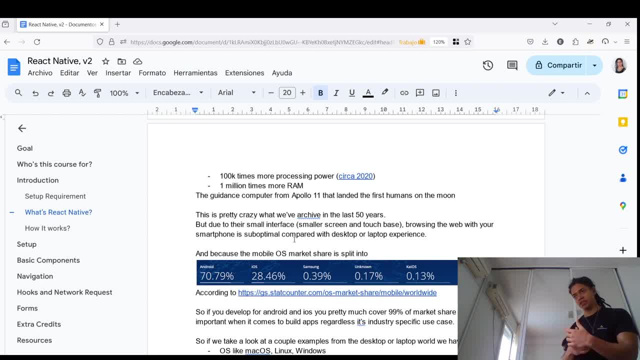 say: we did it right. they can that we did it. so that's great, that's great and over the. this is pretty crazy because we great and over the. this is pretty crazy because we achieved this, we are chief. we achieved this, we are chief. we are here. so we achieve this in the in the past. 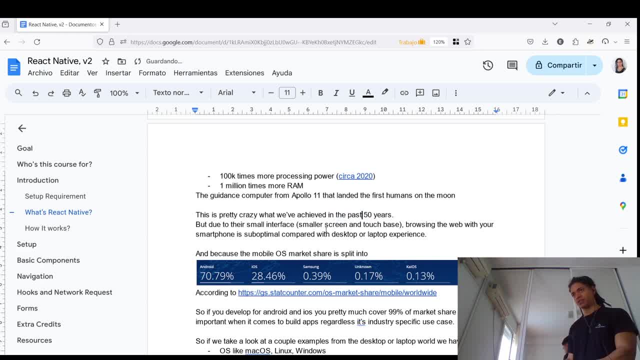 are here, so we achieve this in the in the past. are here, so we achieve this in the in the past, in the past 50 years. okay, so well. because these devices are in the past 50 years. okay, so well, because these devices are in the past 50 years. okay, so well. because these devices are small, because these devices has a small 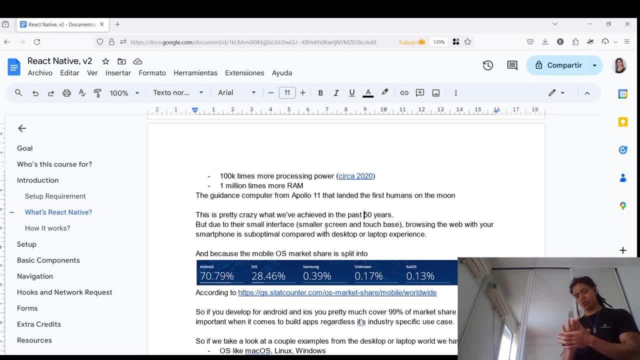 small because these devices has a small small because these devices has a small interface and they have a small touch interface and they have a small touch interface and they have a small touch base- its most green. their web browsing base: its most green. their web browsing base, its most green. their web browsing spirit is suboptimal, then desktop or 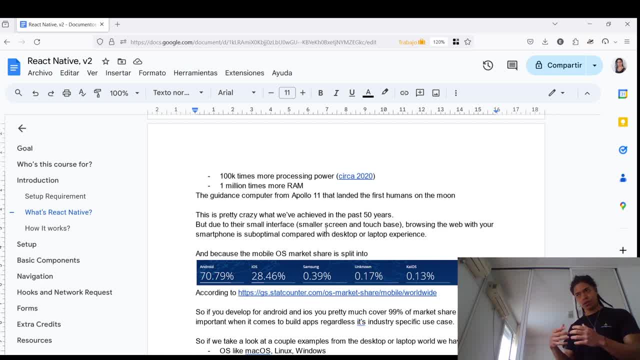 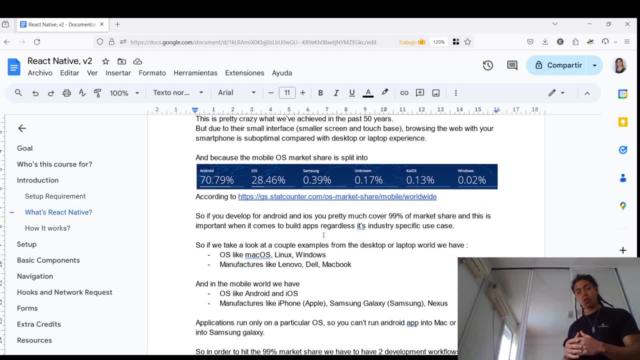 spirit is suboptimal, then desktop. or spirit is suboptimal, then desktop or laptop experience, so laptop experience, so laptop experience. so even, even even though the mobile marketplace, though the mobile marketplace, though the mobile marketplace worldwide is include that seventy percent of the worldwide is, include that seventy percent of the 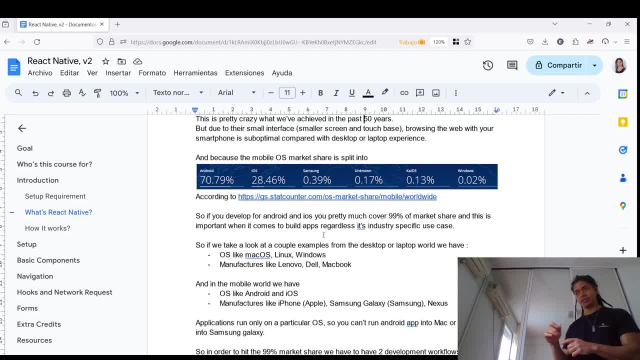 worldwide is include that seventy percent of the population use Android, whereas the population use Android, whereas the population use Android, whereas the iOS is being used by twenty point forty six. iOS is being used by twenty point forty six. iOS is being used by twenty point forty six. the point here is that a lot of the 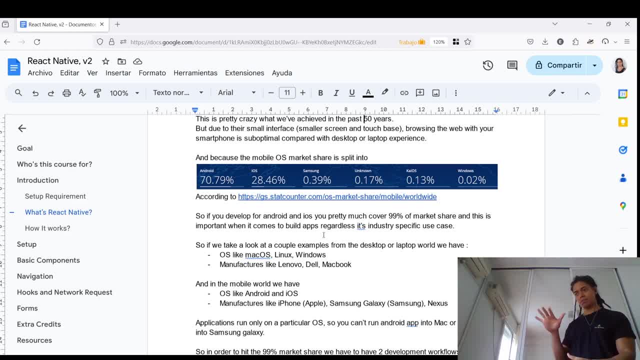 the point here is that a lot of the. the point here is that a lot of the people that you might know from the US, people that you might know from the US, people that you might know from the US or Europe they might use is, or Europe they might use is. 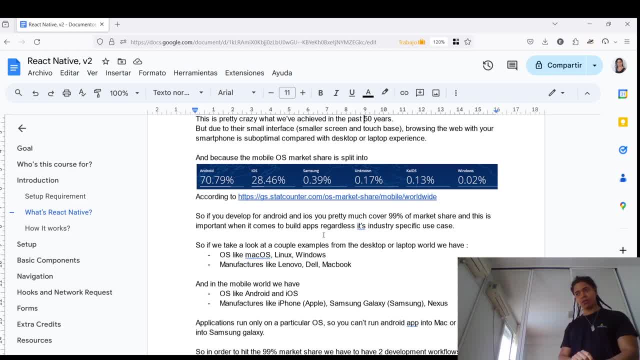 or Europe they might use is iPhone, but for example, in places like iPhone. but for example in places like iPhone. but for example, in places like left-hand, where honestly it's to me, left-hand, where honestly it's to me, left-hand, where honestly it's to me. isn't it quite up top that barely people 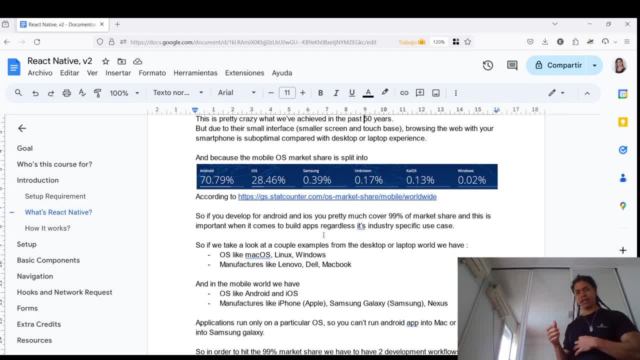 isn't it quite up top that? barely people. isn't it quite up top that, barely people that do this kind of comfort. they, they that do this kind of comfort, they, they that do this kind of comfort. they, they don't even mention about left-hand is, don't even mention about left-hand is. 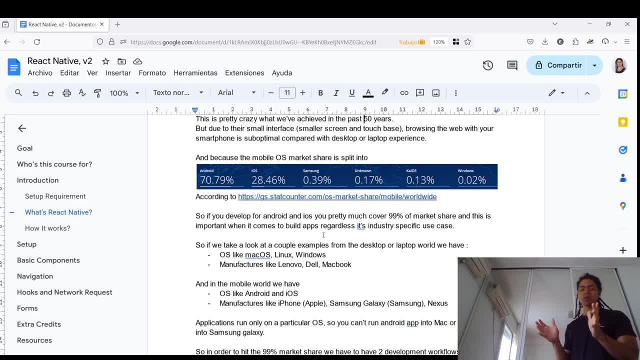 don't even mention about left-hand- is like a lot of time doesn't exist. well, I like a lot of time doesn't exist. well, I like a lot of time doesn't exist. well, I hope that can change over time, and we hope that can change over time and we. 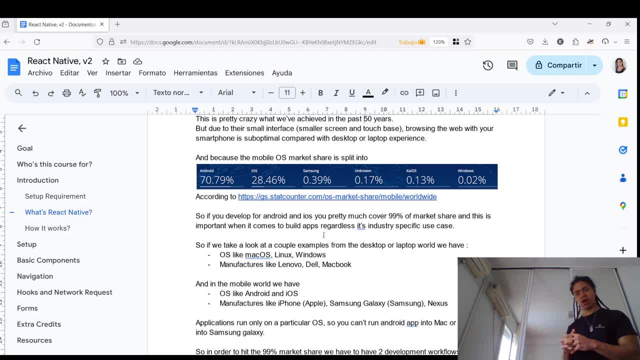 hope that can change over time and we can be more competent. we can understand, can be more competent. we can understand, can be more competent. we can understand why we are here in the blessings, that why we are here in the blessings, that why we are here in the blessings that we get by being this land anyway. but 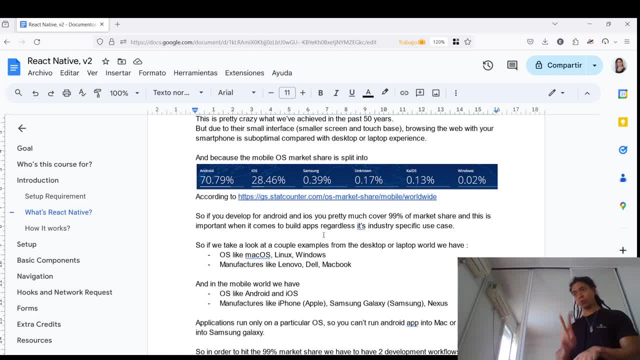 we get by being this land anyway. but we get by being this land anyway. but yeah, the places like India. they only, yeah, the places like India. they only yeah, the places like India. they only have 2%- roughly 2%, of users of iOS for. have 2%, roughly 2%, of users of iOS for. 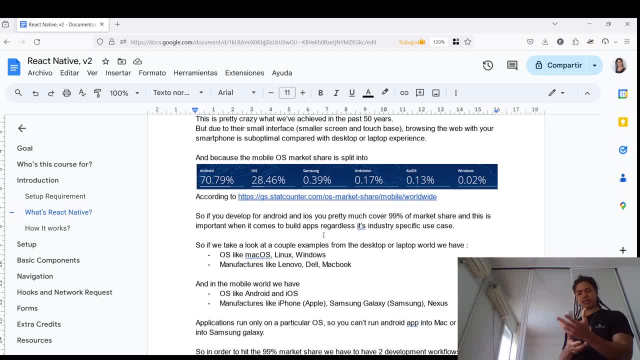 have 2%, roughly 2% of users of iOS for iPhone users. so because this iPhone users, so because this iPhone users, so because this discrepancy exists, you can pretty much discrepancy exists. you can pretty much discrepancy exists. you can pretty much cover, cover, cover, 99% of the market share if you build applications on Android and iOS. so for 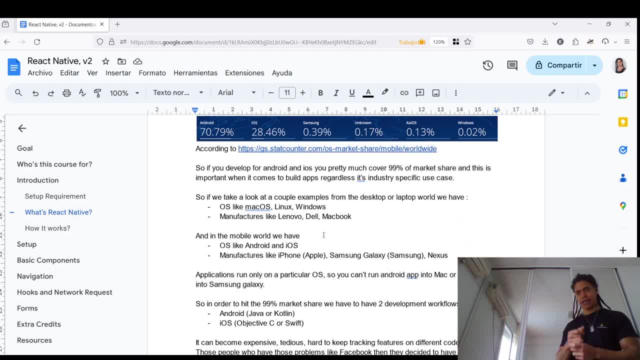 example, OS like Mac OS, Linux and Windows. they have manufacturers on device run on top of this hardware, whether it is manufacturing hardware, whether it is from Lenovo, Dell or MacBook, and in the case of the mobile we have now OS like Android and iOS was several bunch of them. the most dominant are these these: 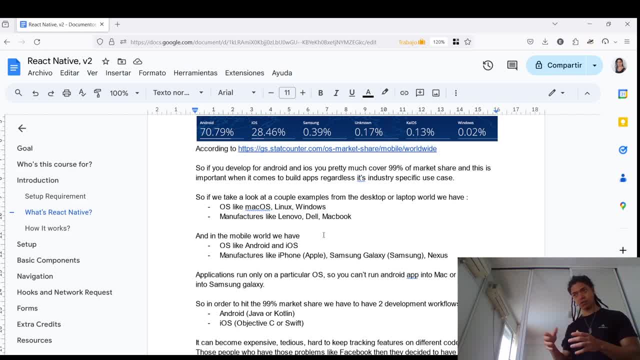 two, and the devices that it can run can be iPhones, Samsung Galaxy Nexus, iPhone, Apple, the iOS and Samsung Galaxy Nexus using Android. so because applications run on their particular OS. so if you have an application that is built for Android, it won't be. it won't work on iOS, similar to Linux, it only works there. 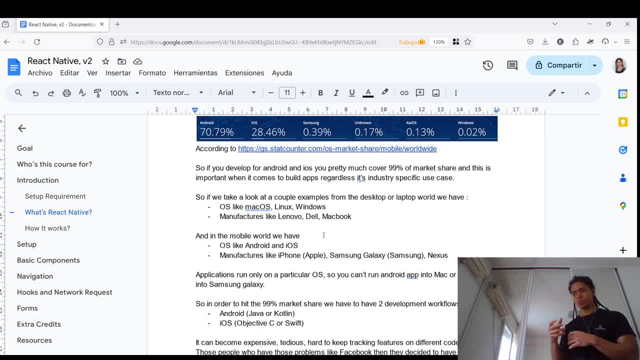 not on Windows. so because of this giving obligations and in order to hit 99% of market share, we have to development work located. she described a lot of things which is very, very, very important to me. first is the ability to describe: how do we get here? 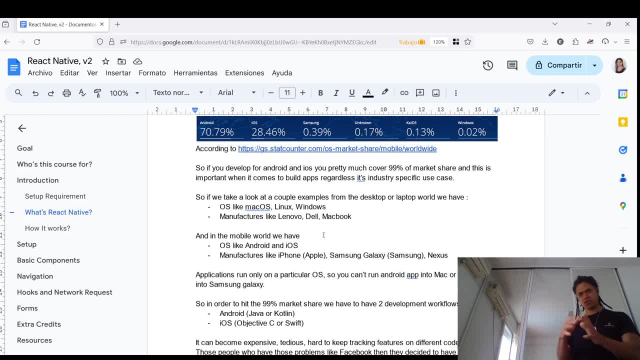 very, very important. a little bit of history for context, and then how we move on to recognize what are the different environments that we can build applications. where can we is now use this device? what are the main use case of our device, for example, in the case of mobile browser, in browsing the internet, in how, from there, we look at. 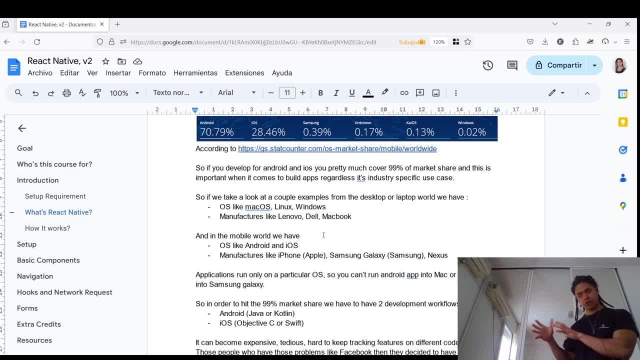 now at the market share as a way to recognize this reality, especially when you needs to build applications in from which platform you want to build applications, because those are where the eyeballs are. yes, should are in the what the people actually are using, because he wants to. 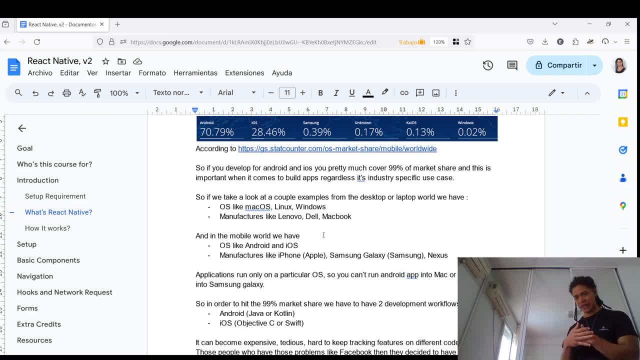 target 100%, or at least 99%, of all the devices in that in the mobile market. so we need to understand a little bit of basics, which is the reason why we City- yeah, the ger in the web. let's say what audience looking at this mobile. 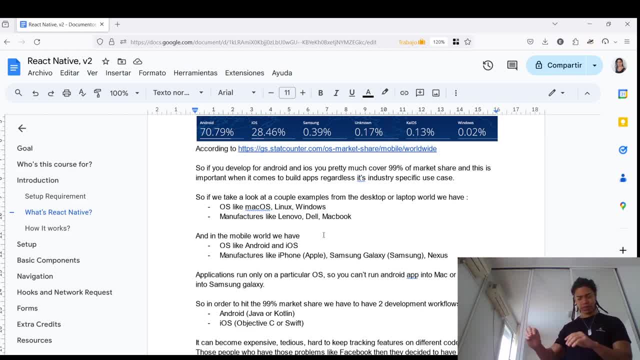 market share this OS in? how about running applications in one place or another? so, for example, why by running application on OS, it doesn't work on app or Android and y by running applications on Android, it doesn't work on IOS. then they are now talking to different architectures. so a good analogy of this: 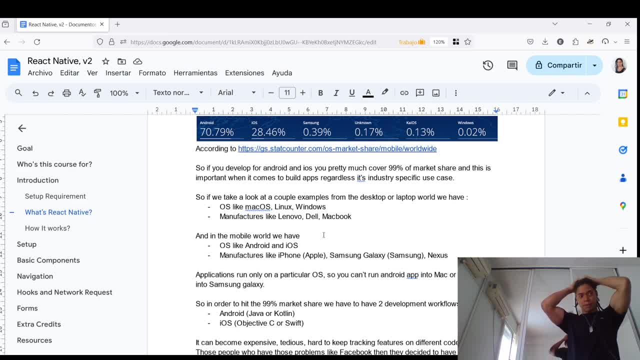 is like you're trying to build a house with people that know in there, or the people that know Spanish and you are an English speaker. it won't work or not in the expected timeline. so in the case of them as different from us, we can learn each other along the way, but unfortunately for this kind of device, 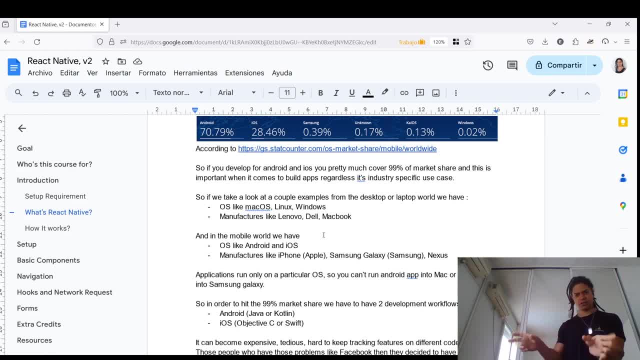 they are just a fixed set of instructions, so they are not capable of learning. so, but in every case it exists right discrepancy, which, in the case of only applications, which can become quite tedious because now you have two different workflows, one of them is for Android and the other is for iOS, and so 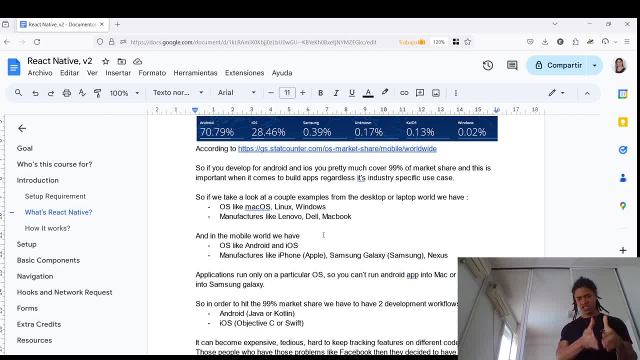 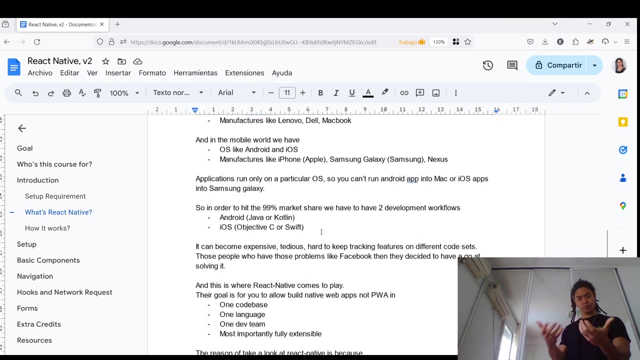 for example, in Android you need to run is or you need Java or Kotlin- something that I quite a little bit more familiar with- and the other is on the iOS, you have a Jack to see or Swift. okay, so it can become expensive, tedious, hard to keep track of different features on different code sets and those people. 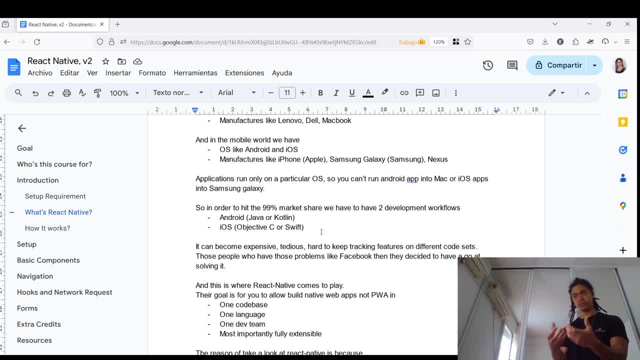 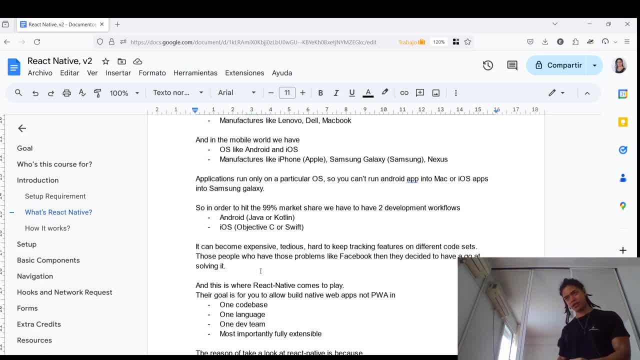 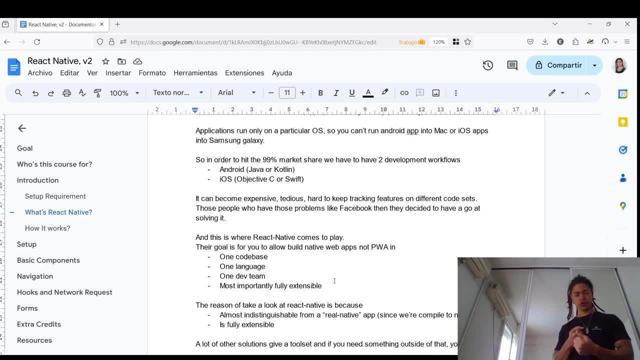 decide to have a go at solving it. interesting, so they decide to have a go at solving it very, very, very important, very, very, very important. so this is where react native comes to play- is because those big company actually now are facing a lot of problems. they are at the frontier and now they have to build, particularly 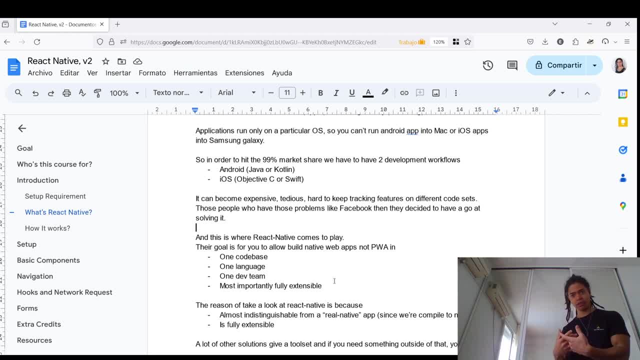 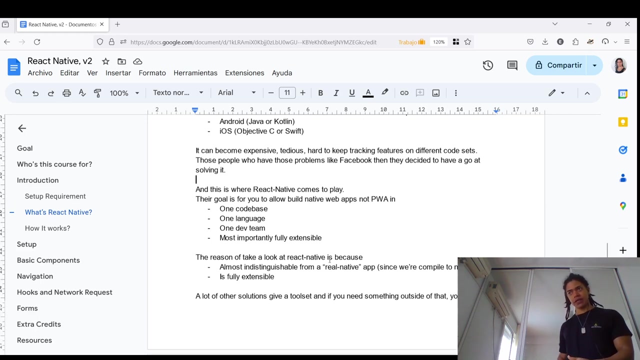 stridey techniques in systems that help when, that help them to now deal with the entropy, deal with the mess facing their own problems. in this case, building web application as well as native mobile application or that behave similar to that. so that's where, in the case of react, native comes into play, and 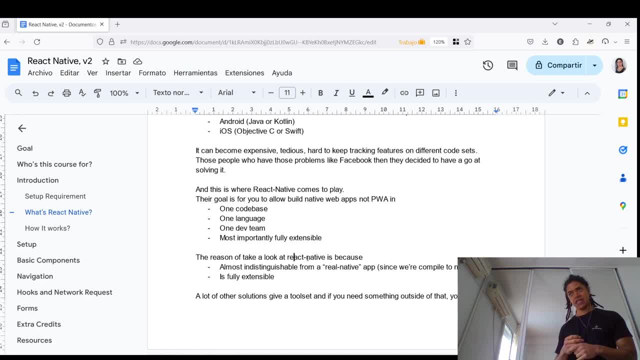 in the idea of this is to well, because we have now this particular problems. we have two different workflows workflows. one of them is for Android, using Kotlin or Java or Kotlin. the other is using iOS, with object to see in Swift. so we need to find a way here, okay, to actually simplify the workflow. only one. 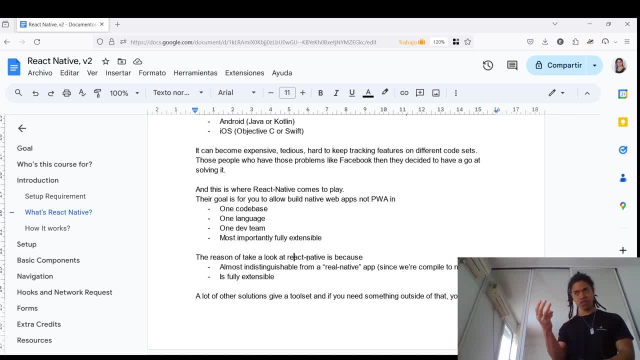 workflow, only one language with all, with one dev theme and, most importantly, okay, fully extensible. okay. so, in case of all that, when you work with other platforms, I only native script, so they provide you a set of toolbox, and when you need something outside of that or when you want to create something, 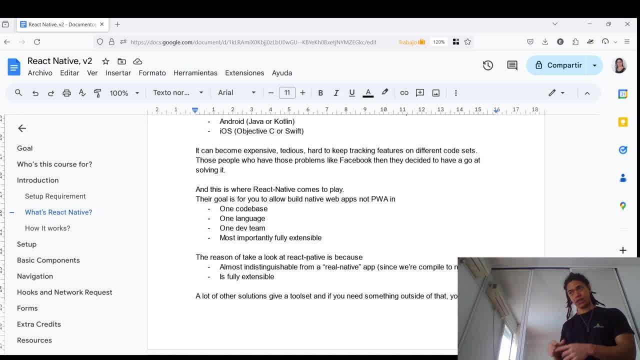 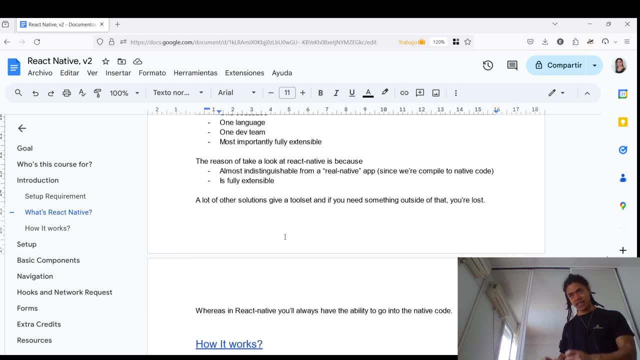 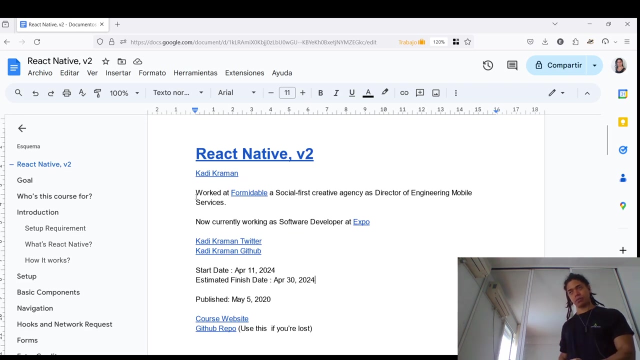 outside of that, you aren't by your own. your loss, that's what happened. so the idea of looking, now react, maybe because you also have the ability to go in to the native code, according to cat right. according to. according to caddy grandma, according to caddy. 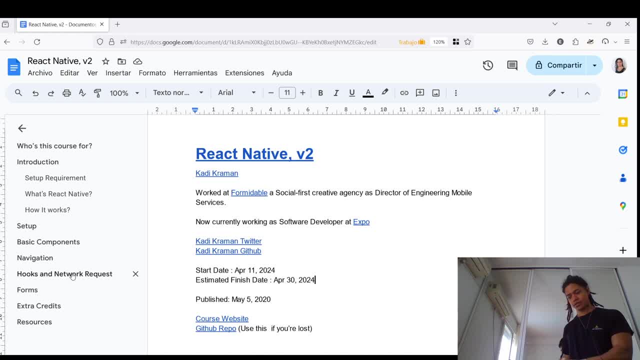 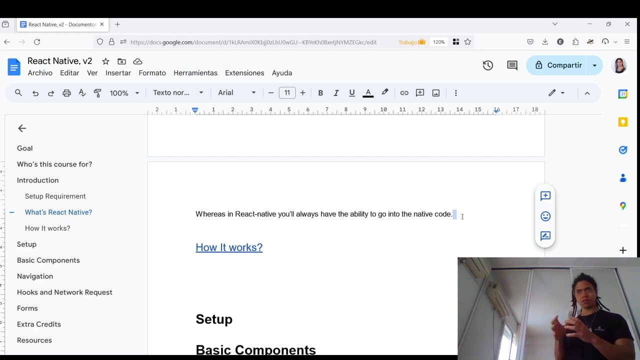 catty catty. ok, creation command ëc storyí. okay, so you got it good, good, good. this was just a little bit of intro to get myself familiar with that. so what is the sort of requirements? what react native? what react native and createンメI mean in Learningmedias bycelial program. but 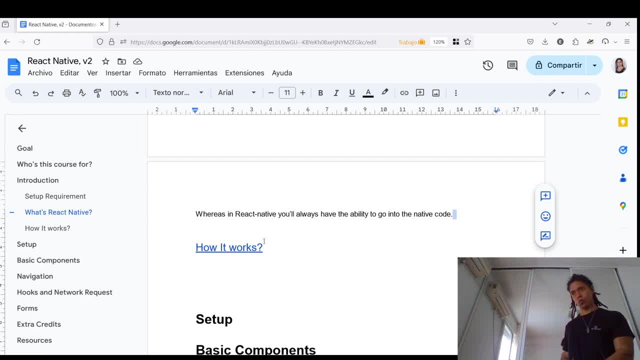 is and how it works. okay, i think this is very, very, very important as a way to get- but not only as a way to gain- perspective in the industry, but also the way to understand is and to improve your communication skills. you need to tell or you need to talk to college or someone outside of that. 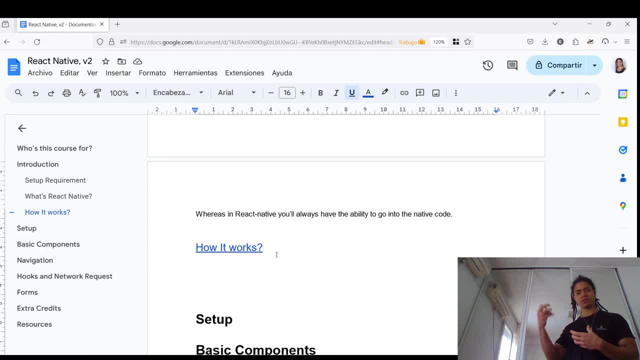 so try to describe this story as much as possible, but try to describe this story in the most succinct and sure, the most succinct possible way, in the most succinct and effective way. that's the idea of doing this. all right, yep, yeah, believe me. yeah, it is so good how it works. 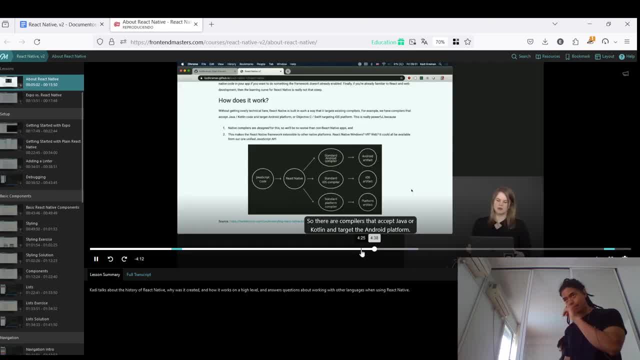 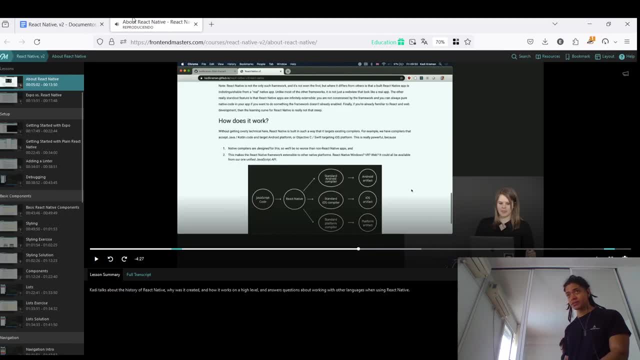 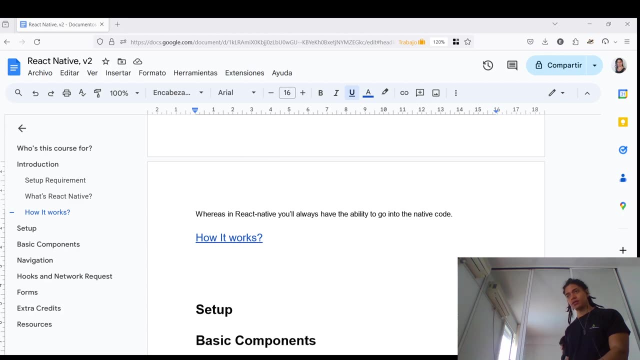 how it works, okay, oh, um, yeah, that's right, you can see this. sorry, not sorry, what exactly exactly? okay, uh, i'll be right back. okay, uh, i'll be right back. okay, i'll be right back, Thank you, Thank you, Thank you, All right. 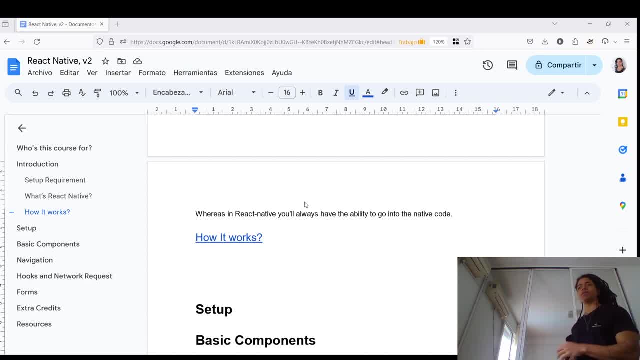 So right now, what I'm going to do is just taking notes of that particular course. So that's the reason why you're not able to see what I'm going to do. That's fine. So yeah, maybe this is actually the third or the only such library that aims to do this. 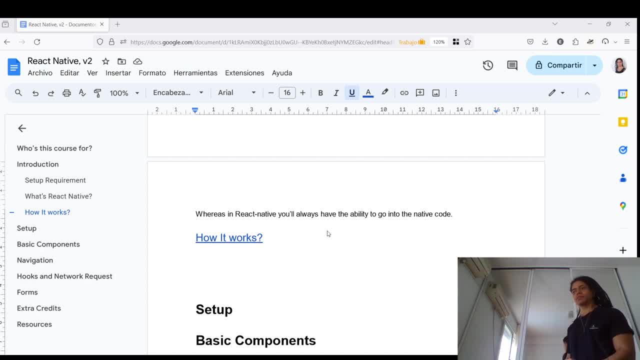 But it is incredibly powerful and arguably the best. But this is because A we're building fully native web apps, so the compiled React Native application is indistinguishable from a real native application. And secondly, because it's really expensive. 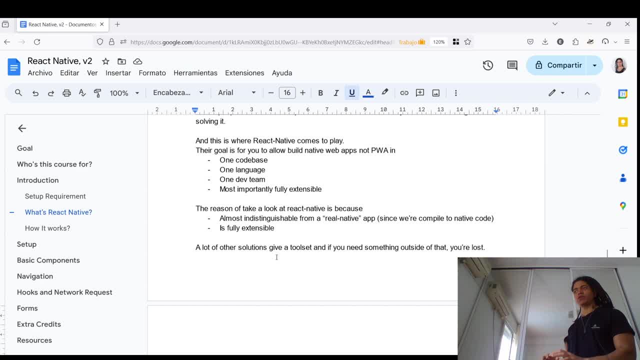 So That's one of the reasons why we're looking here at React Native and why it's important and powerful: Because it is almost indistinguishable. It is almost indistinguishable, Indistinguishable, It is almost indistinguishable. So it is almost indistinguishable from a real native app. 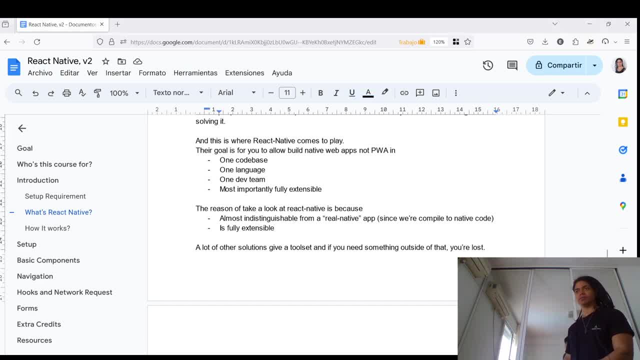 That's one of them And the other, So it's fully extensible. A little existing library. Basically, you can do this toolbox of things that you can do, But if you want to do anything outside of this, you're lost. 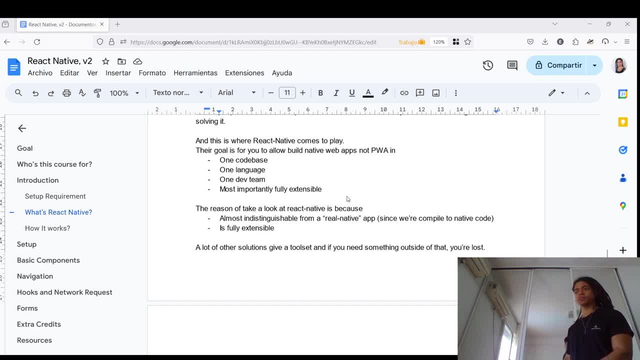 Whereas in React Native you can always- You always have the ability- to go into the native application and add into React Native the ability- Mm-hmm, It's fully extensible- by going into into the native code and add something that React Native doesn't. 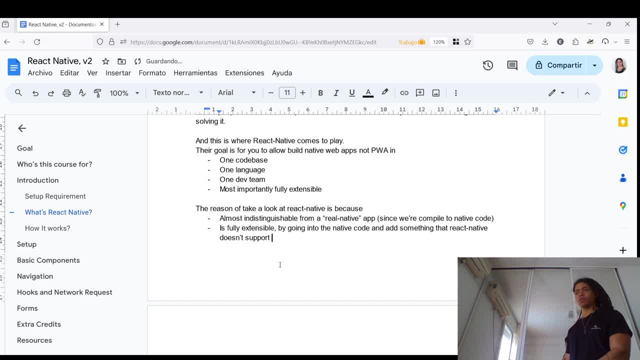 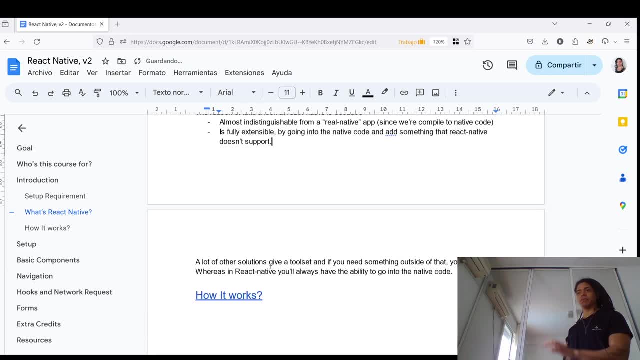 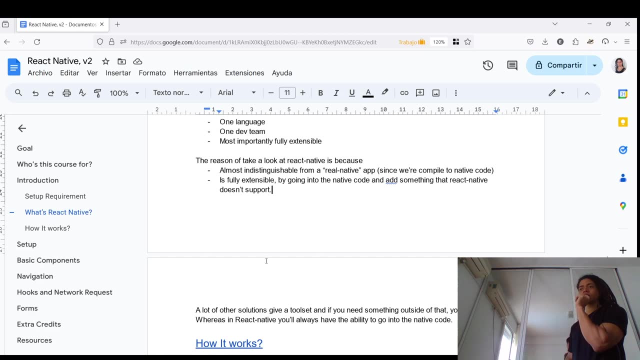 doesn't support, well, Or doesn't support, Mm-hmm, That's interesting, Okay, That's very, very, very interesting here. Okay, So this is the, the, the, Let's put it here. So benefits, you know. 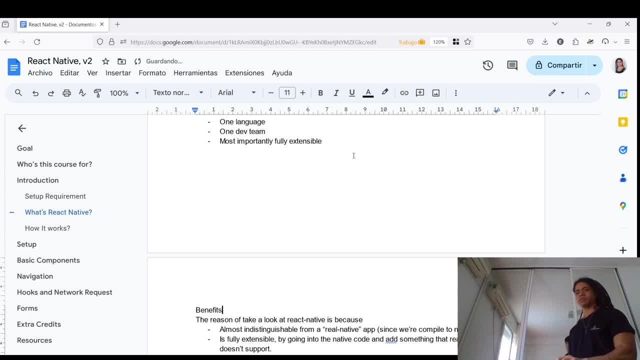 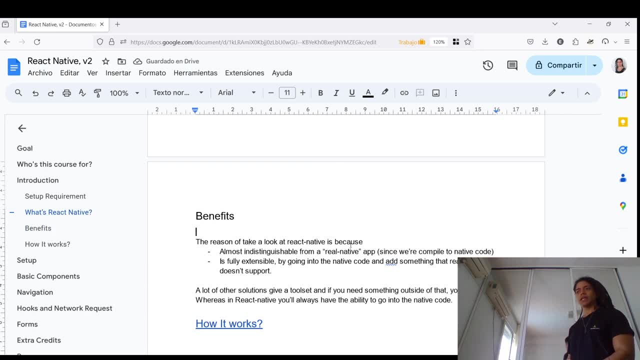 Benefits, Benefits. The reason to take a look at React Native is because besides, besides, besides- yeah, there's no, there's no- besides being powerful, powerful and powered by Google- oh, my mistake, my bad bro- by Facebook, like you, must be an agent. a Google agent by Facebook is almost indistinguishable from real. 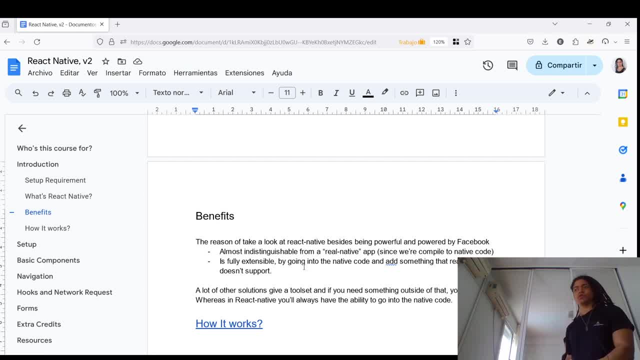 native apps. okay, so, since we have compiled to native code, okay, it is almost indistinguish- indistinguishable from real native apps and it's fully extensible by going into the native code and adding: okay, it's fully accessible by going to the native code and adding something that we 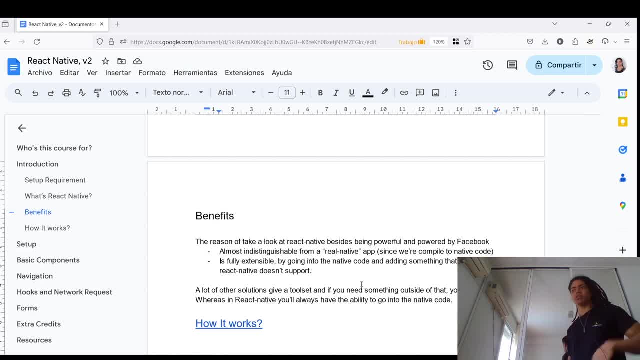 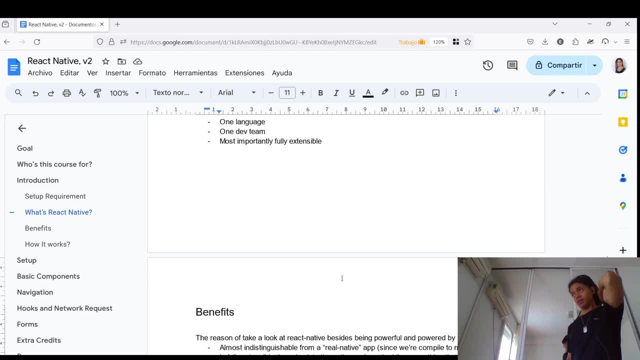 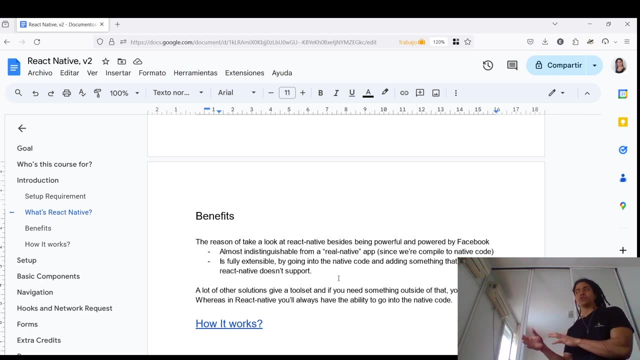 have needed doesn't support. interesting, and I think this is something very, very, very powerful. it's just one of the benefits of using the react, because a lot of other solutions. so they provide you a lot of things. they provide you a tool set, and if you need to make something outside of that, you're on your own, mm-hmm. 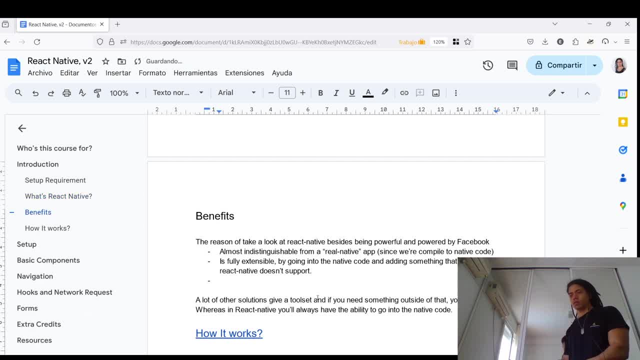 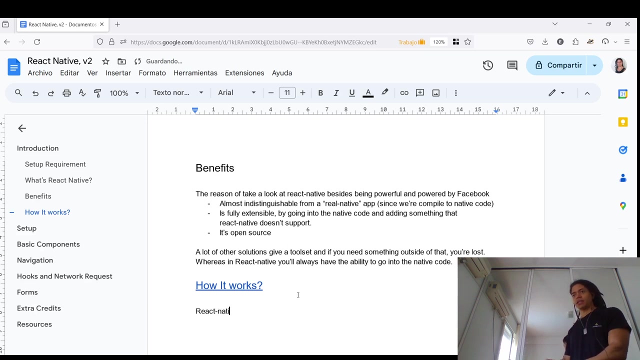 saying it is, it is open source. okay, so how does it work? react? react native is targeted. the reactionary is built exactly. react native is built. react native is built in such a way, in such a way that that it targets, that it targets the existing compiler, and that is java or kotlin or the ios. 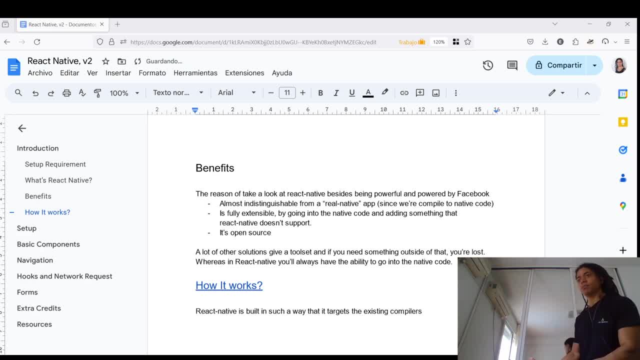 standard android compiler, standard ios compiler, standard platform compiler platform artifact, mm-hmm. so there are compilers that um accept java or kotlin and target the android platform, and there are compilers that um accept objective to your script and target the iris platform. and this is exactly what react means. and the reason this is powerful is because 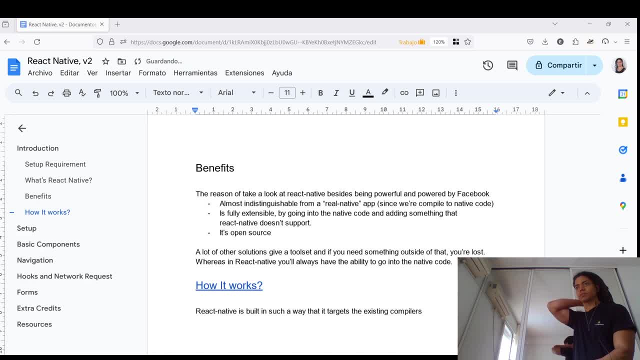 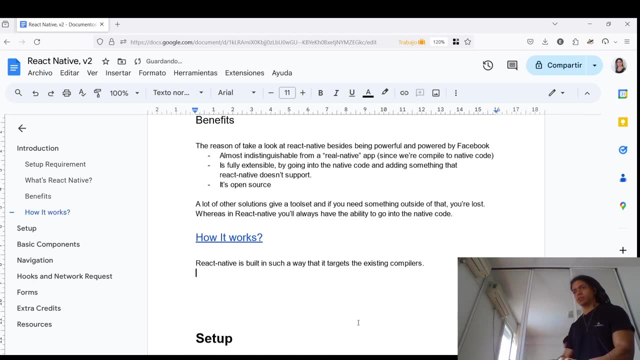 these compilers are already built to android and it also makes react native very expensive existing compilers. so react native is built in such a way that it targets the existing compiler. so android has have it is. it says: android has its own compiler. that receive that, receive that we. 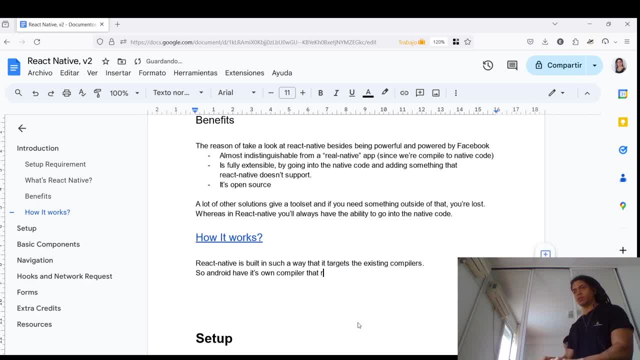 re see: receive java or kotlin. okay, so android has its own compiler. how, the notion of compiler is something that has ship, that has shaped the today's world. so android, so the platform. android, so the platform. okay, has its own compiler, trans translator that receive java or kotlin. 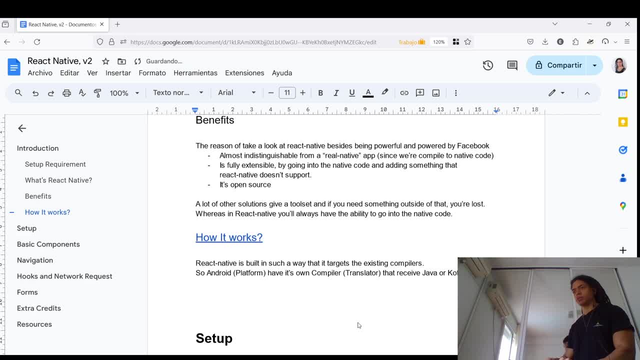 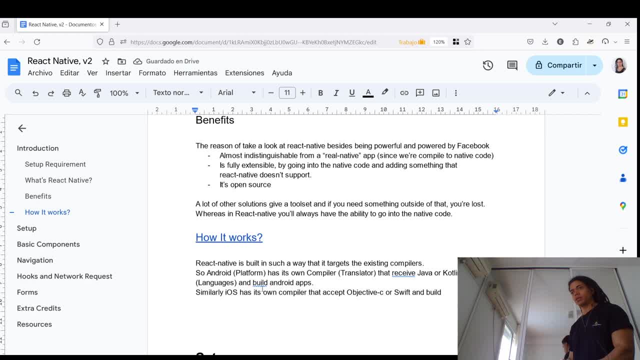 in, build in, build in exactly in, build Android and build iOS apps, but the idea here is to recognize that concept and anything you are trying to run something. remember those fundamentals and how powerful is how this several concepts, the platform, the translator or the compiler, interpreter and the language- has shaped. 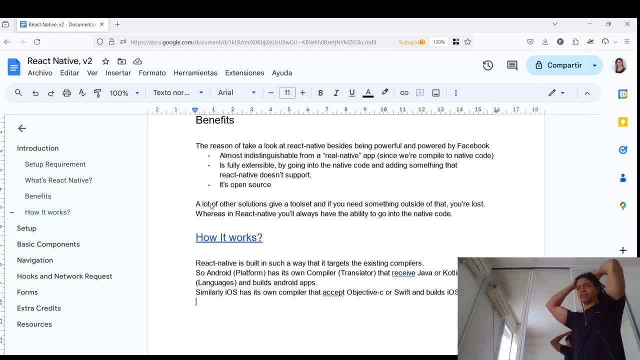 our reality so vastly that you're not able to see what I'm doing here, recording here, right, because there is a platform that allow is to actually capture all this video and then translate into that can be translate to something, whether it is in a compiler or not, transmit over the internet using a language in a 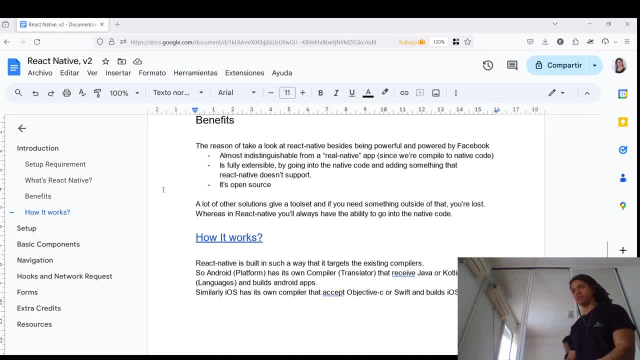 protocol for that. so that's something very, very interesting, thank you. you can have standard platform compilers, so so you can have. so you can have a React native. React Native Windows. react native- yeah, react native windows- m-t Shop ПомН disposal, M-T Shop Пом��. Réact Native Windowsant doe domt. Ok, so you can have. so you can have. so you can have a React native Windows. react Native Windows. react latency ability. more expensive windows: abajo gaddenато ab aumentarumm. não é parceiraığımıztych судум. agora você pode ter Game over cloud. let's get work done with web. вами é Rà que você consegue Orthodoxлав residir na opção do PC Cardanado. estou ceceando-se de reax nativos展望 para o resgate: V horas 70 tones. bem, bem, é bom boarding the Monday. chill está sempre bem e. 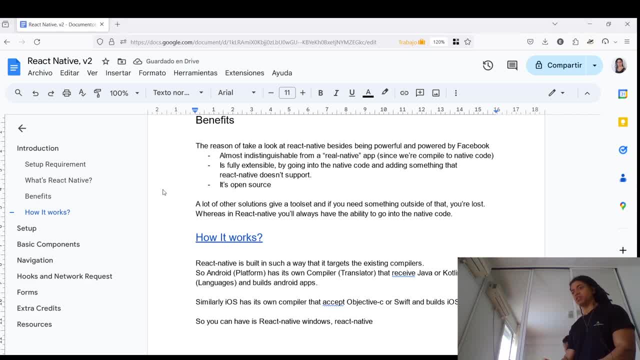 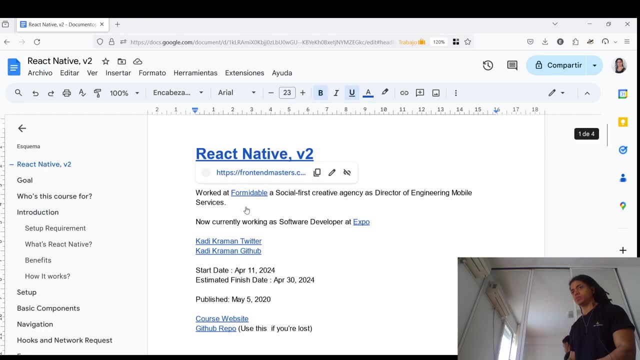 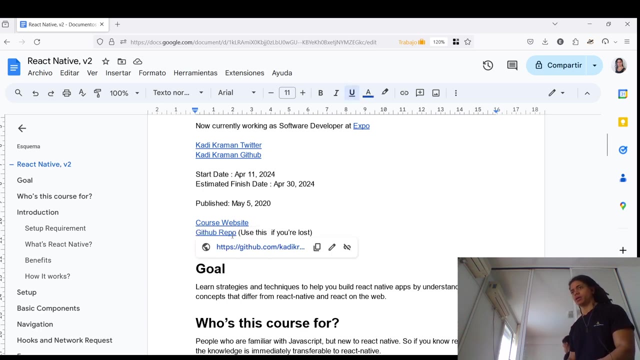 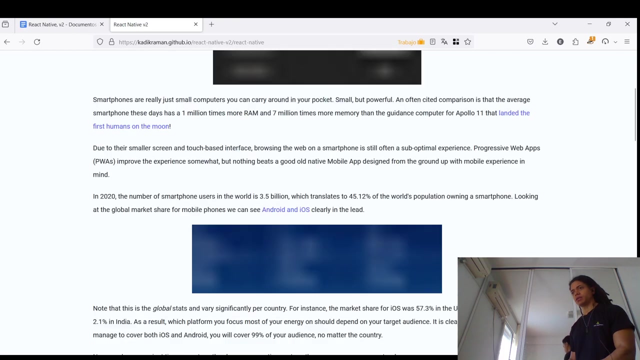 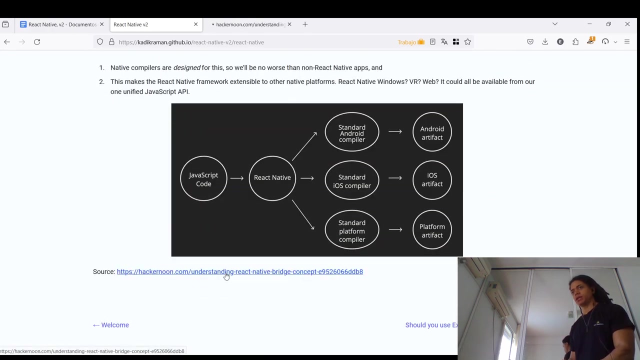 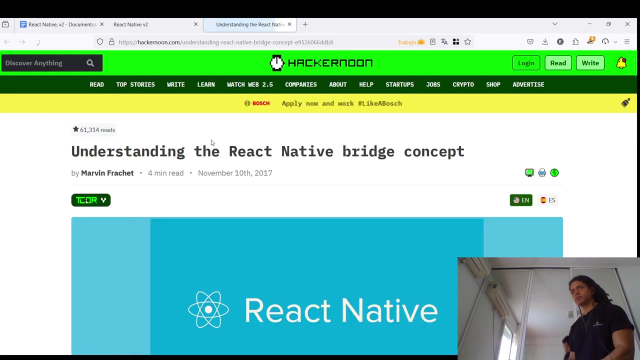 yeah, we have native window, we have native VR. so that's why, why? why, interestingly, yeah, totally, totally- you have repo courses website, whether, as is this: yep, there you go about you exactly, and now we're looking at this right. think around defending react. native bridge council. okay. 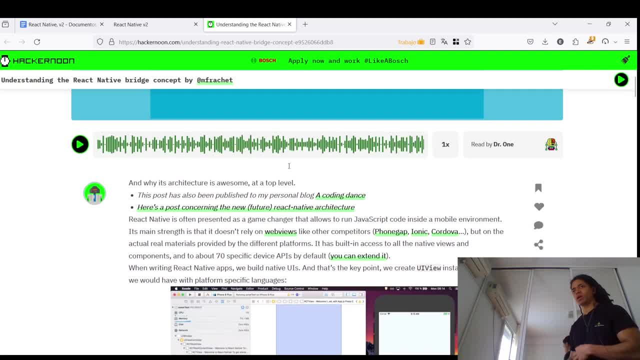 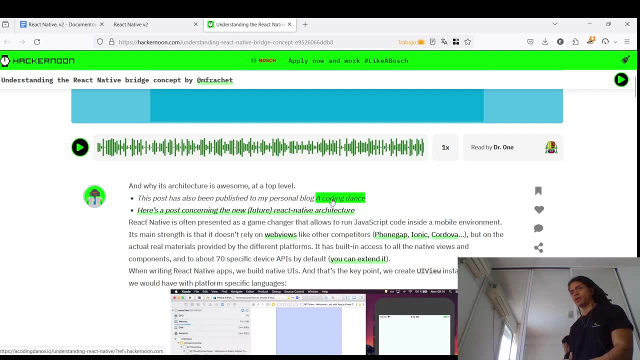 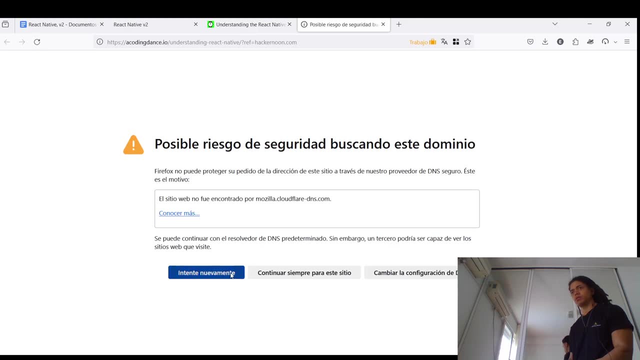 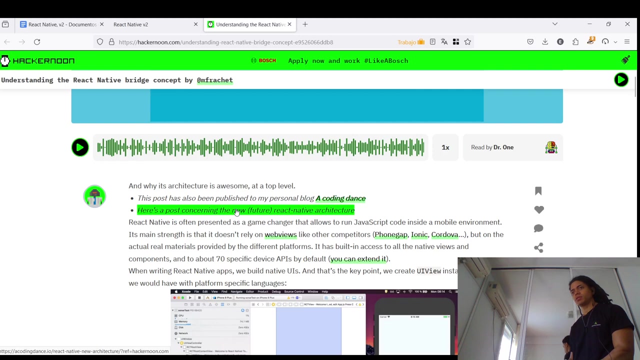 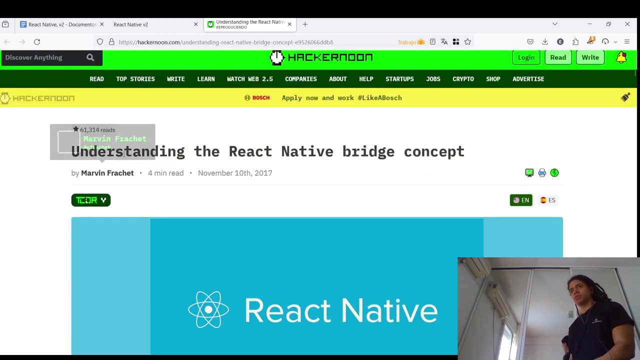 exactly. if you want to have a more dive deep into this, my coding- then yeah, don't you have that? no, hmm, number one actually doesn't say: okay, find your partner in code and work like a Bosch by clicking the logo below, understanding the react native bridge concept by Marvin Pratchett and why its architecture is awesome at a top level. 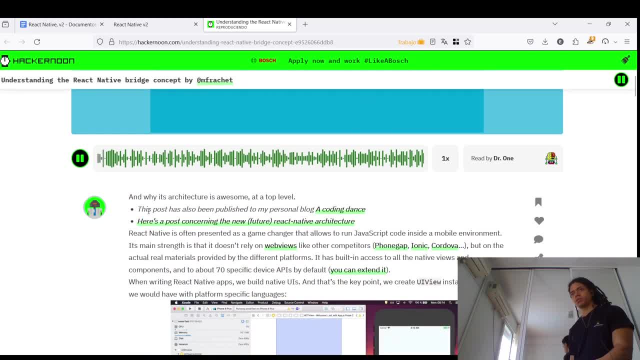 this post has also been published to my personal blog, a coding dance. here's a link to the blog post in the description of this video, if you want to check it out. here's a post concerning the new future. react me okay. that's interesting how they add this particular technology as a way to read text using. 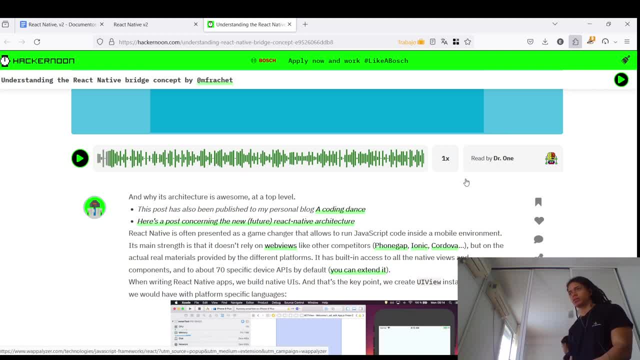 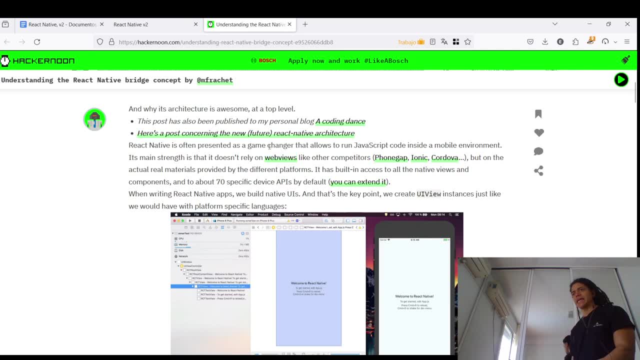 its version and I can see it's quite mechanical, this voice, but it actually do this work. react native is often preserved as a game changer that allow you to run just with code inside a mobile environment. it is mainstreamed and then you can use it to run your experts or learning. you can also use this and 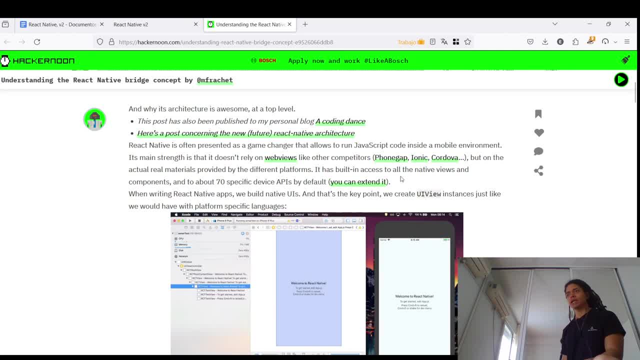 then you can use it to run a operating system or a computer and you can even just run a 것이 in, basically the D. you can go through the various versions, but it's that it doesn't rely on what you like. other competitors: PhoneGap, IONIQ and. 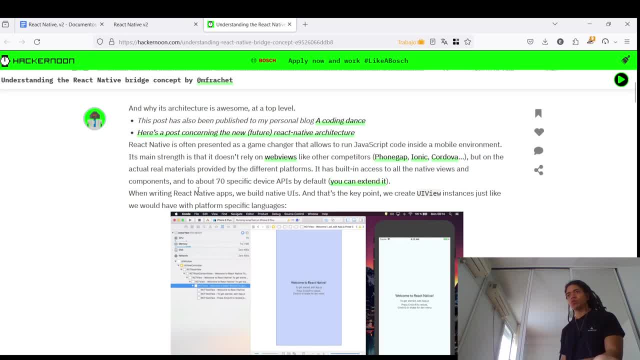 Cordoba, but on the actual, real material provided by different platform. it has building access to all the native view and component and to about seventy, but seventy with sixty specific device API. by default. you can extend when writing react: writing react. okay, so you are now exposed to 70 specific device api. 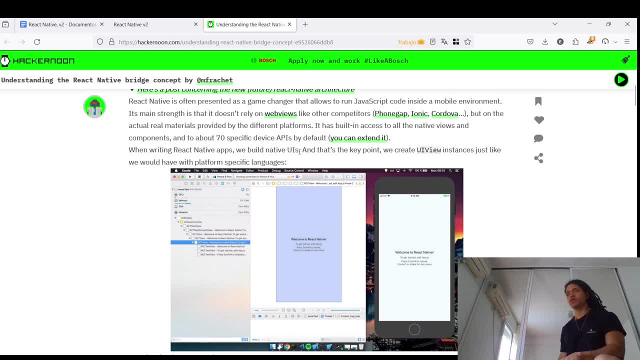 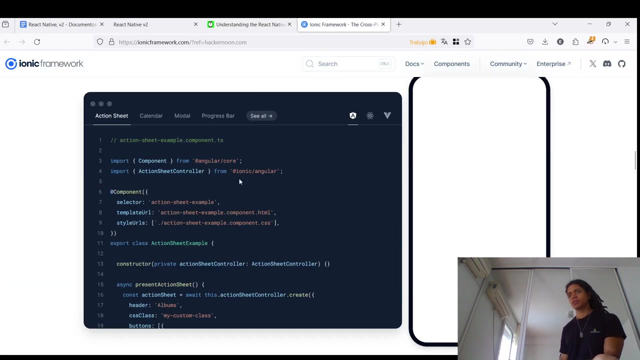 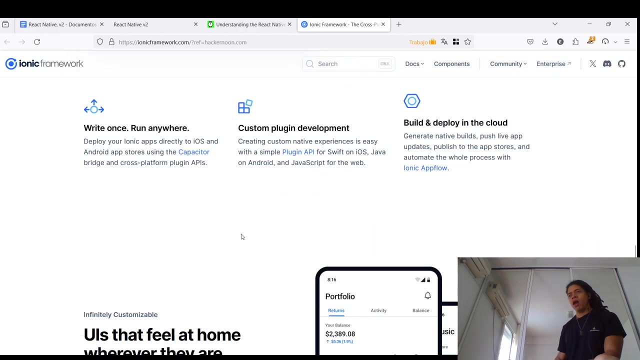 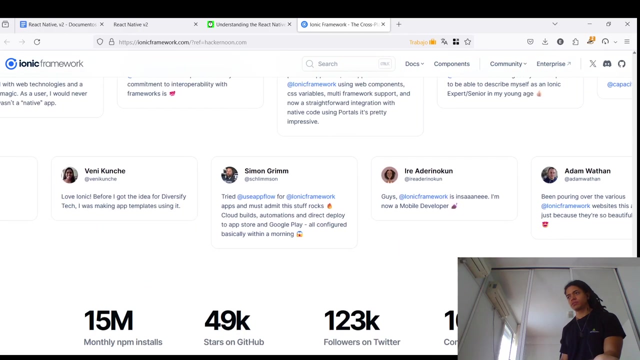 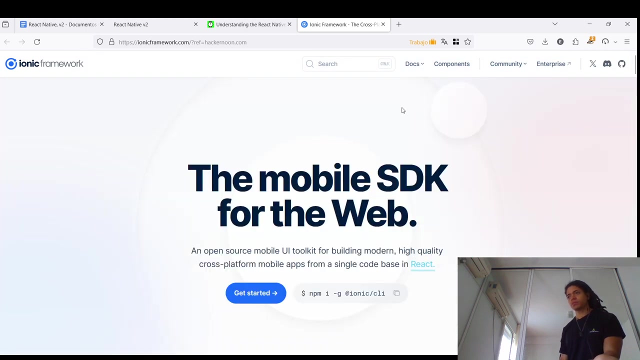 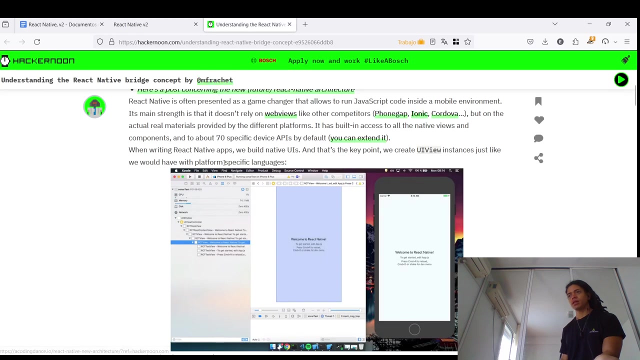 when writing react native apps. we build native ui and that's a key point. we build native ui, we don't use webview for that. are you already in cordova? um, yeah, i'm quite familiar with this and definitely quite familiar to this. uh, but, and that's the key point, we create ui view instance, just like we will have with platform. 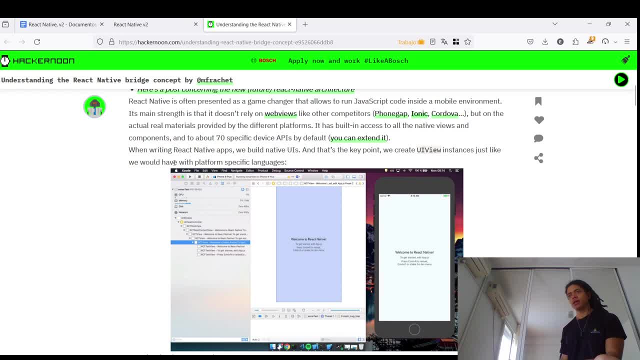 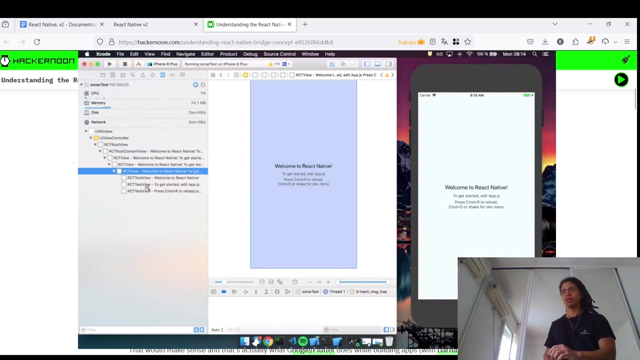 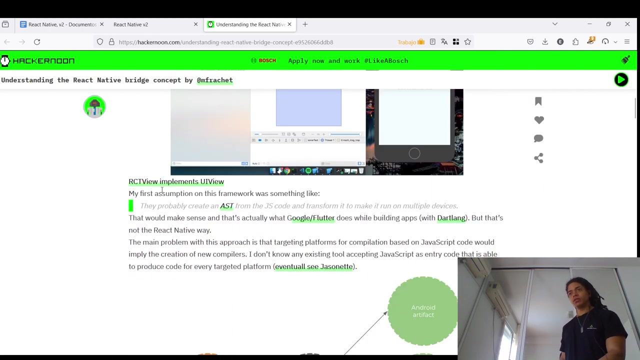 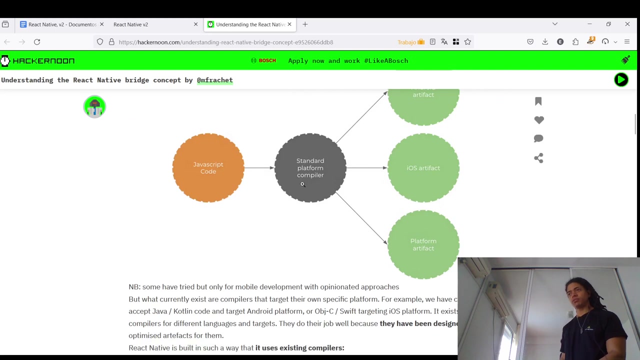 specific language. interesting, okay, so you are not okay. so you are not okay. so you are not okay. okay, we create ui view instance, just like we will have with platform specific language. interesting, so you are now closer to that. all right, rtc view implementation. implement ui view. so this actually is where it comes to that standard platform compiler. 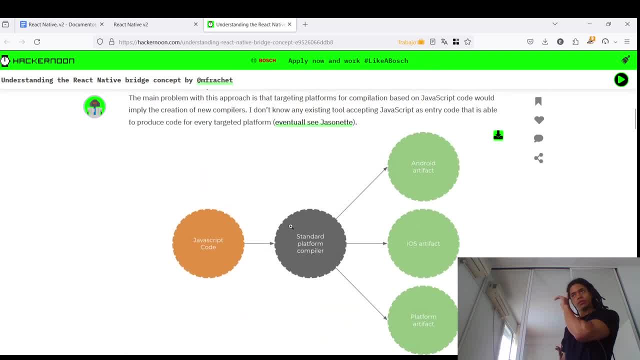 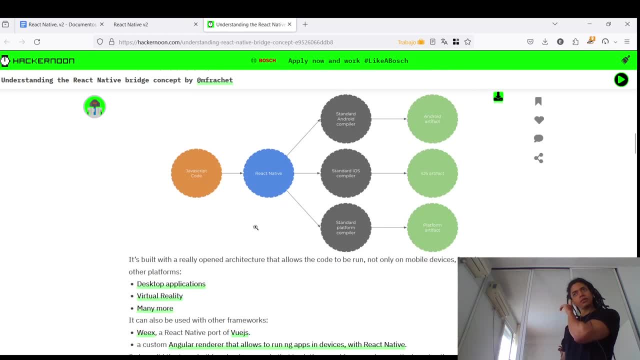 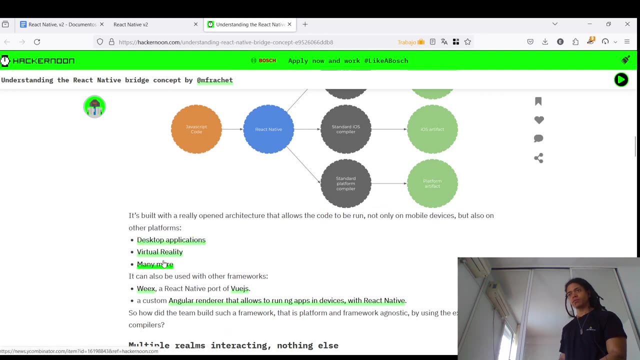 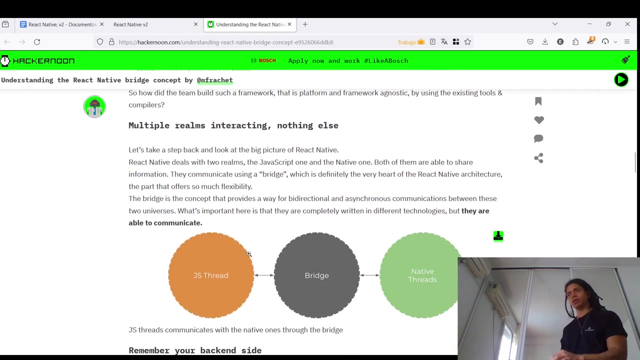 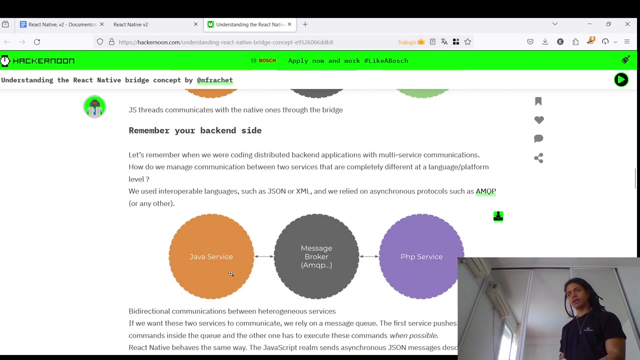 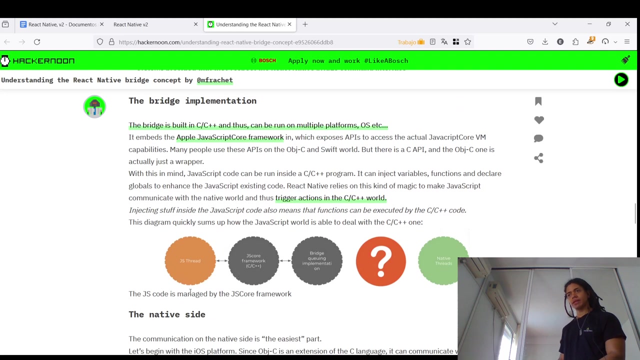 or in the case, exactly in the case- of this standard platform compiler, that create artifact from each one of them. but the thing here is that multiple rounds interacting nothing, nothing else. remember your back inside the bridge: implementation- okay. now this is explaining is how all of this is okay. the architecture behind the scene. 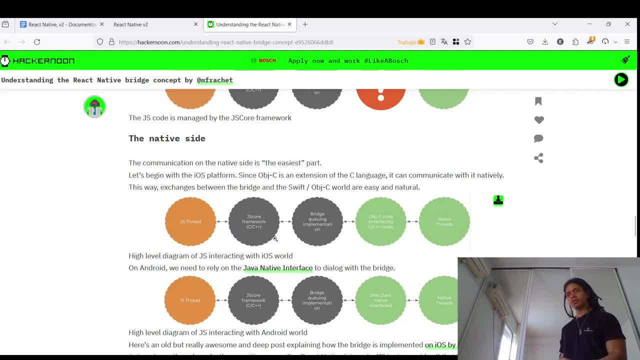 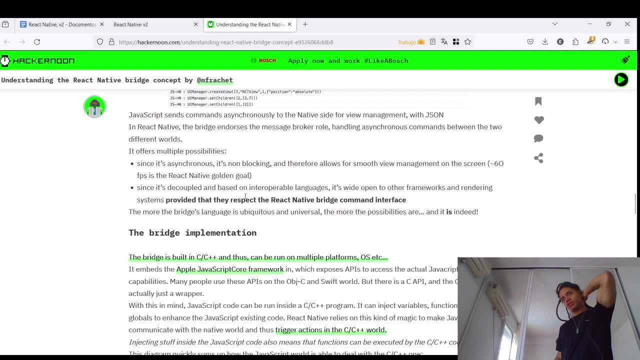 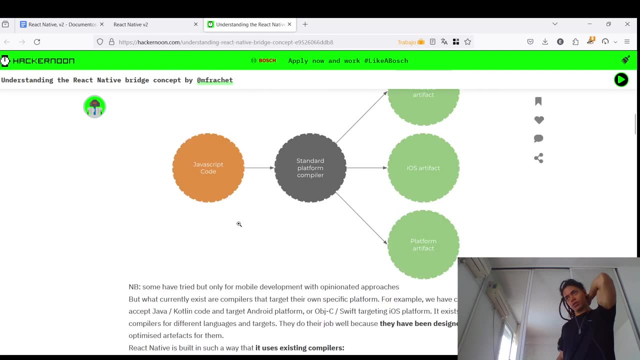 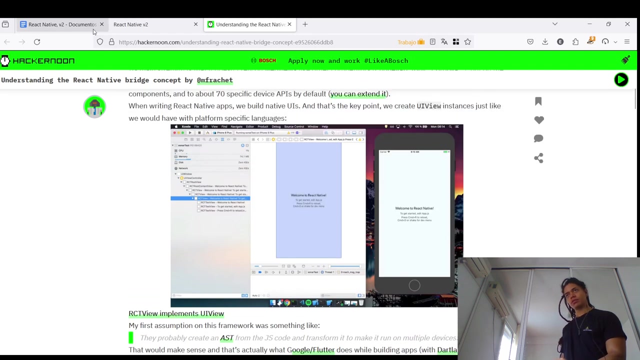 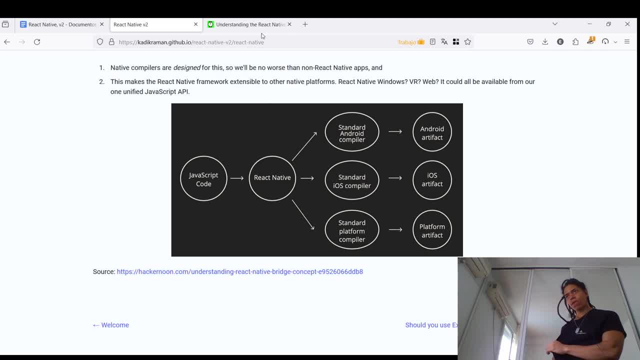 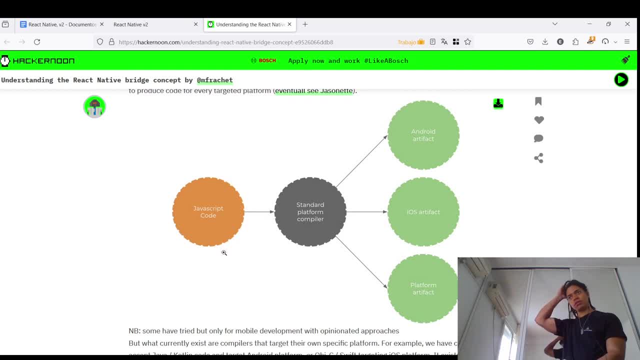 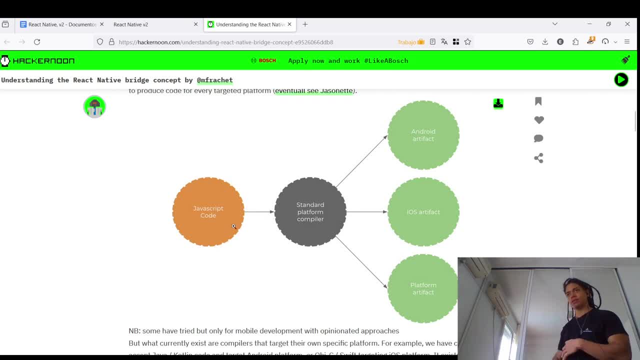 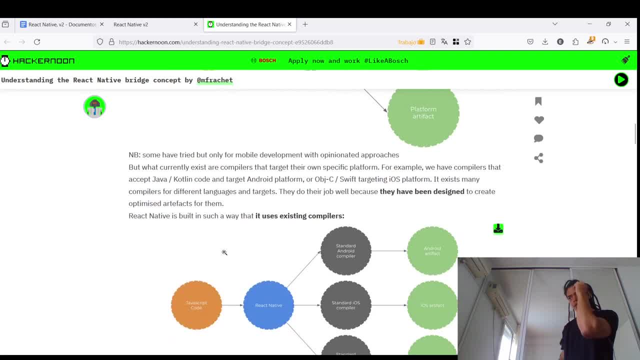 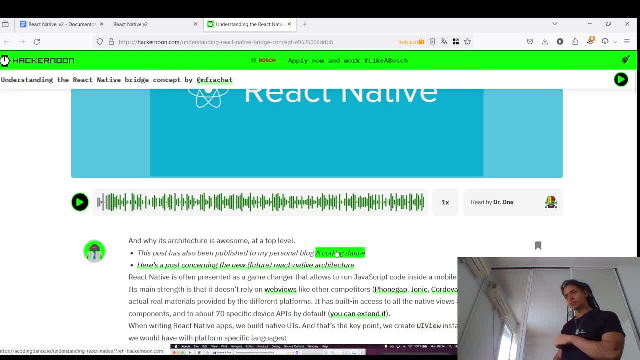 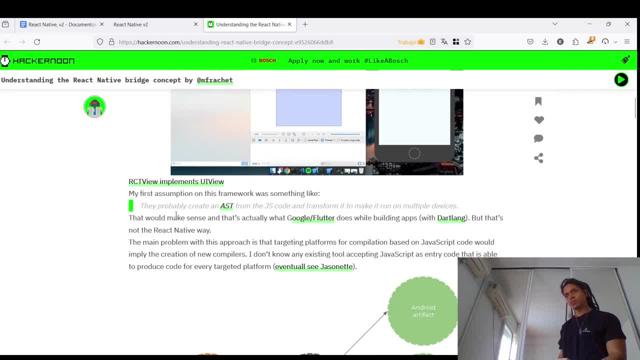 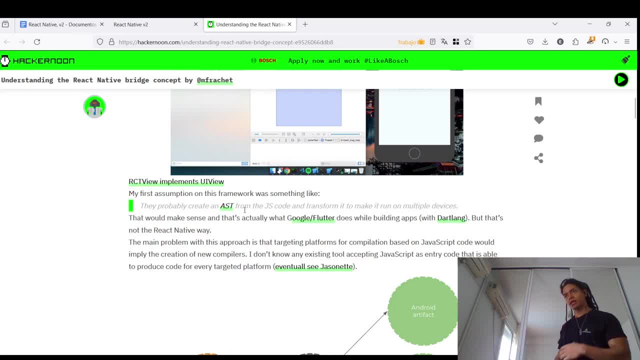 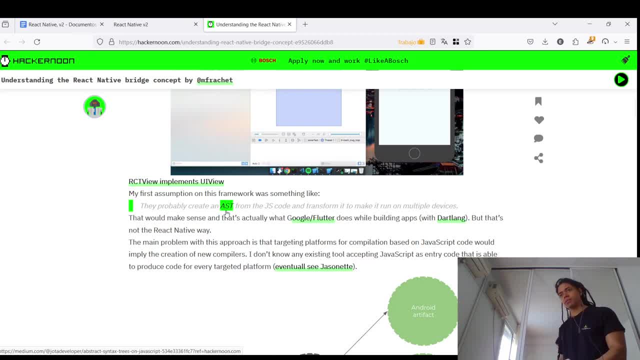 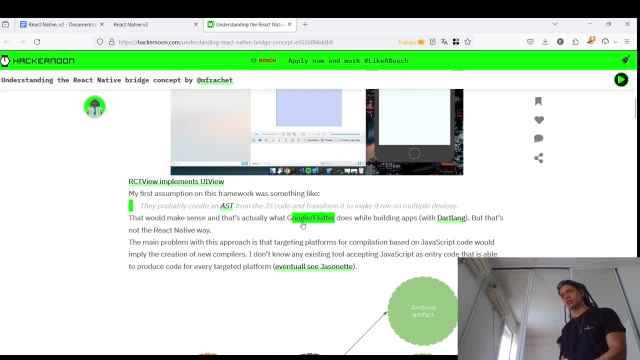 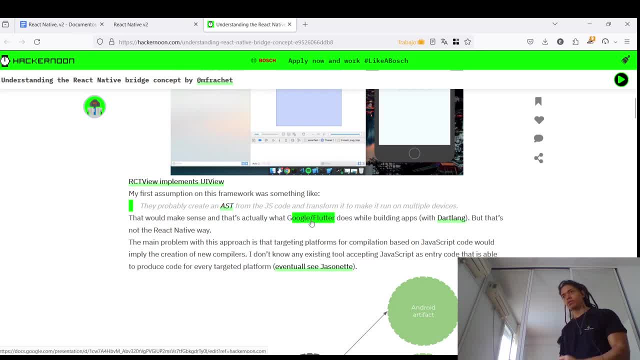 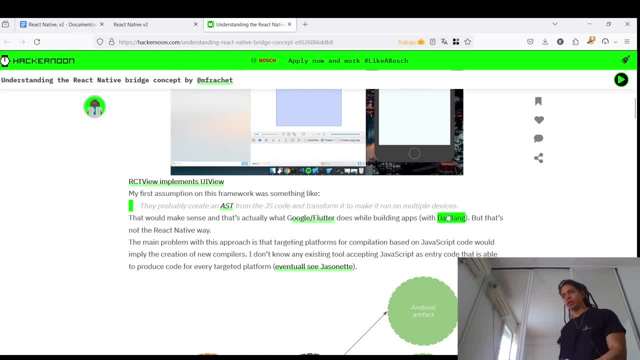 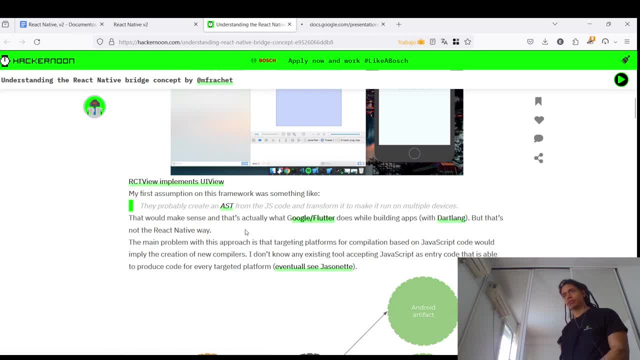 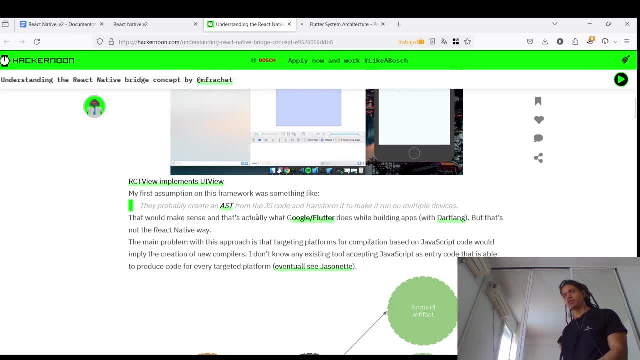 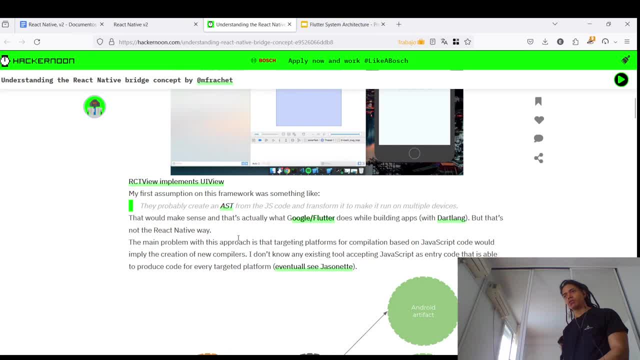 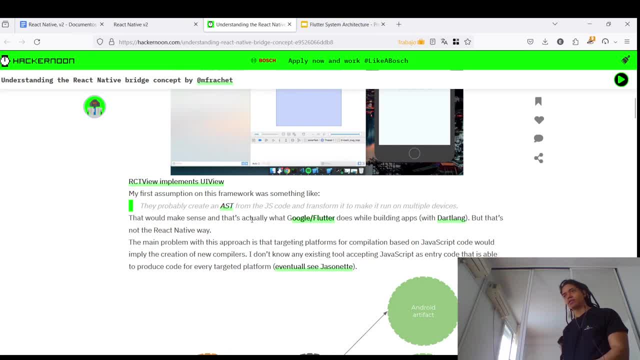 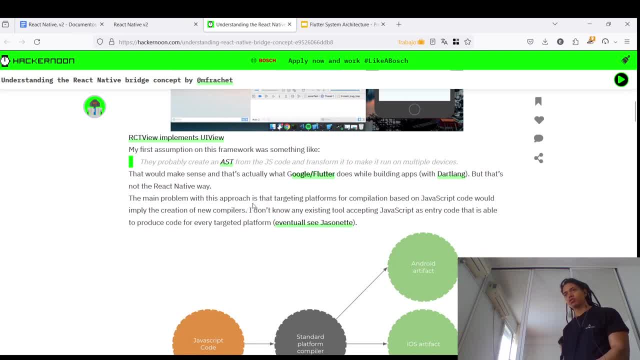 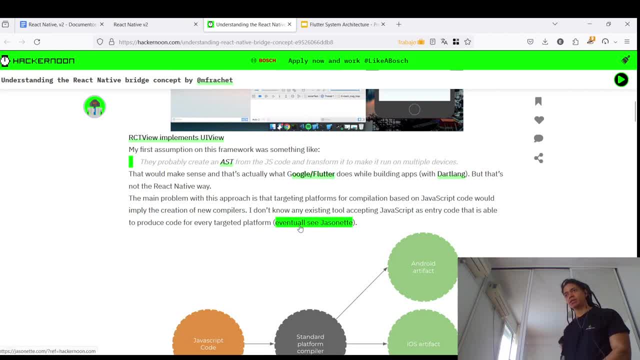 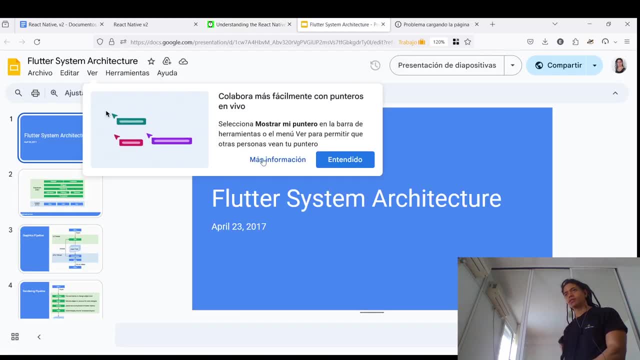 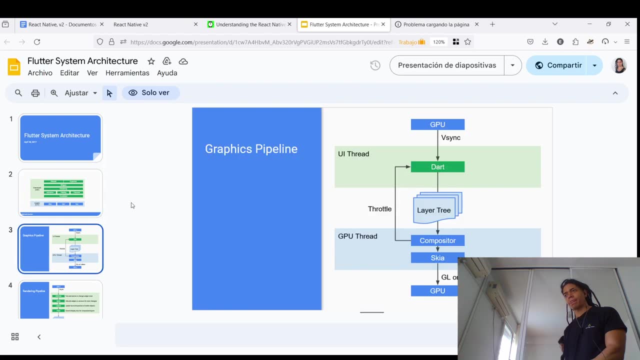 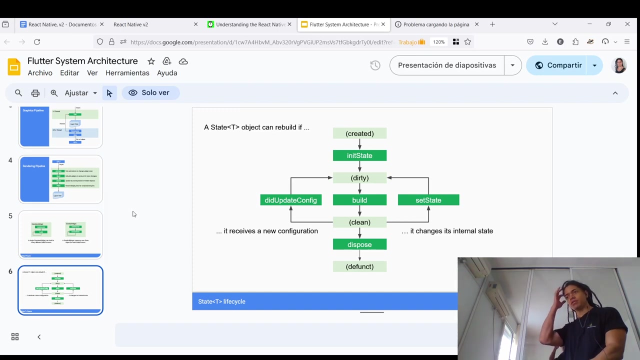 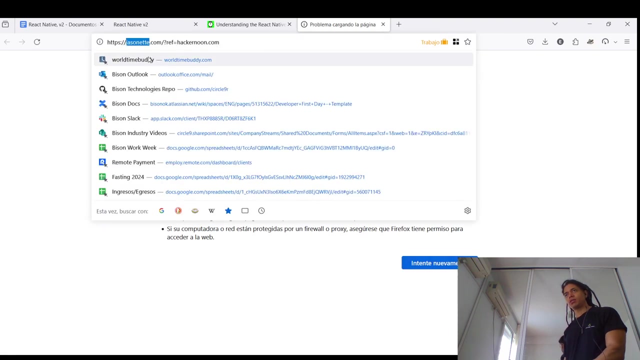 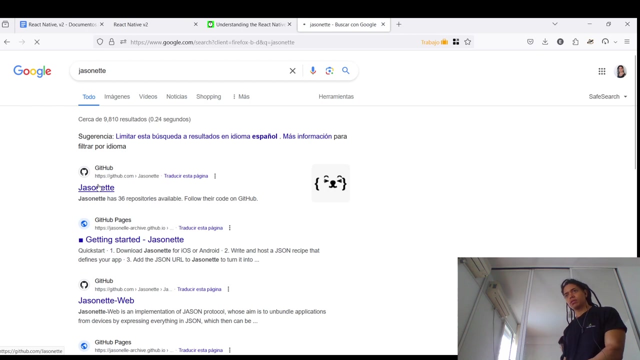 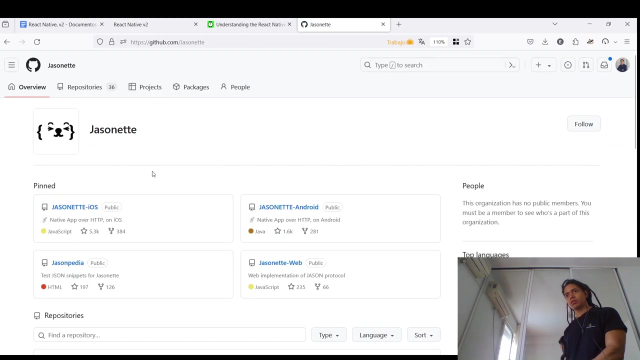 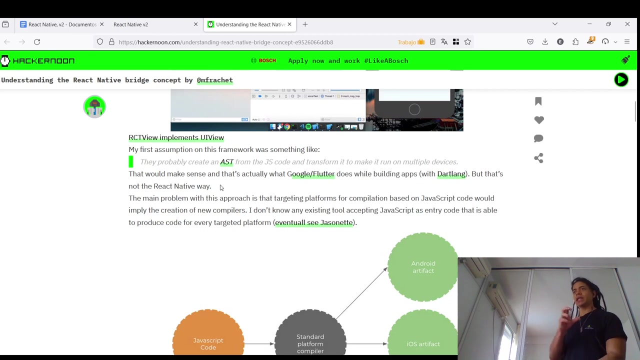 she briefly explained about that and i think it's quite important, as you understand what are all of these themes is behaving behind the scenes eventually, see, just on it. oh, this is describing it. the Florida architecture- interesting. okay, exactly, but so the? so the main point of creating is an abscess, is 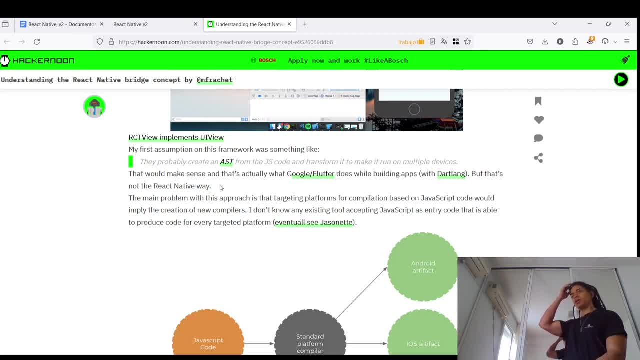 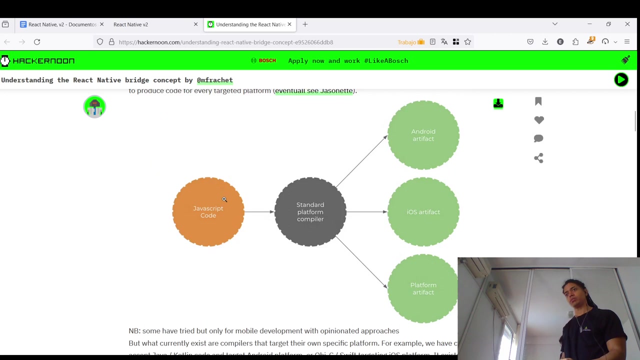 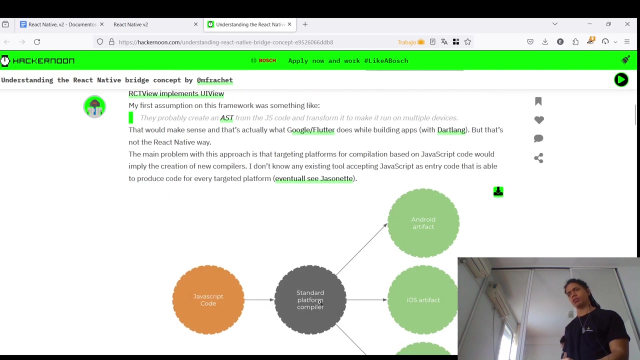 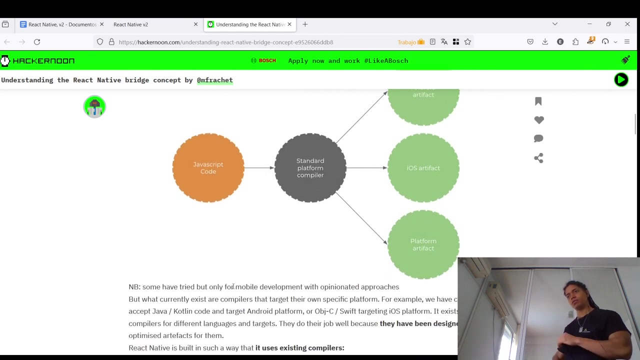 abstract syntax tree from the Yes. go and reform and reform it to make it run on multiple devices. a. so, for example, Google employer does this. so they say, okay, we have now multiple a compiler. okay, we have multiple compilers for each specific stand up okay. okay, maybe some have tried, but only for mobile development with 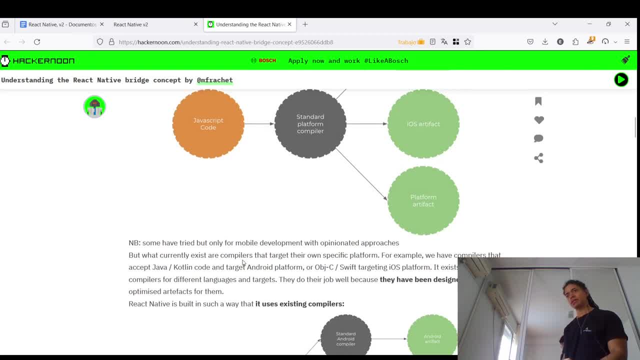 open airing approach, but what's what currently exist are compilers that target their own specific platform. for example, we have compilers that accept gallon Coving go and target Android license for object C and Swift targeting iOS platform. it exists many compilers for different language and talking language. for example, we have a compiler that accepts Jalan codename code and targets Android platform for objects seeing swift targeting iOS platform. it exists many compilers for different language and 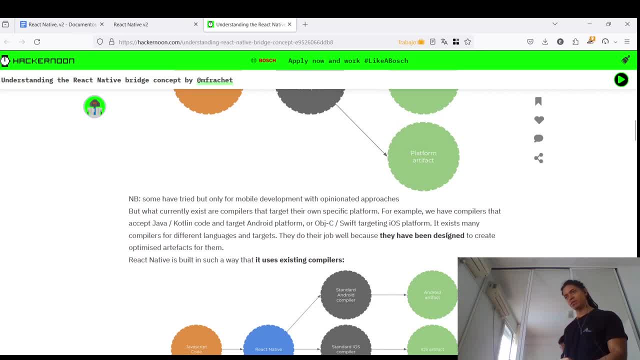 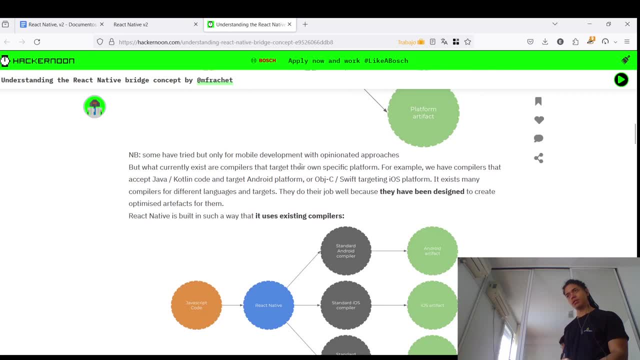 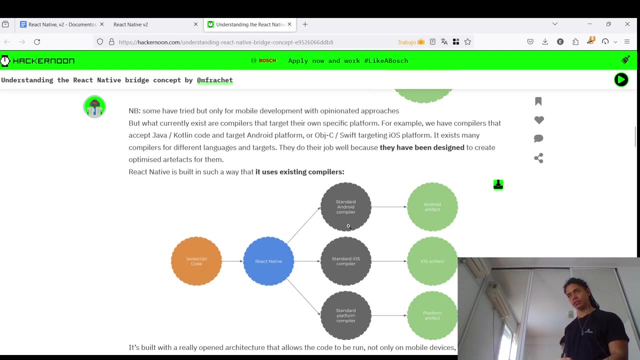 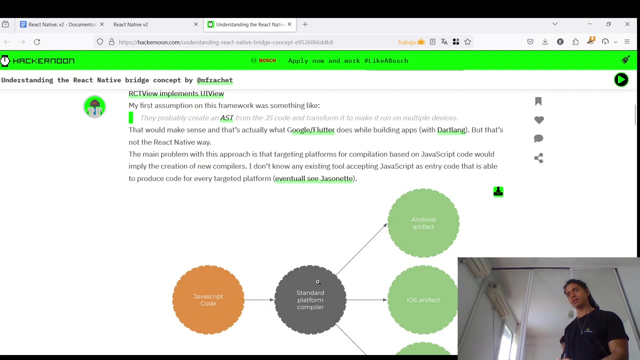 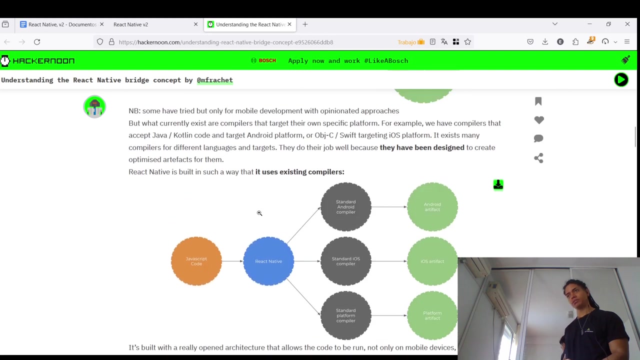 targets. they do their job well because they have been designed to create optimized artifacts for them. exactly so react native is used in such a way that it use existing compilers, so it doesn't create its own compiler. okay, okay, so it will use existing compiler, so it is built with a really 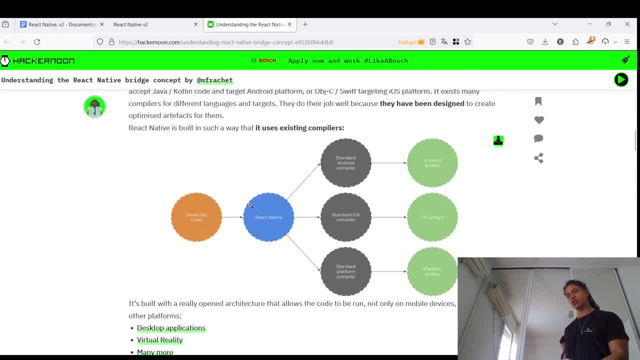 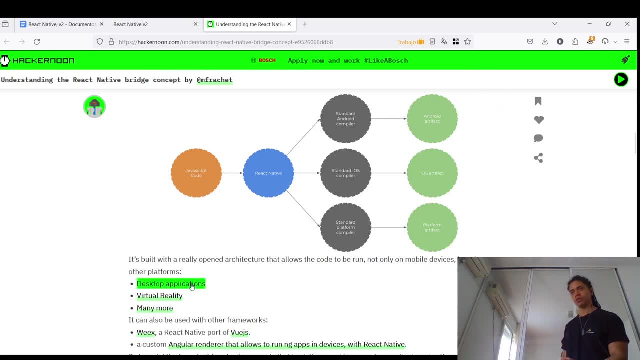 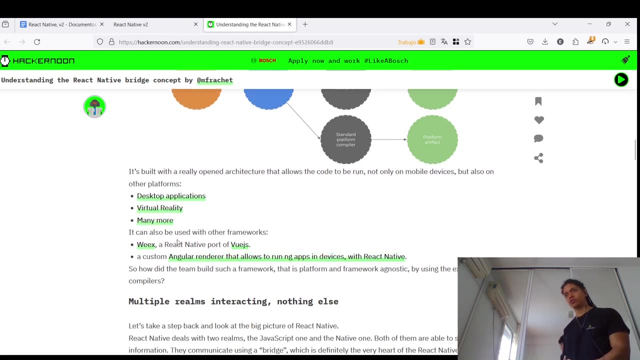 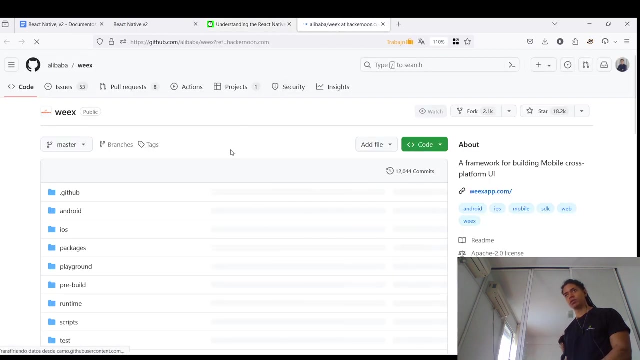 open architecture that allows to code to be run not only on mobile devices, but also an other platform. exactly that's the publication. that's an application, virtual reality and many more. you can also use it in a virtual reality, also be used with other framework. weeks- a react native for of you. weeks in. 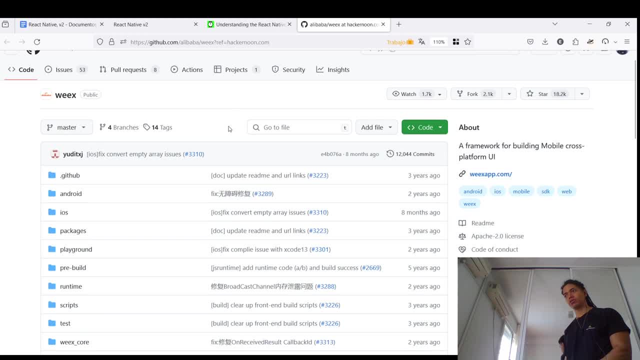 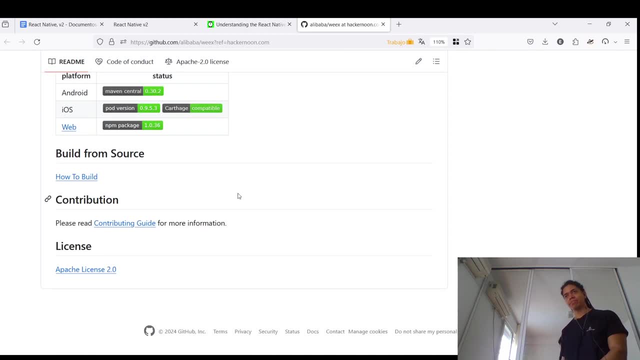 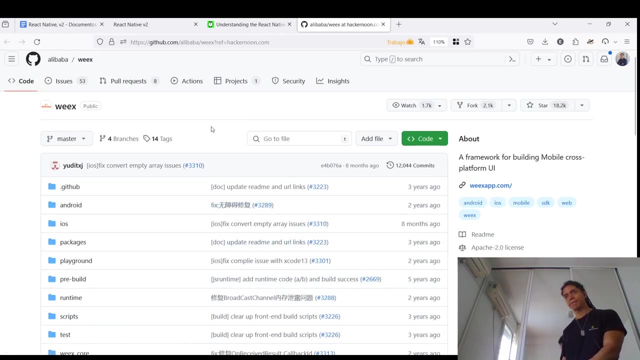 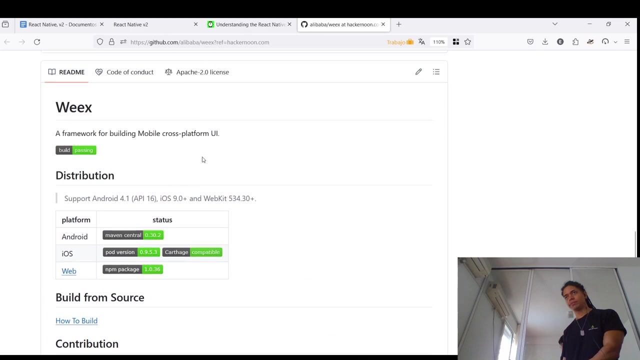 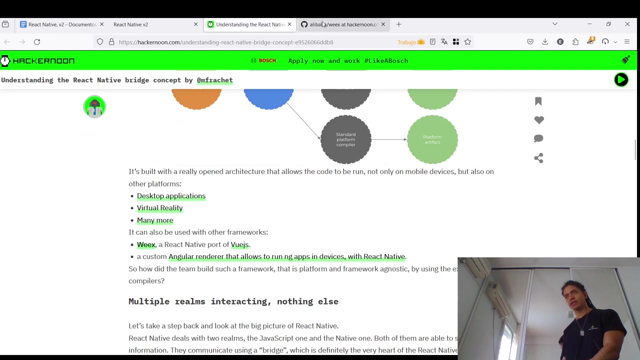 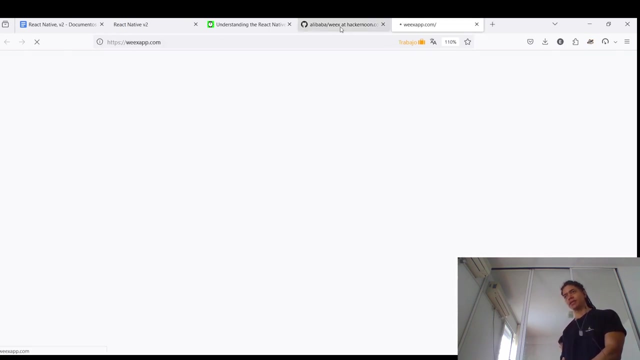 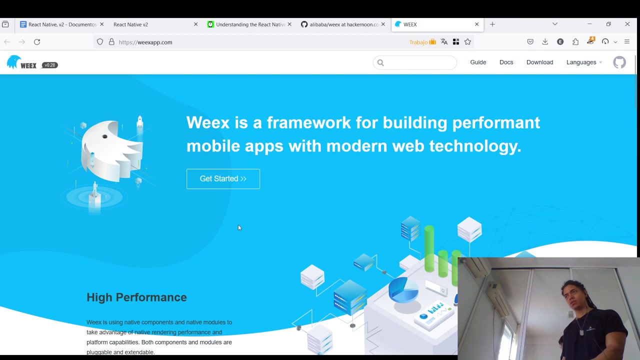 Alibaba a framework for building mobile cross-platform UI. hmm, and we have maybe four of you. yes, Alibaba interesting. yeah, those company actually are building. I can see weeks is a framework for moving black performing mobile app with modern web technology. yeah, those company actually are building. I can see weeks is a framework for building black performing mobile app with modern web technology. 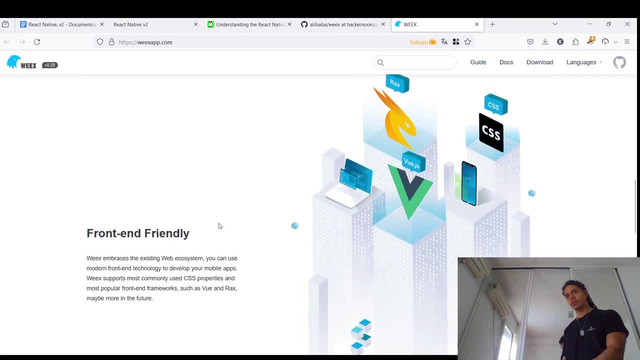 yeah, those company actually are building. I can see weeks is a framework for moving black performing mobile app with modern web technology. from the friendly weeks: embrace the existing web ecosystem. you can use from the friendly weeks. embrace the existing web ecosystem. you can use model from the technology to develop your mobile app we support most commonly. 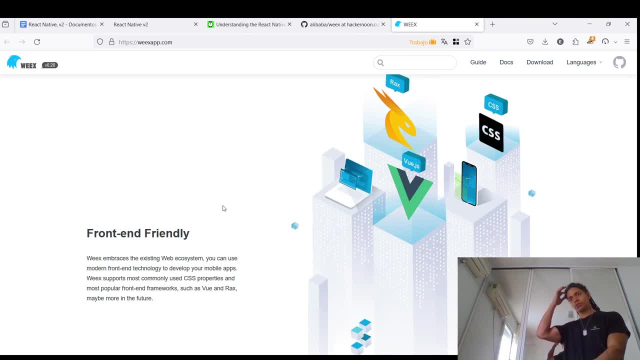 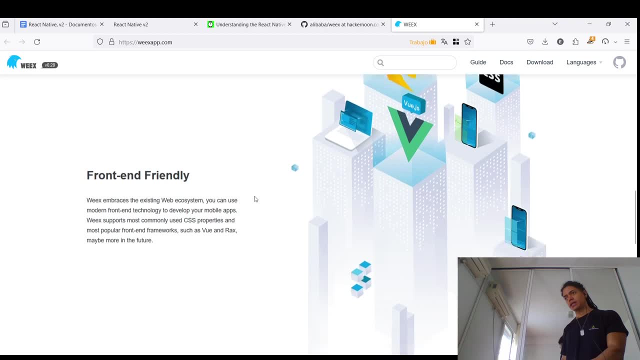 model from the technology to develop your mobile app. we support most commonly use CSS property and most popular from and framework such as you and racks. maybe use CSS property and most popular from and framework such as you and racks. maybe use CSS property and most popular from and framework such as you and racks. maybe more in the future. 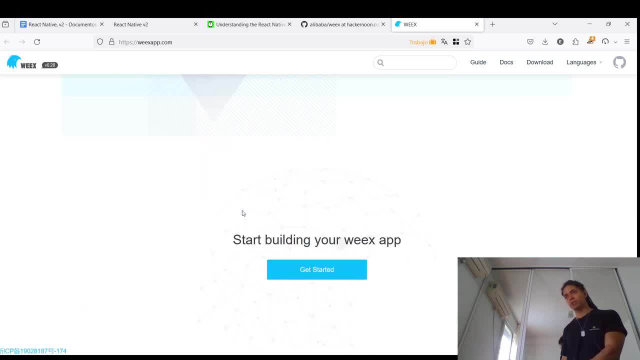 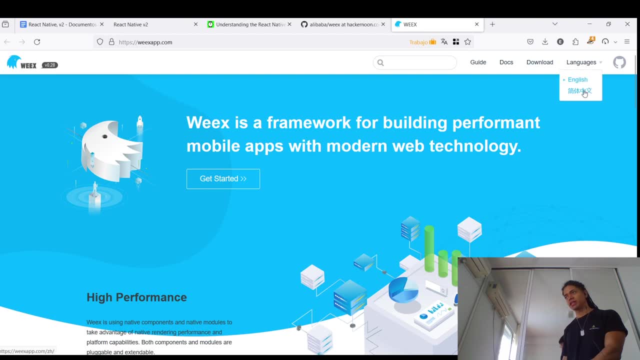 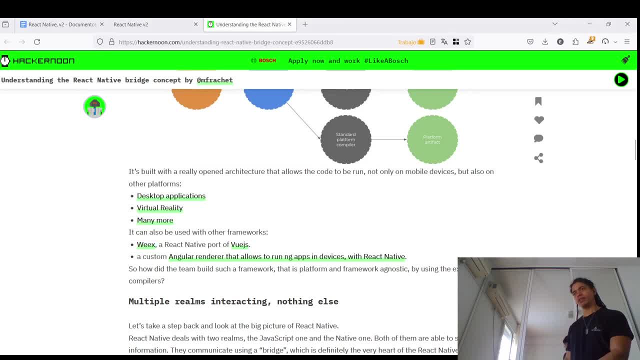 god, oh my god, all right, okay. so yeah god, oh my god, all right, okay. so yeah, this is another okay isn't isn't. is. this is another okay isn't isn't is. this is another okay, isn't isn't is interesting, it's quite interesting. interesting, it's quite interesting. 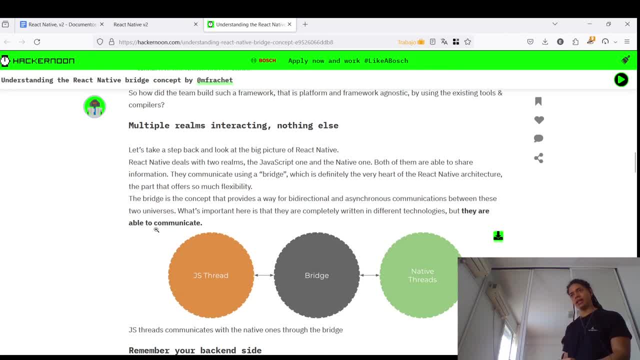 interesting. it's quite interesting. multiple realm interacting nothing else. multiple realm interacting nothing else. multiple realm interacting nothing else. let's take a step back and look at the. let's take a step back and look at the. let's take a step back and look at the big picture of react, native react maybe. 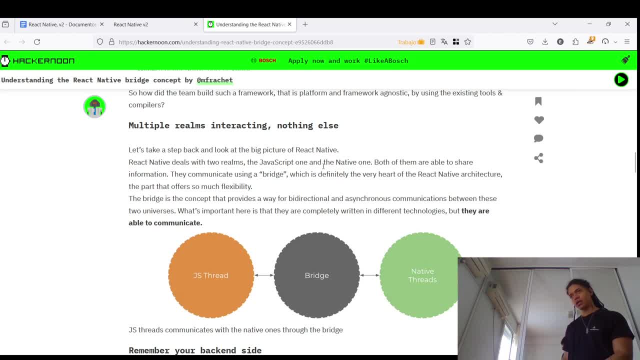 big picture of react- native react. maybe big picture of react- native react. maybe this deals with two realm: the JavaScript. this deals with two realm: the JavaScript. this deals with two realm: the JavaScript one and the native one. both of them are one and the native one. both of them are. 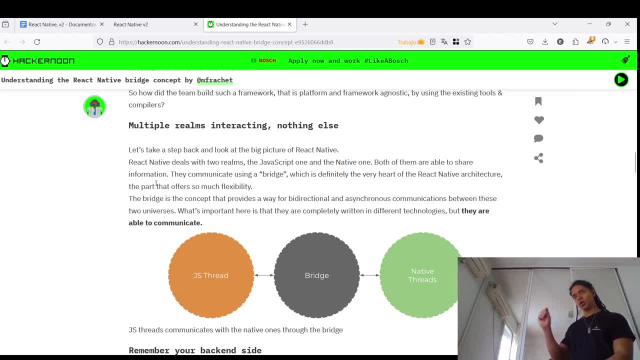 one and the native one. both of them are able to share information because their able to share information, because their able to share information because their particular nature of react. okay as a way. particular nature of react. okay as a way, particular nature of react. okay as a way to look at this, because it communicate. 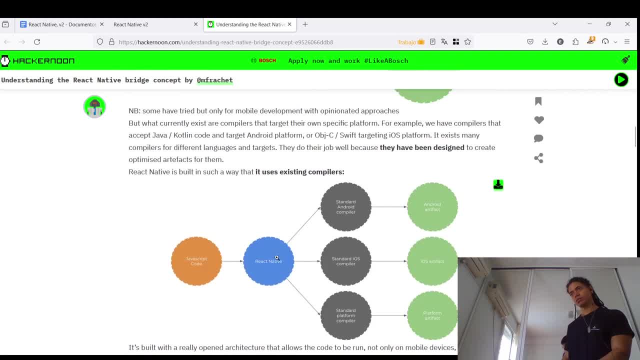 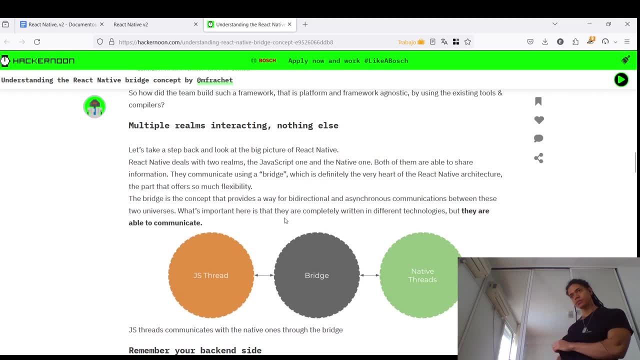 to look at this because it communicate. to look at this because it communicate to their existence. okay, it used existing to their existence. okay, it used existing to their existence. okay, it used existing compiler, compiler, compiler, compiler. okay, it used existing compiler which has. okay, it used existing compiler which has. 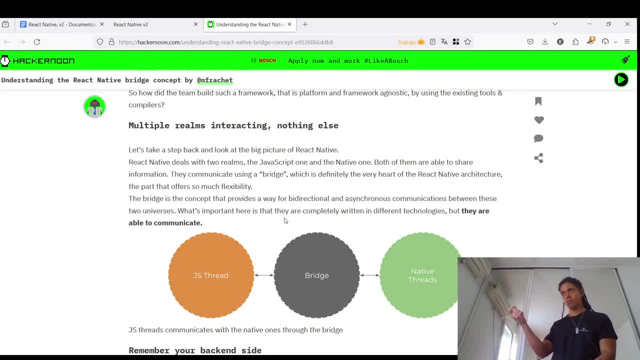 okay, it used existing compiler, which has been show that actually they output been. show that actually they output been show that actually they output. generate is an optimized artifact on that. generate is an optimized artifact on that. generate is an optimized artifact on that platform. an optimal application on. 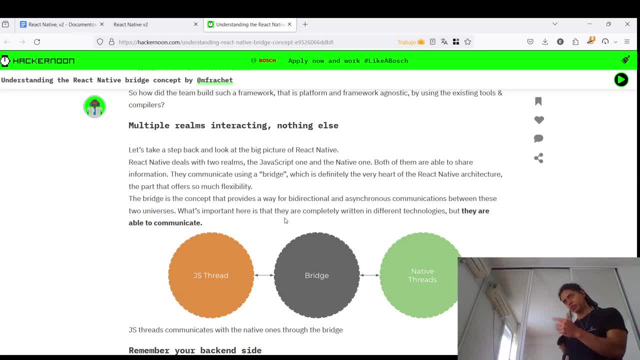 platform, an optimal application on platform, an optimal application on that platform, whether it's an Android on iOS, that platform, whether it's an Android on iOS, that platform, whether it's an Android on iOS. okay, okay, things are starting to make. okay, okay, things are starting to make. 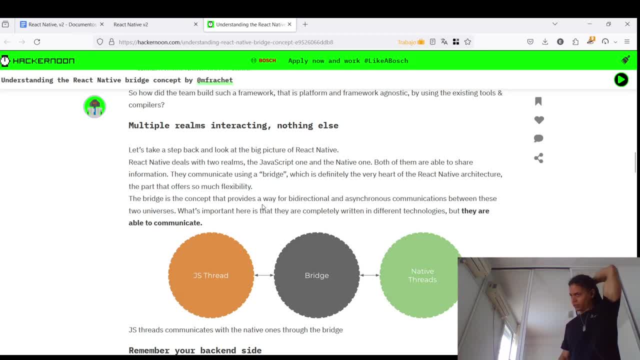 okay, okay, things are starting to make. yeah, things started started to makes a. yeah, things started started to makes a. yeah, things started started to makes a lot of sense, completely complete, lot of sense, completely complete, lot of sense, completely complete. the bridge is the comes. okay, so react. 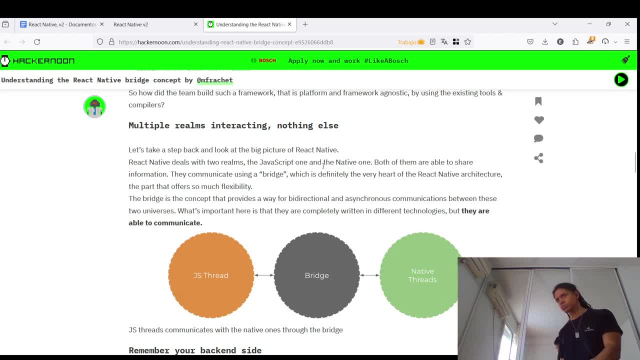 the bridge is the comes okay, so react. the bridge is the comes okay, so react. maybe deal with two realm right. so the maybe deal with two realm right, so the maybe deal with two realm, right so the JavaScript one and the native one, both JavaScript one and the native one, both. 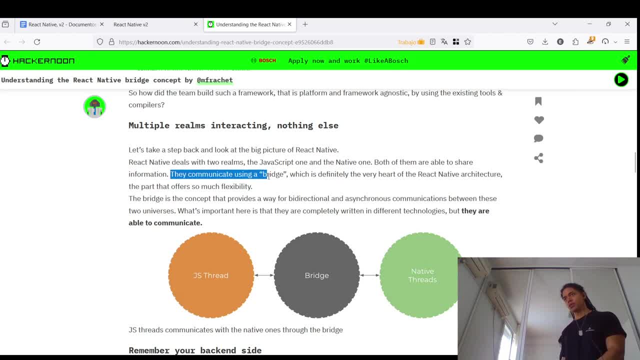 JavaScript one and the native one. both of them are able to share information of them are able to share information of them are able to share information. they communicate using bridge, which is they communicate using bridge, which is they communicate using bridge, which is definitely the very heart of react. 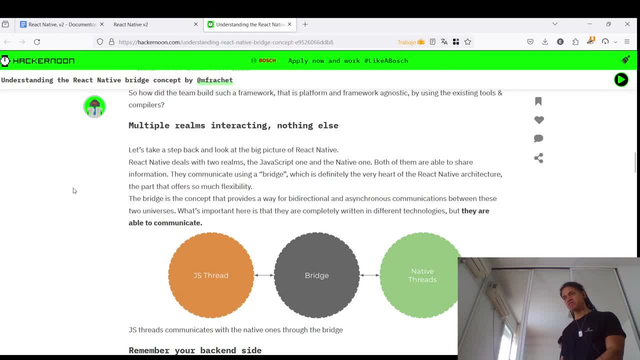 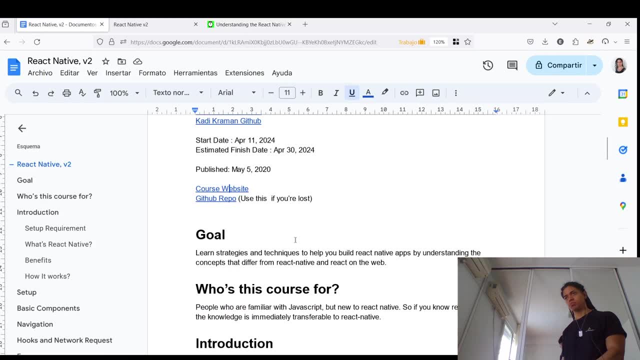 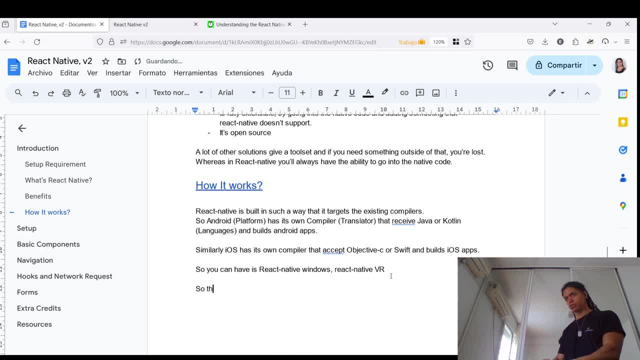 you want to take a look at more of this. you want to take a look at more of this. so the react, so the react native. so the react, so the react native. so the react, so the react native. architecture: okay is by using a bridge. architecture: okay is by using a bridge. 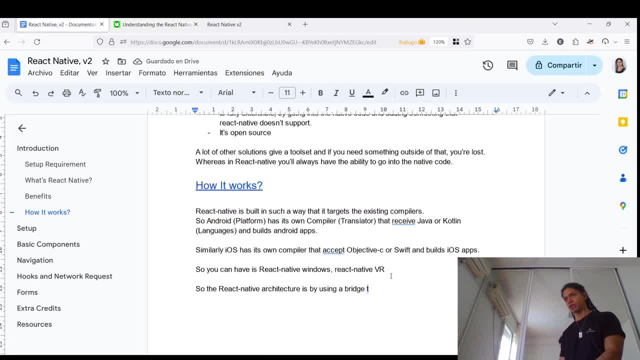 architecture: okay is by using a bridge. is using brick: okay. is using brick- okay. is using brick: okay it's it's. it's using brick- okay, it's using brick. okay. it's using bridge: okay, it's using brick. okay. it's using bridge: okay it's using bridge. okay it's. 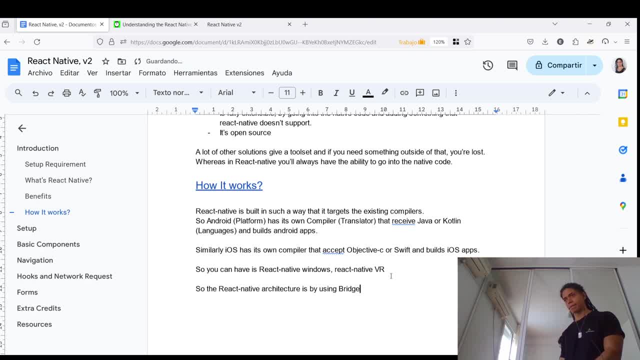 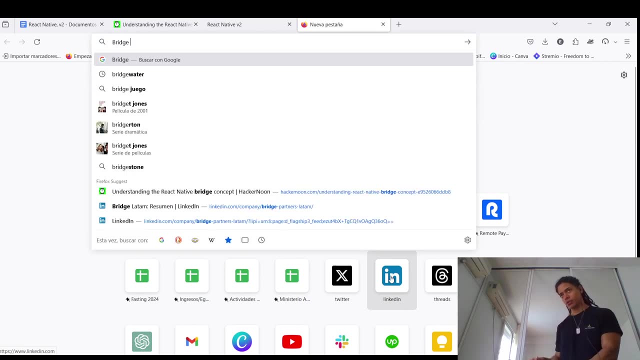 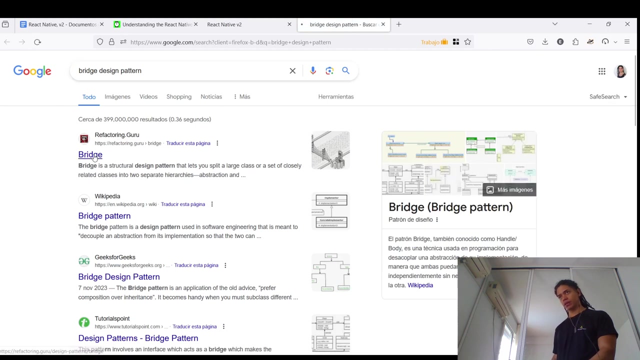 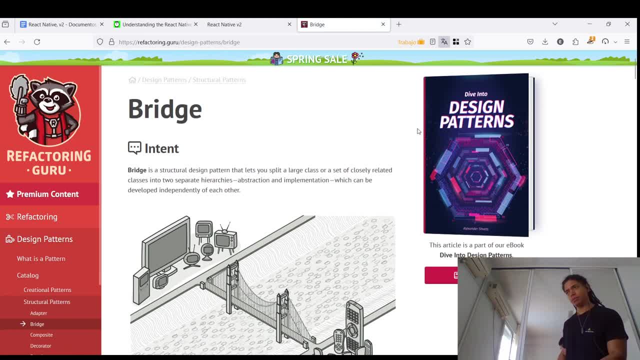 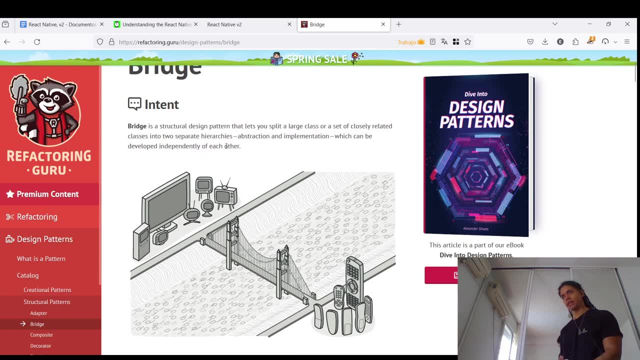 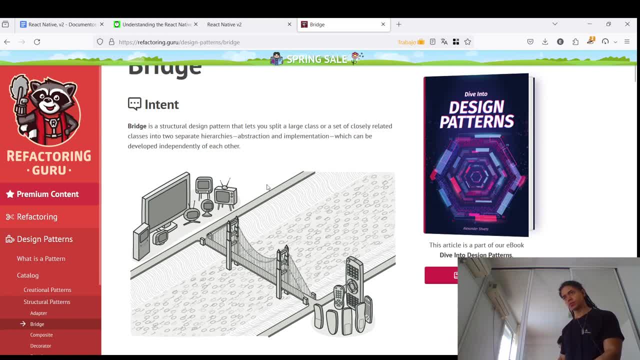 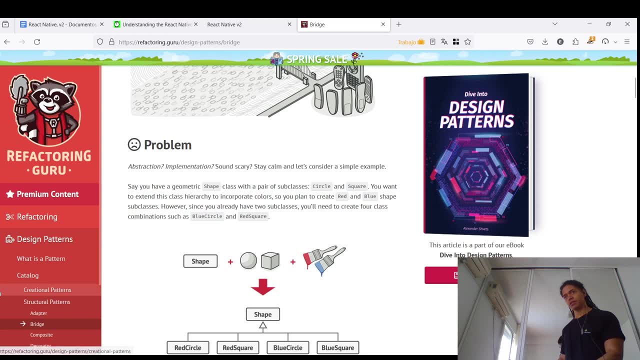 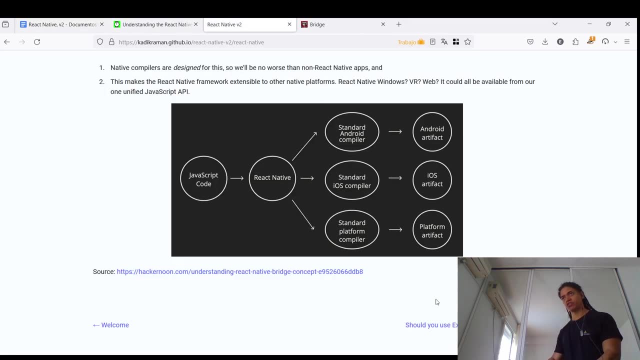 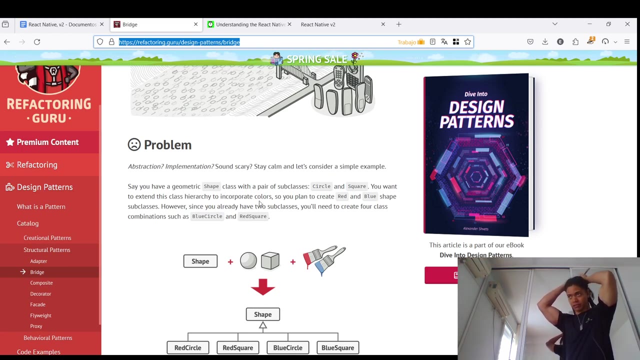 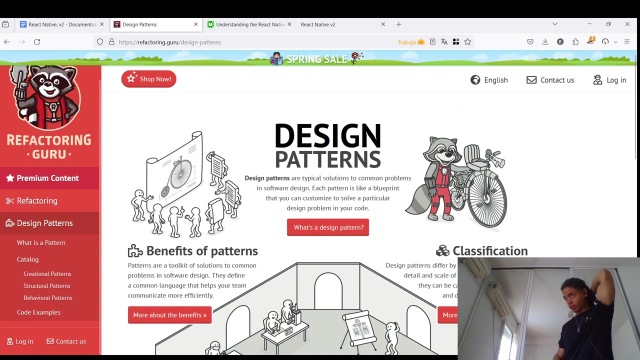 of each other: problem abstraction, implementation, some scary. stay calm, this is part of the structural pattern. mm-hmm. this is part of the structural pattern, part of this pattern. the same patterns, so after all, the same patterns, are just problems that are typically solutions, are exactly our typical solutions to. 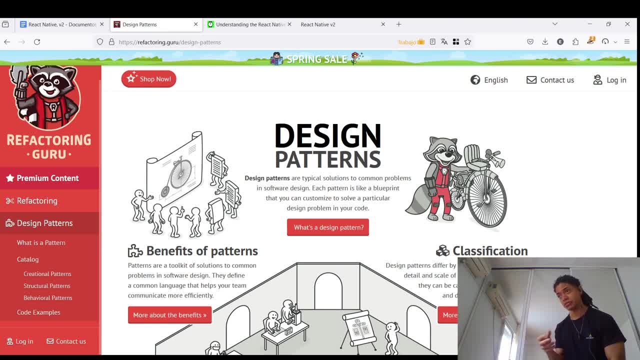 common problems. so this design pattern. for example, anytime you need to brush your teeth, you follow a particular pattern for that. anytime you want to take a shit, you want a piece off, you have, you position yourself, or you position yourself, you get away, or whatever, or whatever gender bandage you want to identify, to piss off into a 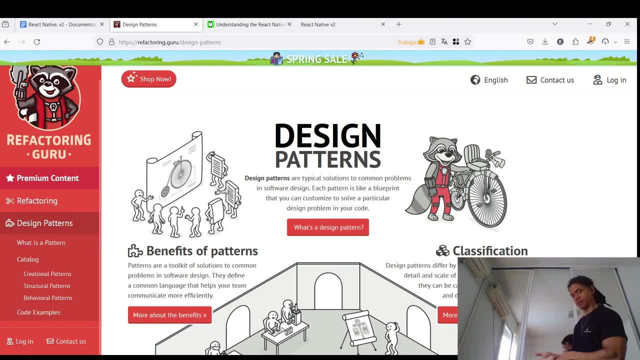 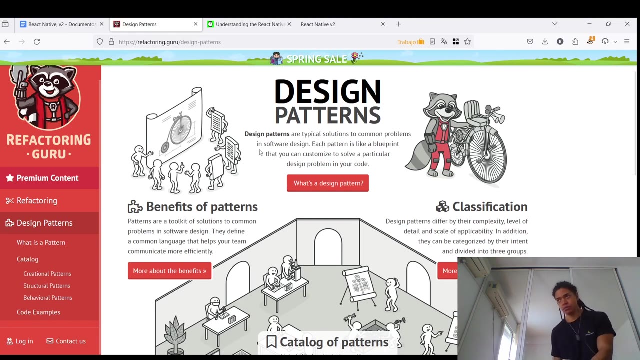 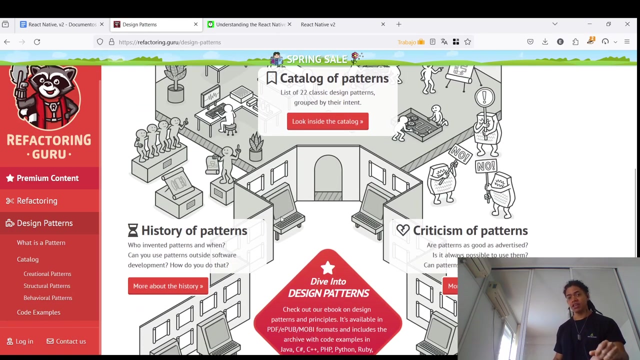 way of doing that. you do that in that way, yeah, so common problems come facing common problems with with typical solutions often. so there's some, of course, there's some benefits of using pat worlds, classifications, and there is a catalog of pattern, the history of the detractors or criticism. okay, our pattern, our patterns as we've. 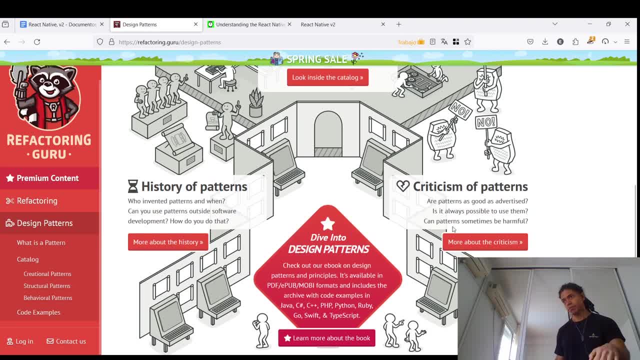 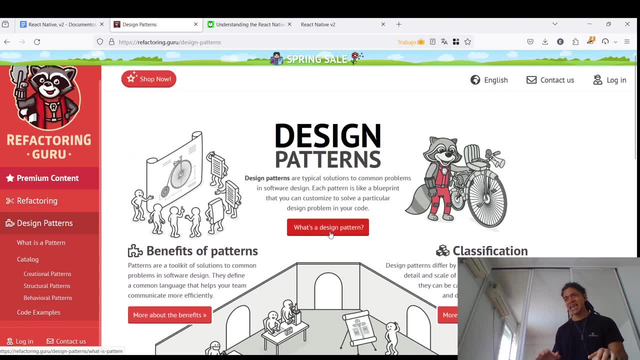 got the organ typing, it is always possible to use them. can pattern sometimes be harmful? yeah, it is, so dive into the same pattern, the. The idea of this design pattern is, as I mentioned before, okay, so if you have a problem that happened over and over and over and over, you're going to create build design a solution for that, a common solution or a typical solution for that. 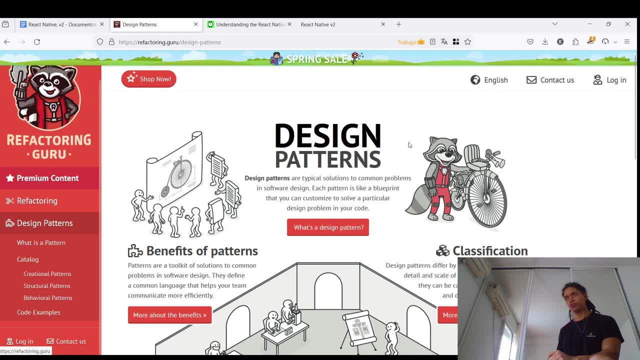 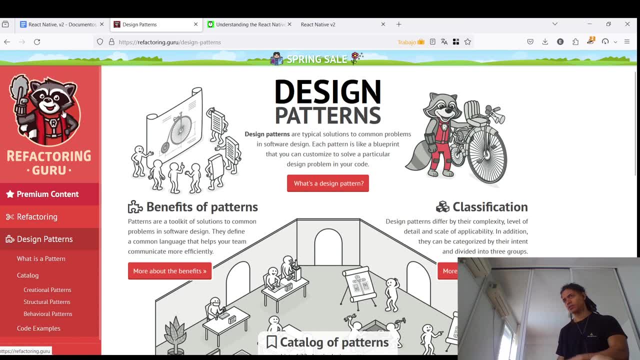 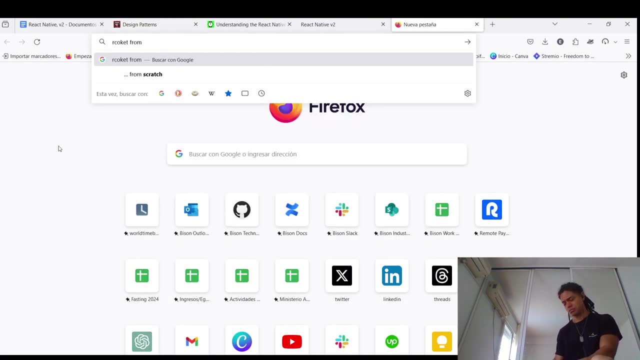 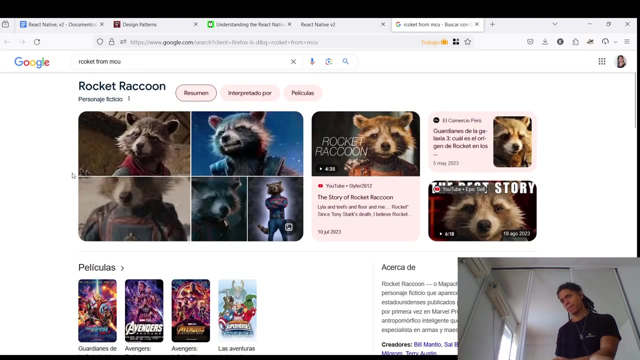 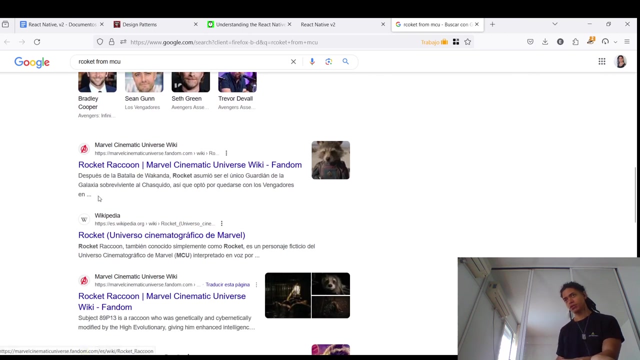 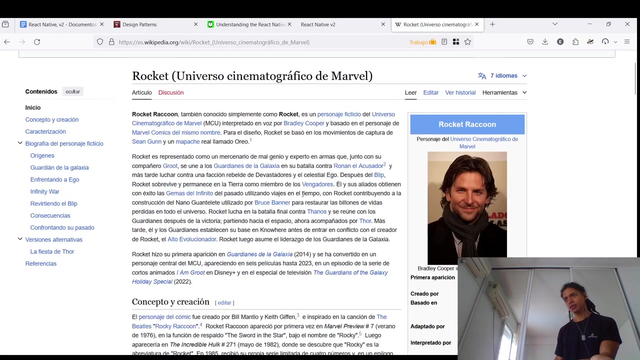 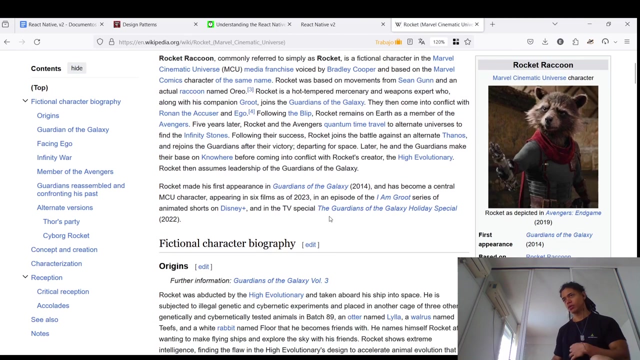 Okay, so now I get it why they're using this rocket for it. I never understand that. and now I know why they're using this rocket for that. From rocket from MCU. okay, rocket raccoon. exactly, exactly, Rocket raccoon. I don't know how old is rocket in the MCU. Yeah, I don't know how old is rocket in the MCU. 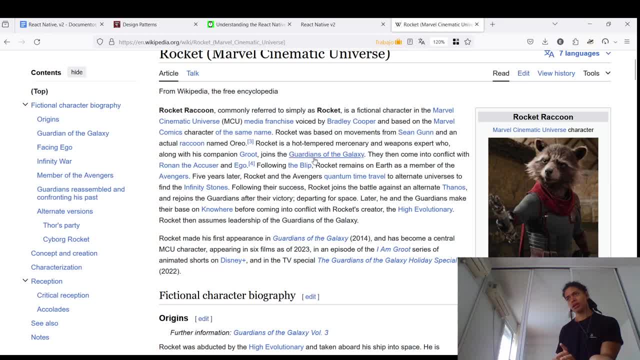 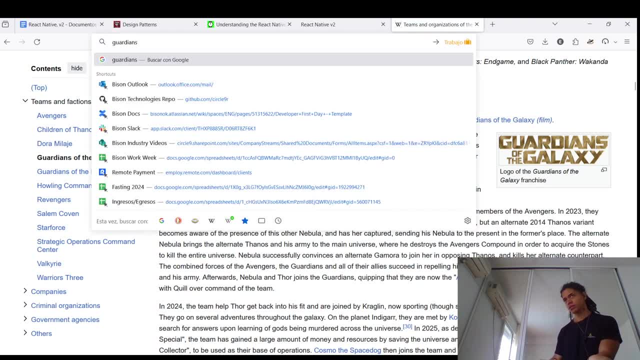 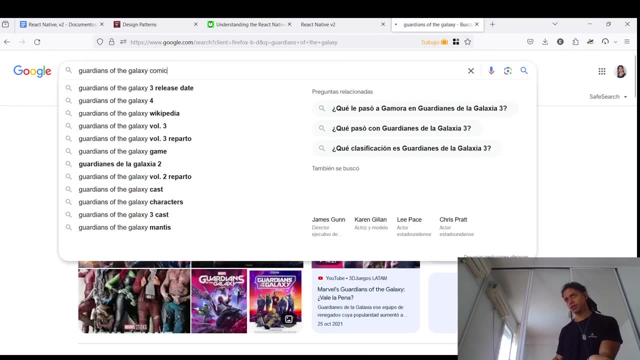 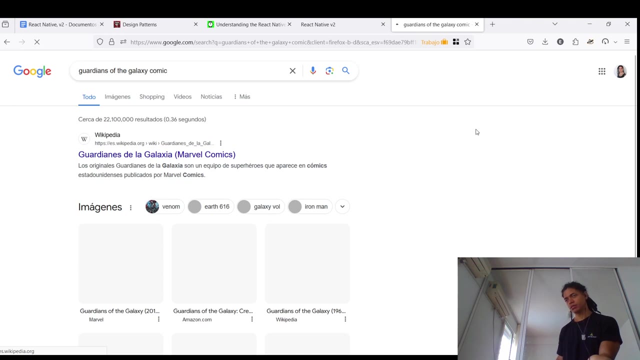 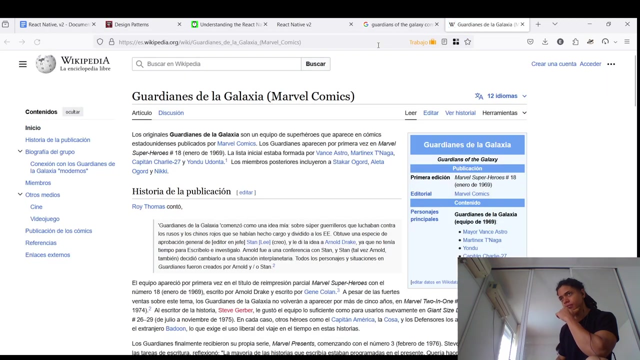 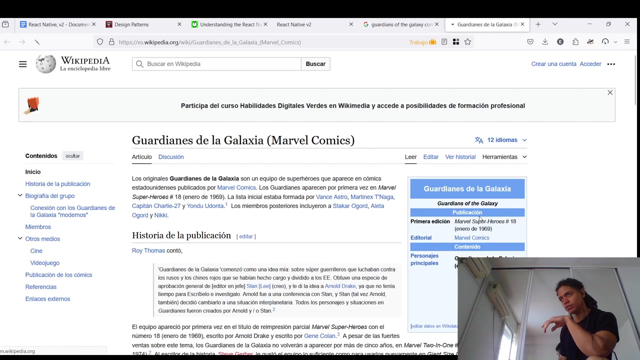 And not only in the MCU, but as the Garden of the Galaxy. the comics- Yeah, You know, Guardian of the Galaxy comic, like Marvel comic. okay, Okay, this is in Spanish. I'm looking for more interesting on English. You got it Exactly. 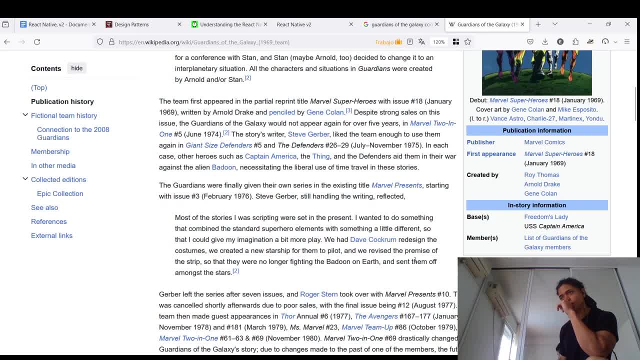 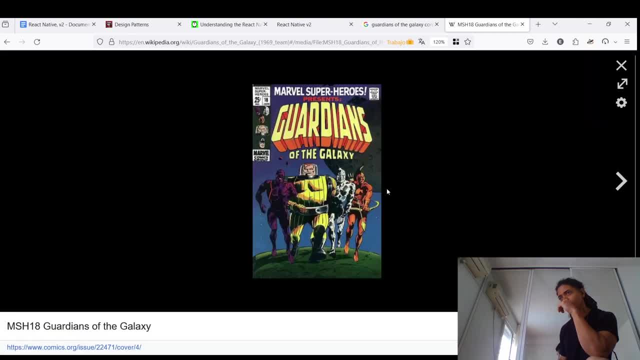 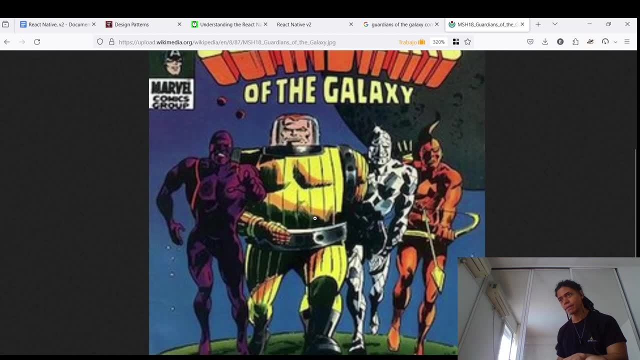 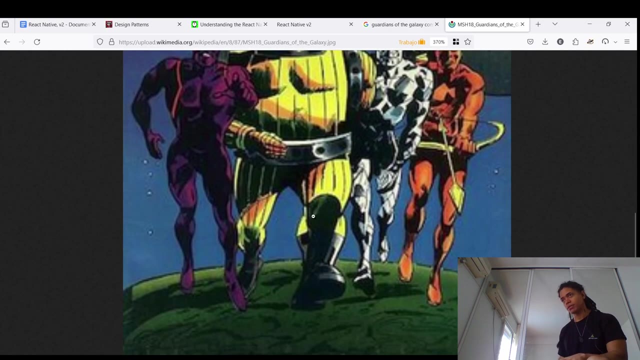 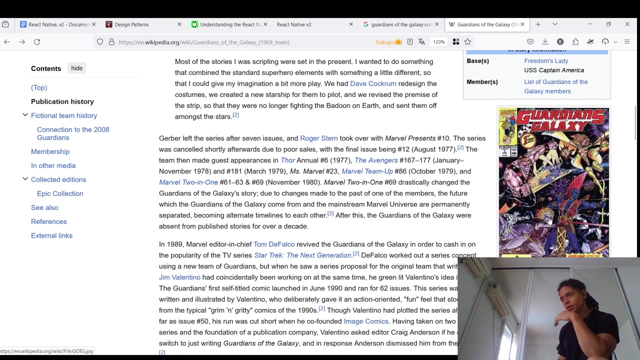 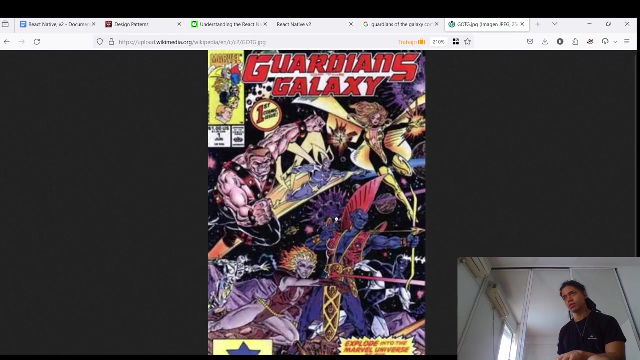 Guardians of the Galaxy- I think this is the original one. Okay, okay, Guardians of the Galaxy, And they have only four of them. okay, okay. And revival iteration of the team: okay, Okay, Very exciting, but there is no. 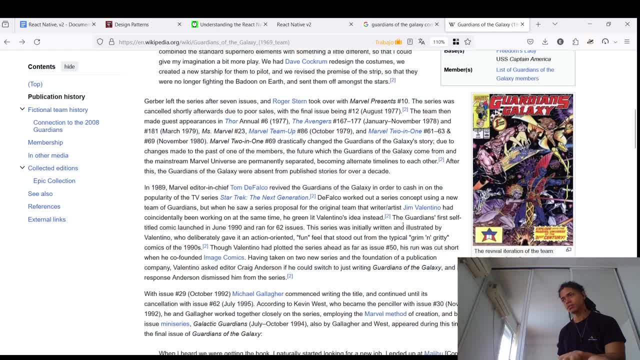 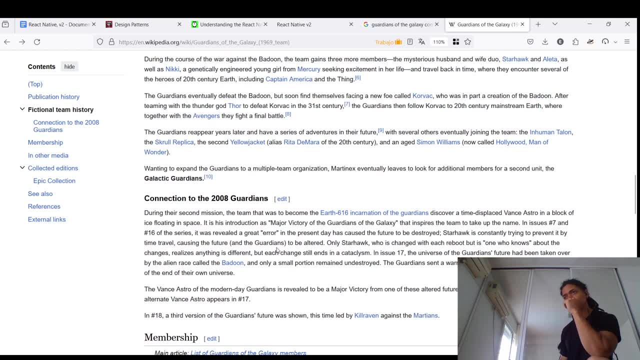 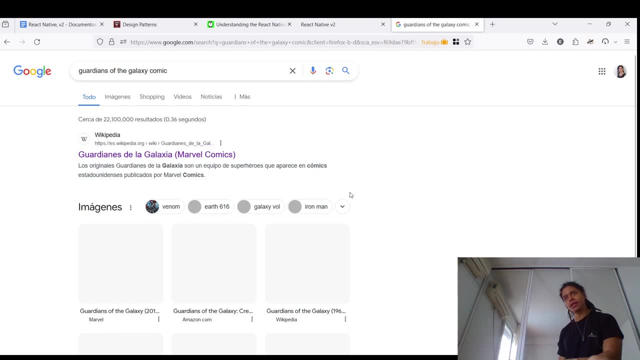 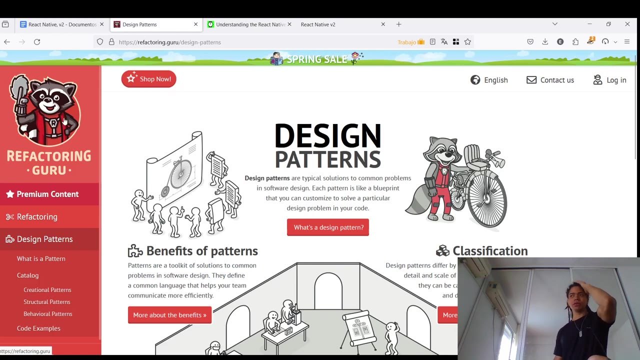 There is no rocket here or that, but yeah, you know it's like: okay, Guardian of the Galaxy. I thought they come, their logo, their image is from that, from rocket, but it is, but it is. 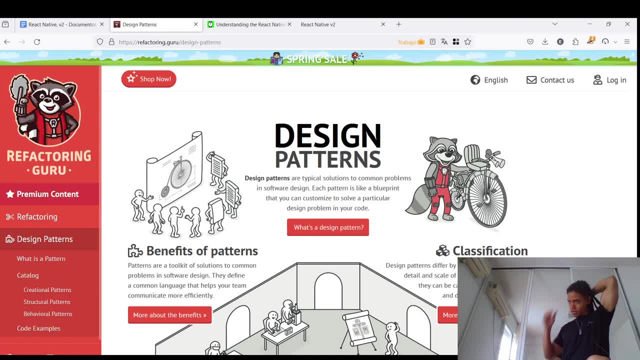 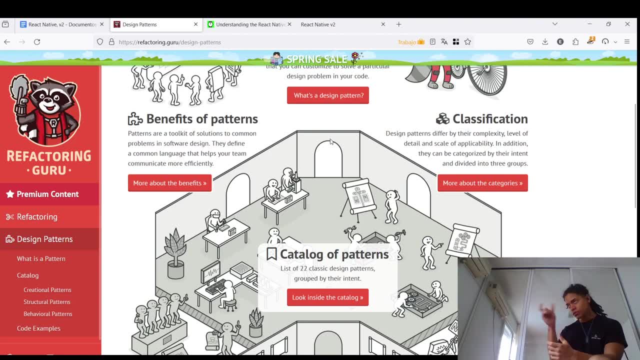 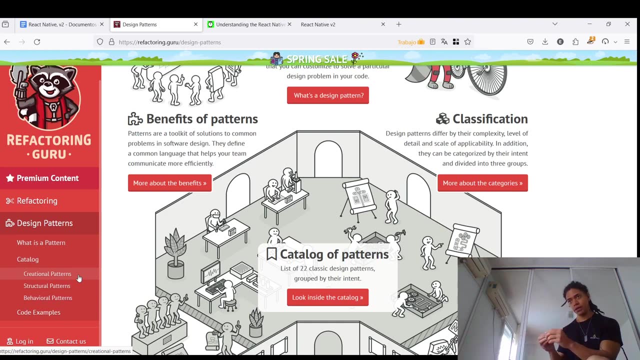 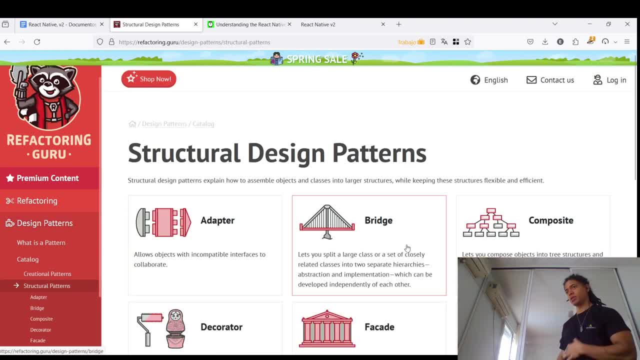 So, in the case of structural, we have this: the bridge and structural design pattern. So, in the case of structural, we have this: the bridge and structural design pattern. So, in the case of structural, we have this: the bridge and structural design pattern. 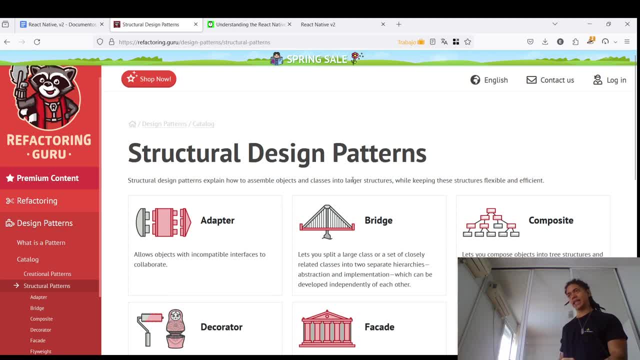 Explains how to assemble objects in class into large structures, while keeping these structures flexible and efficient. So, in this particular case, what we talk about is: how do we now make sense of this JavaScript code that can be now, that allows to generate, that allows to talk to any of this? 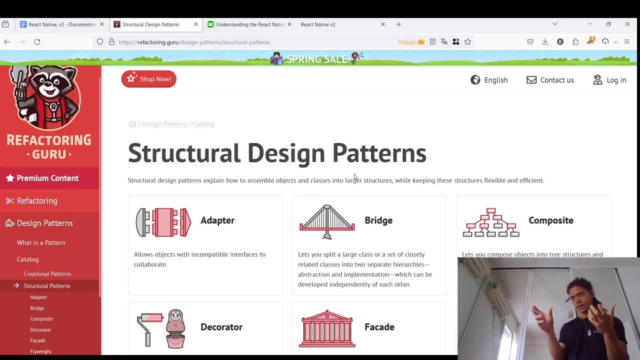 other platforms? Okay, Yeah, that allows to. so how can we, by having one language, Javascript, how can we make sense to talk to? to talk, Yeah, to talk to those mobile platform- Android and iOS- that they generate is the application or artifact that we need from. 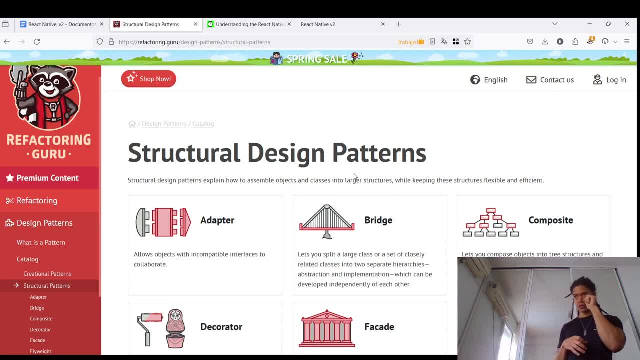 Based on the set of instruction in JavaScript. Okay, So how can we make, How can we communicate these different pieces? Okay, Together, okay, and actually, if let those different, That lets those different Objects, those different things be independent of each other, and they can now. 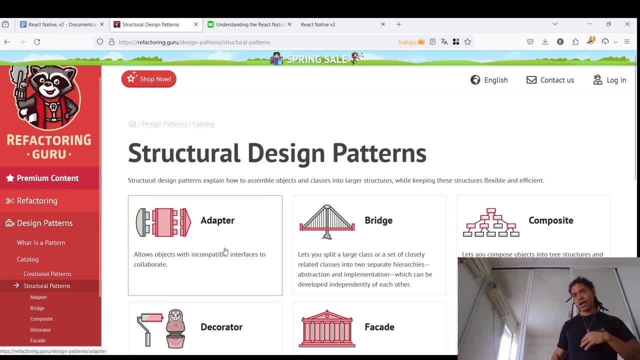 Interact with another. so adapters allow objects with incompatible interface to collaborate. So the use is an adapter Might be as well as a bridge. Let you split a large class of set closely related classes into two separate hierarchies so that they can be developed independently of each other. 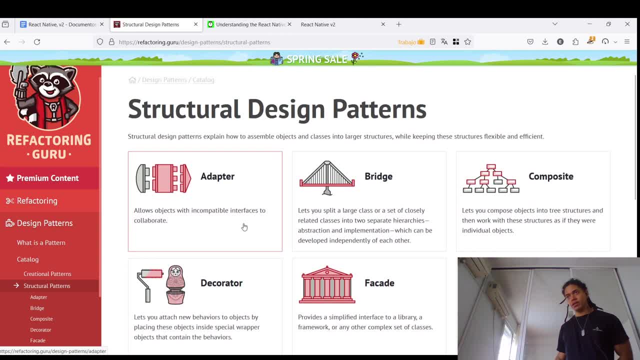 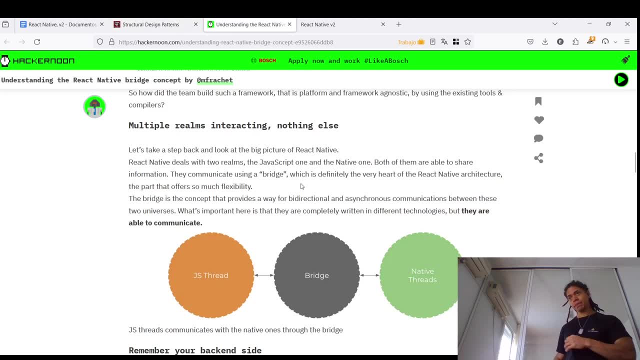 So in this case, I'm assuming that they use is the adapter. Okay, so how can we? what is the bridge that we want to build? Okay, I think they using is this adapter or, as they mentioned here, is on the bridge. the question is: 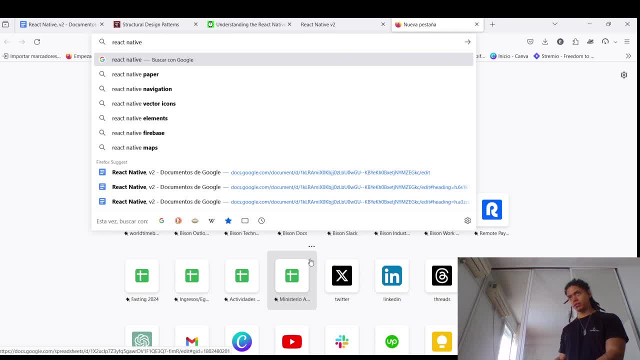 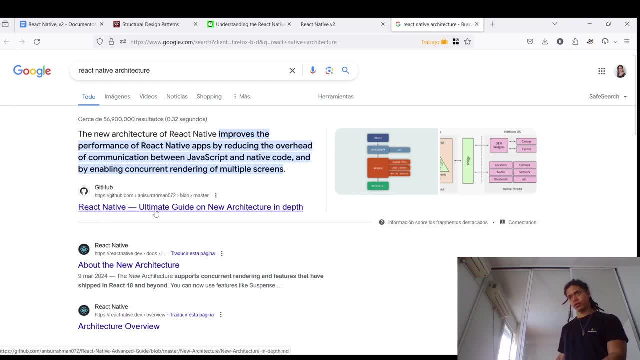 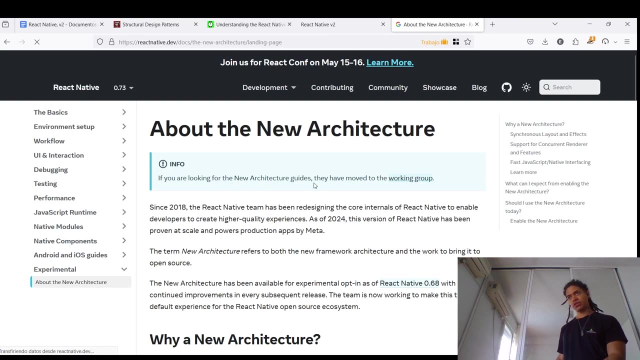 Do we have react native here? Architecture- Because I don't want to React native architecture here, If you're looking for a new architecture guide. they have moved to the working group. since 2018, the react team has been redesigned- the core internal of react native- to enable developers to create a higher quality experience as 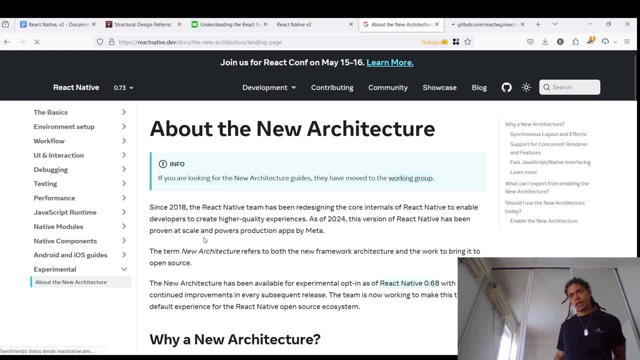 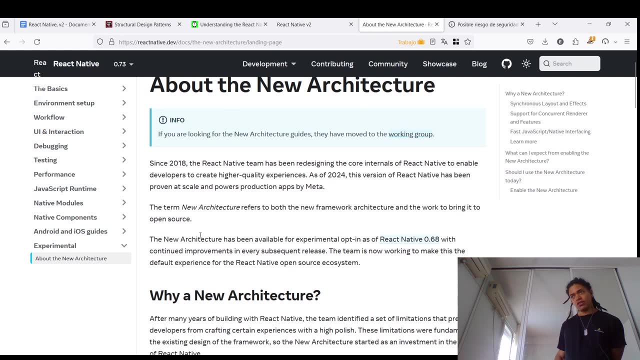 2024. this version of react native has been Proven at scale and power production app by meta. The terms new architecture refers to both The new framework architecture and the working and the work to bring into open source. The new architecture has been available for experimental opt-in in react native. 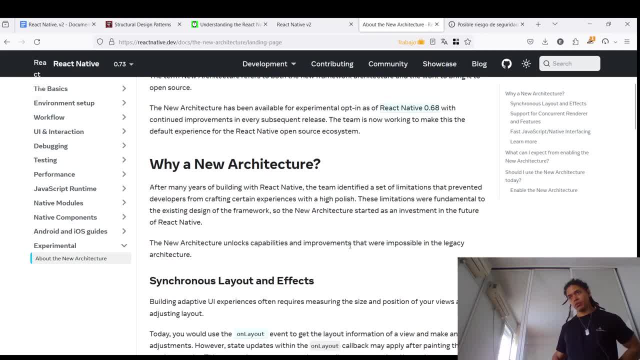 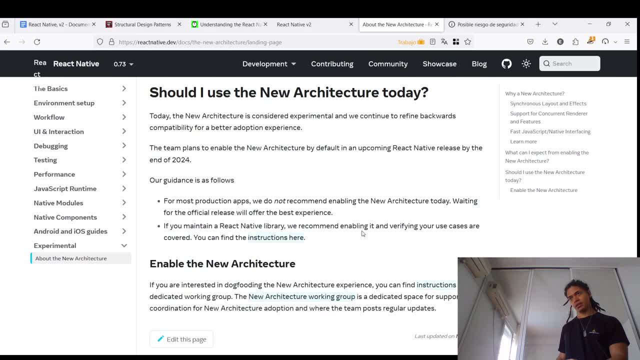 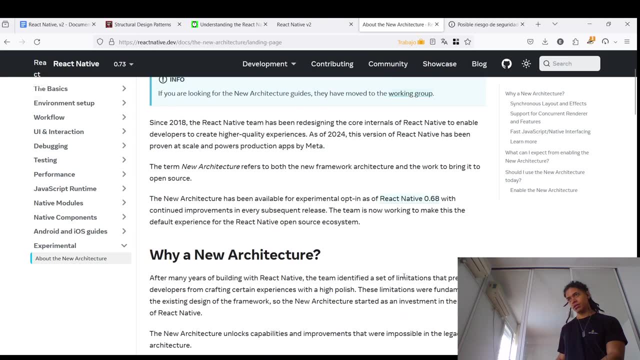 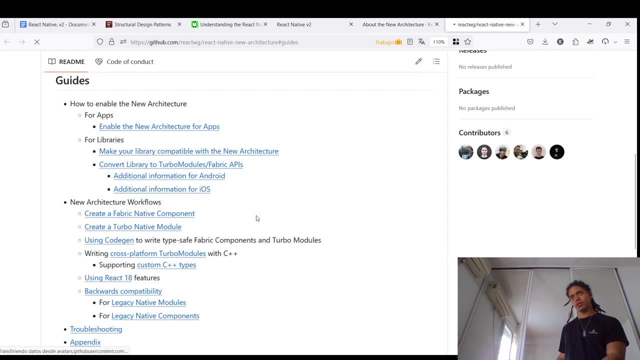 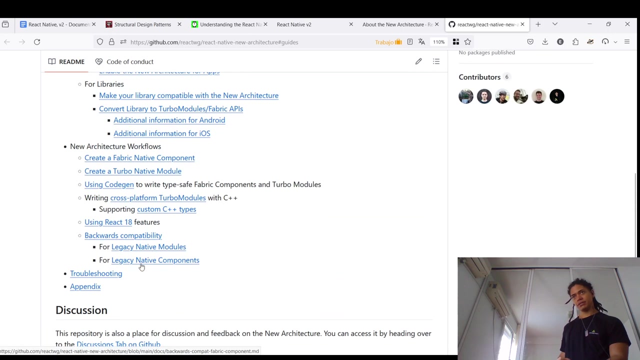 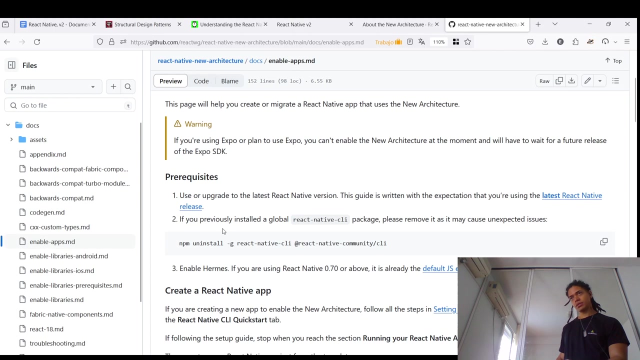 0.68, with continuous improving in every subsequent release. Do they have? is, For example, any little image, Because they have a lot of. They have a lot Really get react native architecture working, But I don't think they have is Enable the new architecture for app. If you're using export or plan to use export, you can't enable the new architecture at the moment. 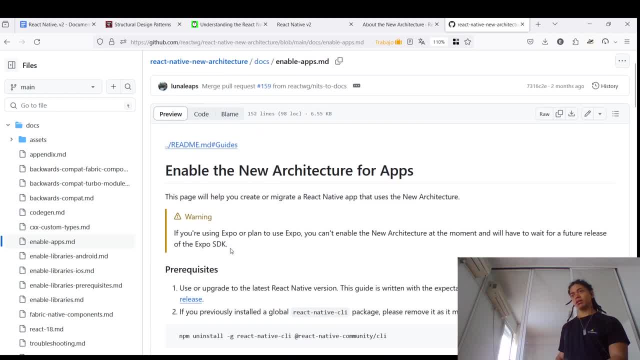 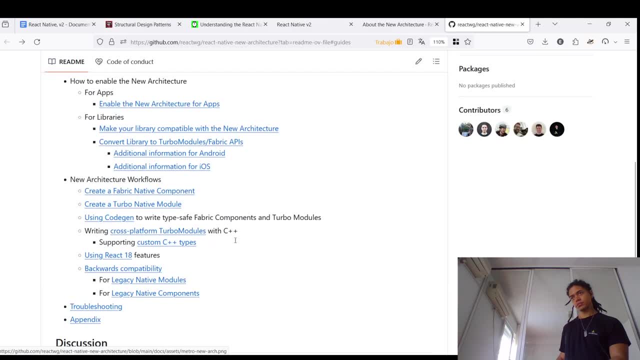 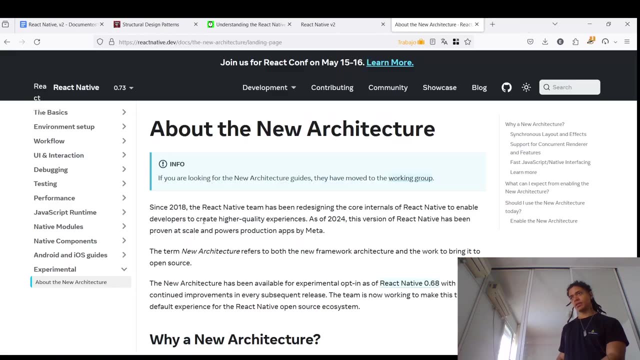 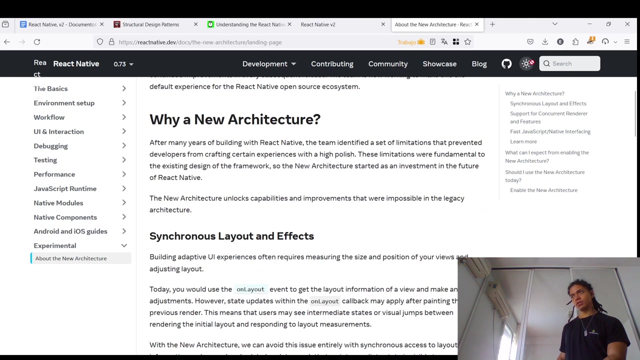 I will have to wait for future release of the export as you gain interesting, interesting. So very many gates are in any case. in any case, The idea here is to develop a sense. There are a number of's, The architecture, of the architecture value We would say. if I say, hey, what is the architecture here? 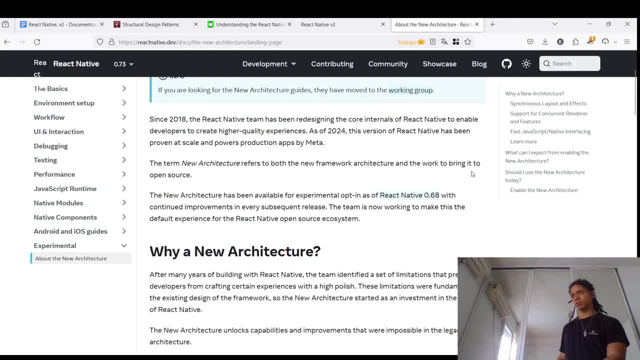 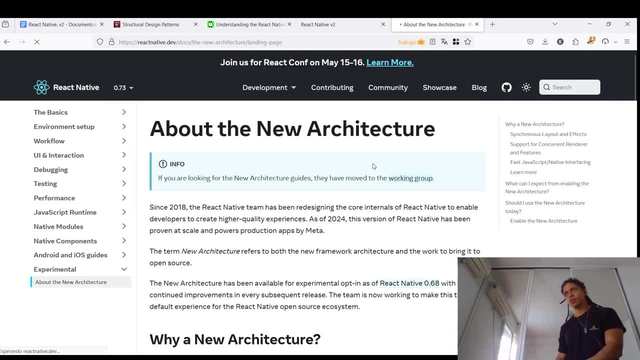 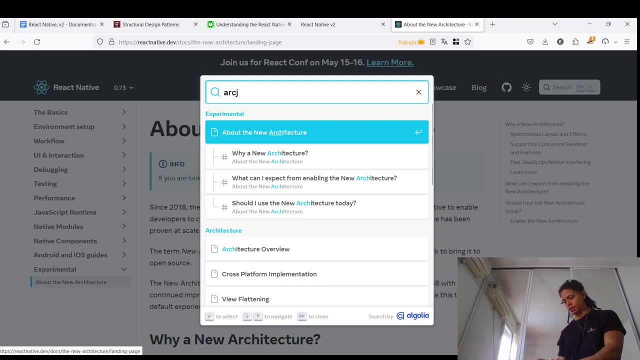 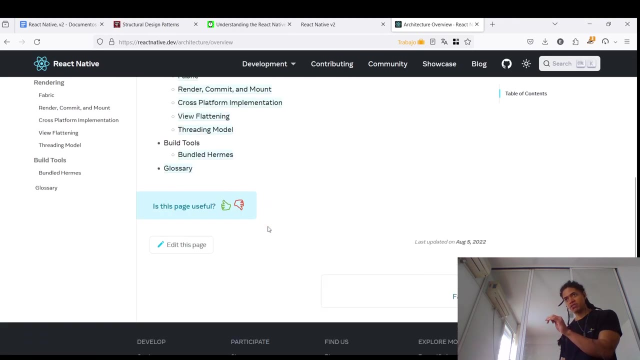 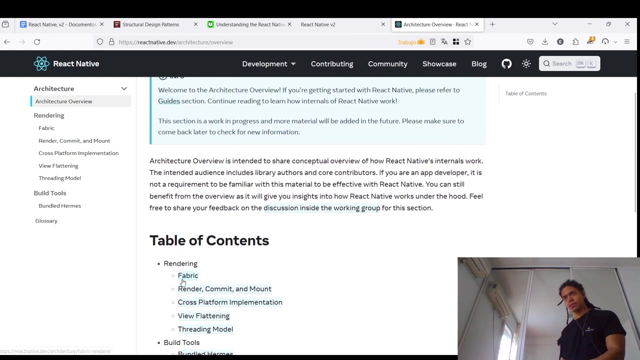 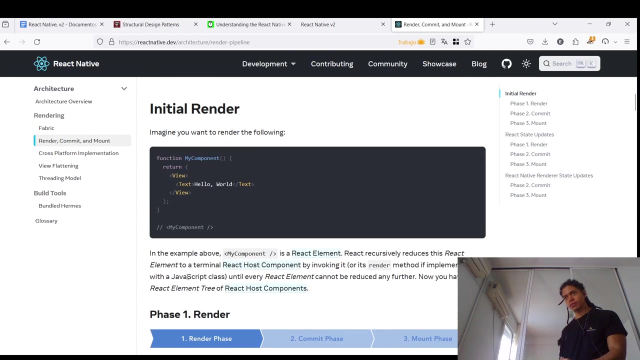 Come on Really. Come on Really. Come on, Okay, Thanks. The other in architecture: architecture, The architecture, The architecture of the texture. Okay, thanks, do you have Any new? any new image, things like that, rendering, build tools and glossary. yeah, but it's like render committed mount, we are going to three creation. okay, so cross platform. 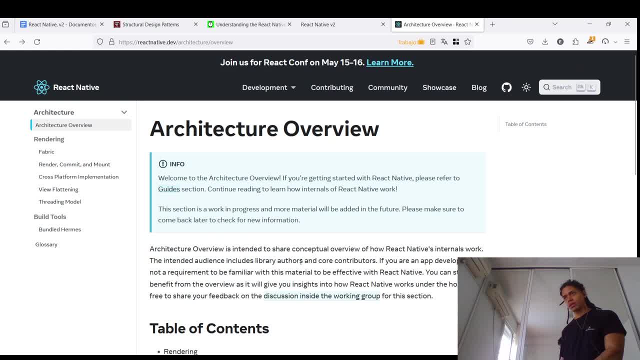 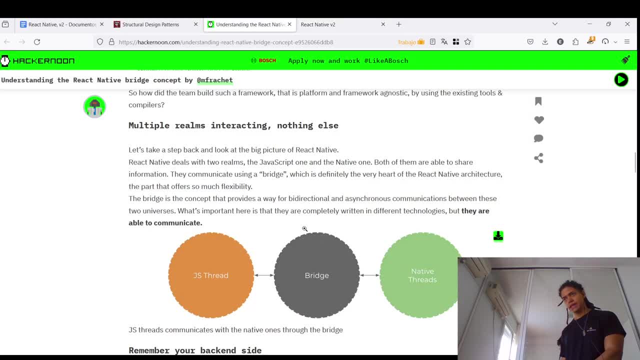 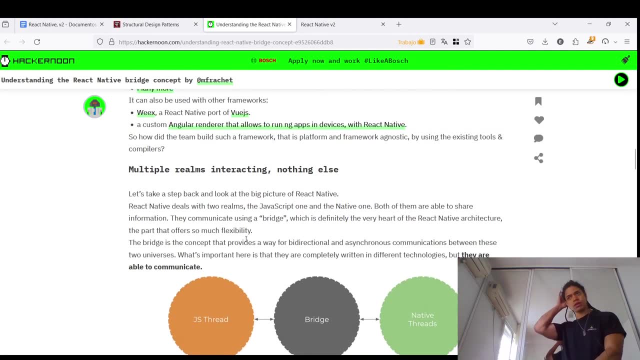 implementation. you flatter the entire mode. okay, for now I got this. I'm going to stay with this particularly. I'm going to stay with this particular approach. okay, so react. native working group say: hey, instead of creating a new, instead of creating something that takes JavaScript in output platform specific. 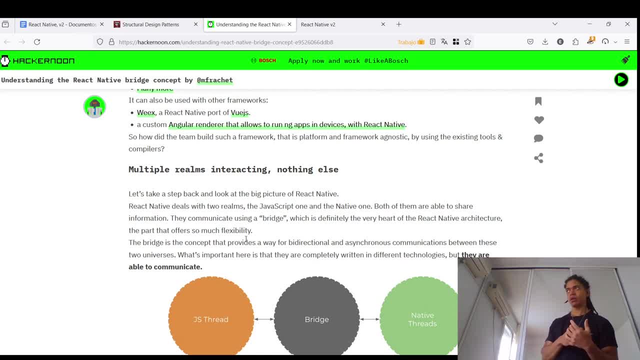 application. let's going to say something. let's going to now create a bridge or an adapter where now you can, given this JavaScript instructions, communicate to the actual compiler, to the actual render, the actual compiler, which is the under compiler, that it received now Java and cuddling, and I'll put you an Android app, or it received is a during the case of 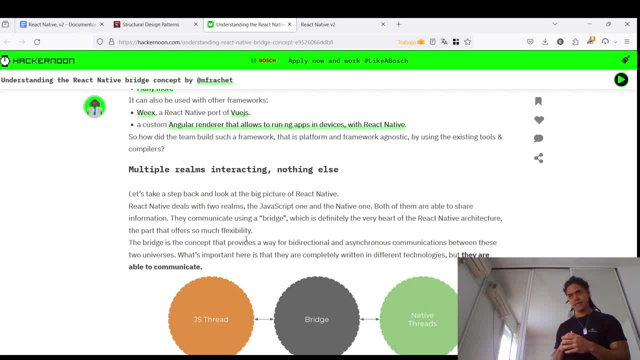 iOS. it we see is a an iOS. it received an option, XE or Swift code and then output using the Android the iOS compiler into Mac OS application or iPhone apps and similar to all of this. so this is something that is very powerful, because now, if the coupling from a lot of the couple, the 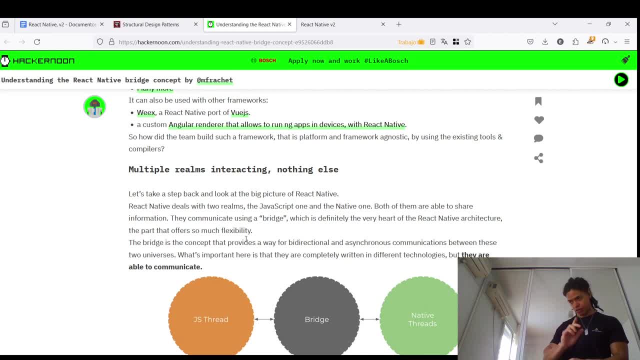 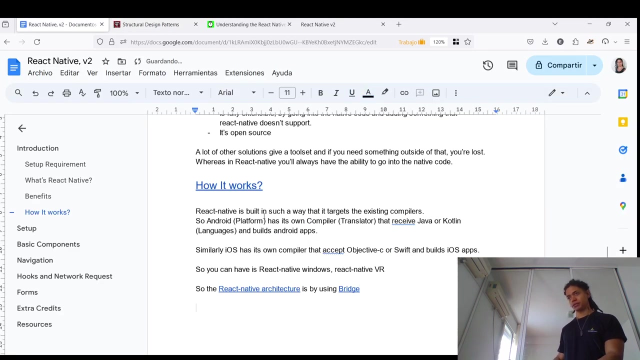 code make it much more modular in talking. be able to communicate to any. be able to communicate to any compiler platform specific, so it allows you these to build applications on Android platforms or iOS platform or Windows, even virtual reality. that makes a lot of them. that makes a lot of them. 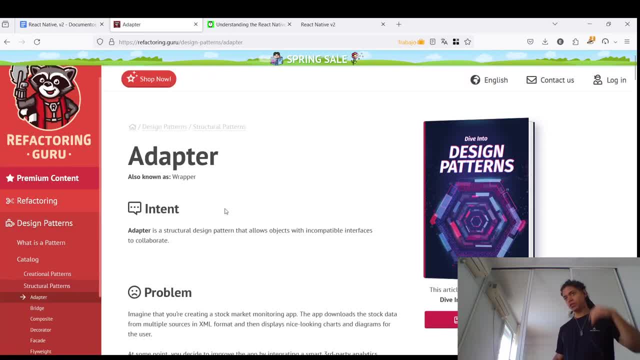 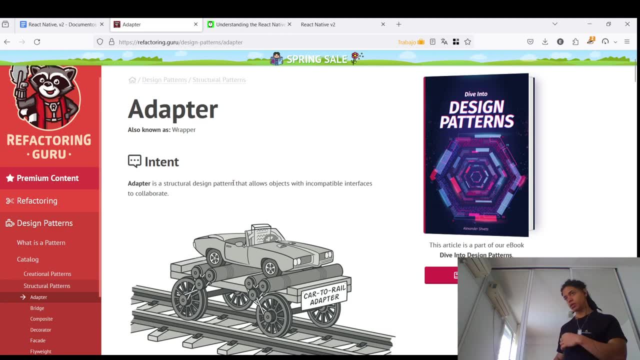 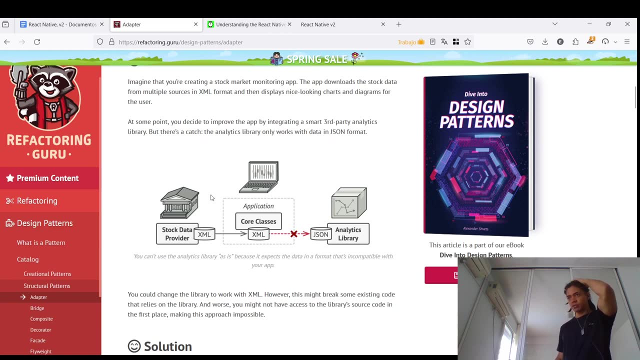 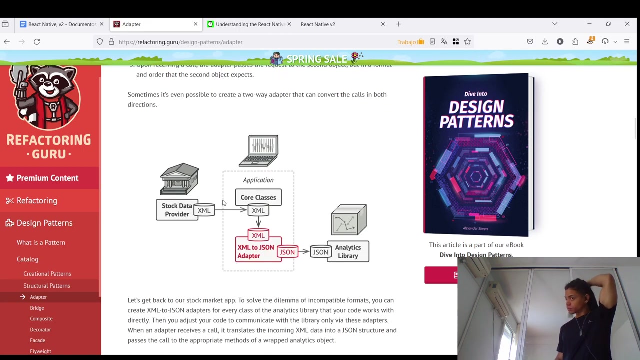 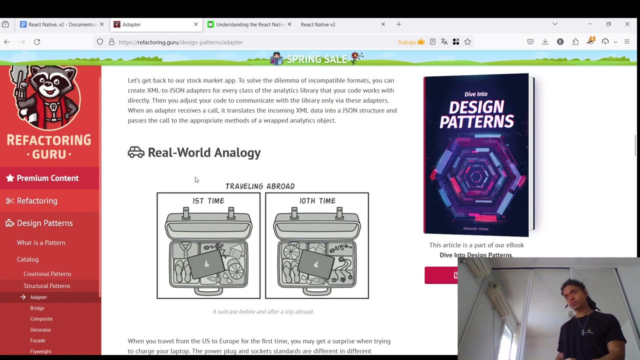 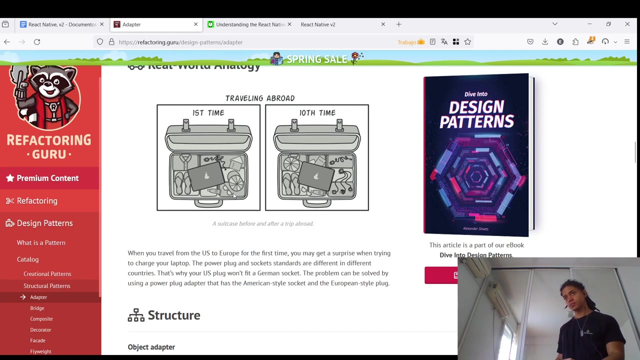 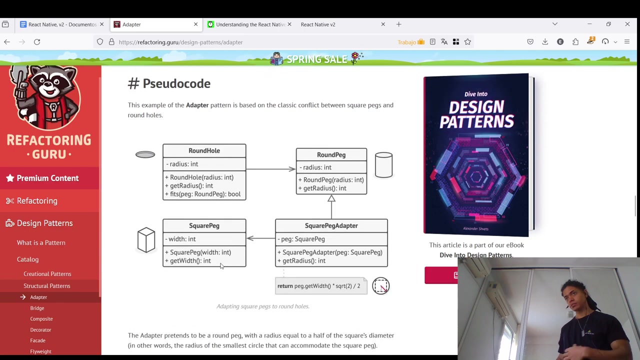 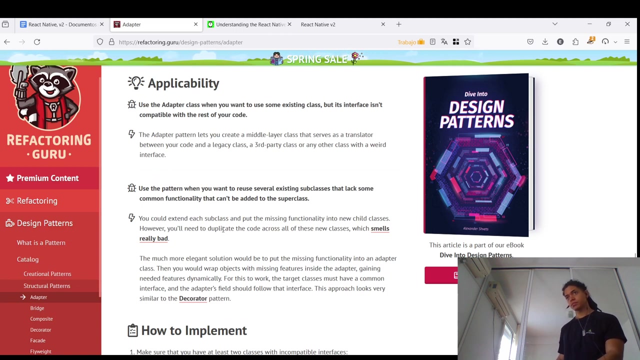 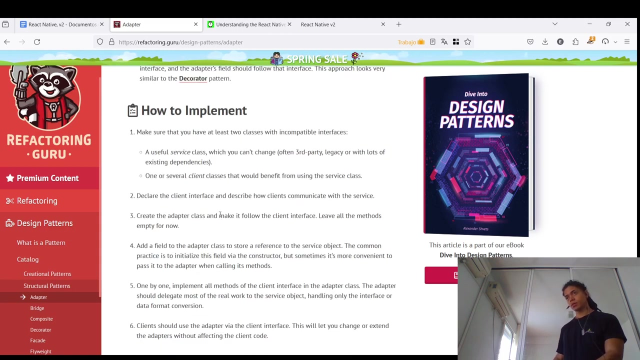 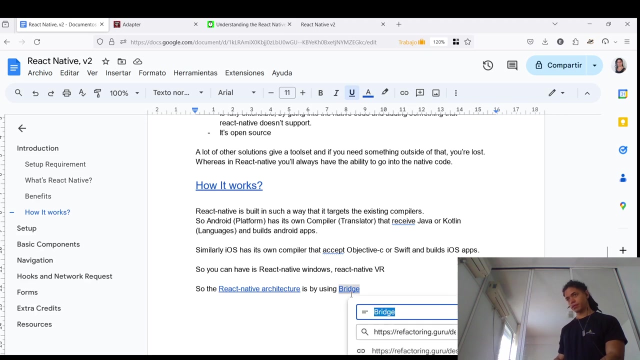 it leaves you on the2�레온. well, really using in the adapter. by the way, only using is the adapter a good end of an adapter. Thank you. Okay, the adapter. I think actually that's Presumably the adapter pattern. 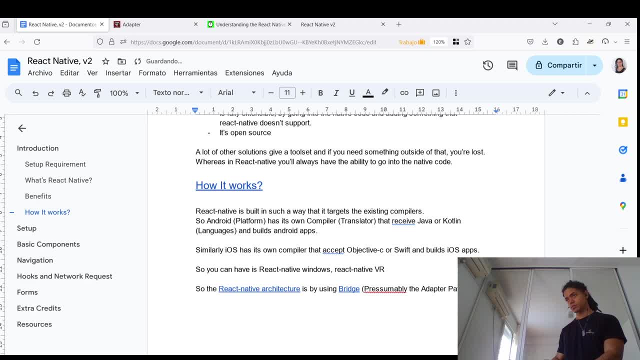 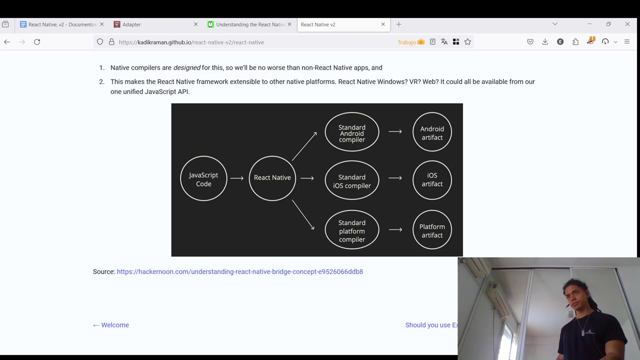 Okay, so presumably the adapter pattern. Okay, presumably, presumably the adapter pattern. Oh, okay, Okay, so presumably the adapter pattern. Yeah, so I have had a couple of occasions where I've had to build something native. 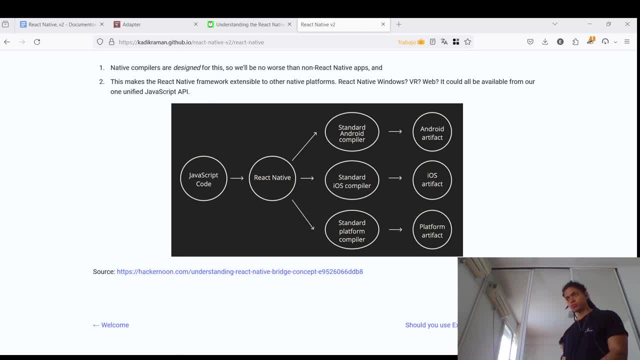 One works for, I think, for Android for linking into a particular mail provider, and the other is on my current project, which is actually pre-built before my time. One works for, I think, for Android for linking into a particular mail provider, and the other 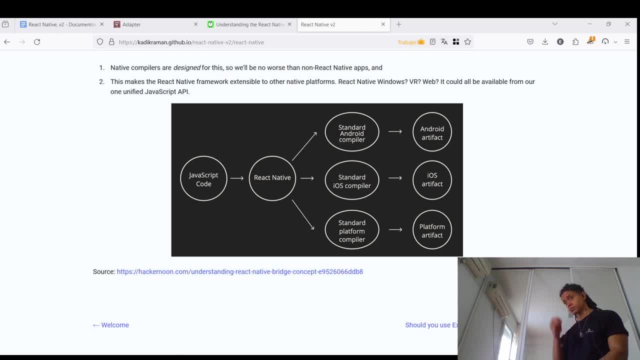 is on my current project, which is actually pre-built before my time, which is integrating with a payment provider that isn't available in React Native, So the platform fully supports it, which is one of the features of React Native. It's very straightforward. it's quite straightforward. I'm going to say very straightforward, quite. 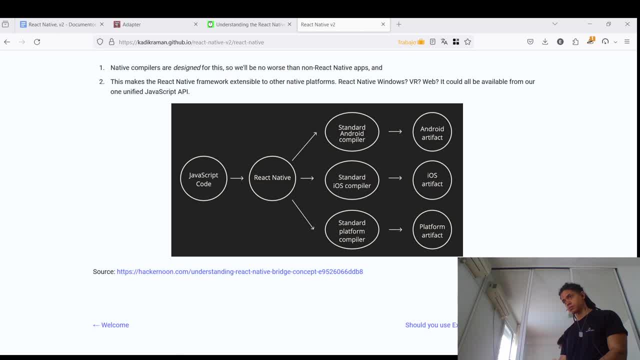 straightforward to bridge into the native code. So if you have, for example, if you need to add a new module or add a new component or add some native functionality that interacts with the native Java or Kotlin or Objective-C code, there's a particular entry point and there's a really good guide to how to do it. 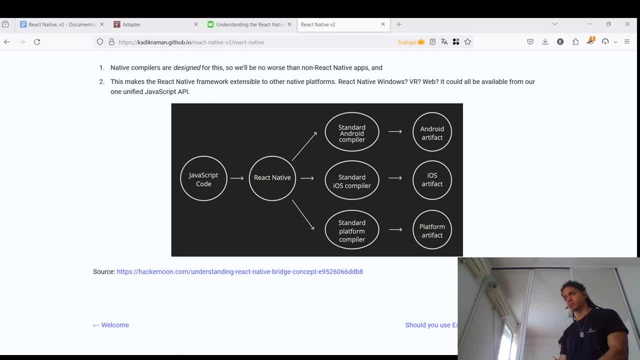 So it is quite useful. It is a bit of like a hassle, like I always like to say that, like I had written no Objective-C code prior to going to React Native, but now I wrote a security library, So they kind of lure you in with the parameters of just JavaScript. 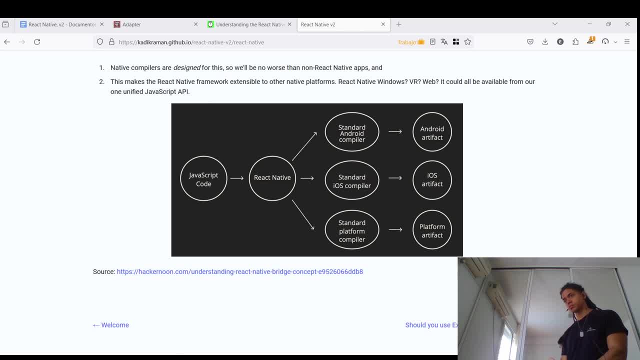 Yeah, And then you kind of start going like, oh, let's do this little bit in Java, So you do actually get to like, learn these new languages. Yeah, so to answer your question, it's a bit of a hassle in that you try to stay in the React Native. 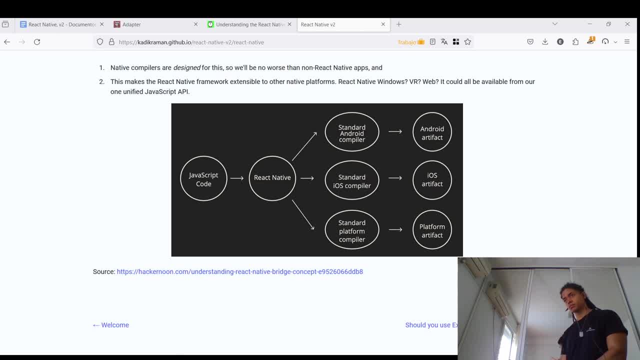 space as much as possible, but if we have to go outside of it, it's not very hard to customize it. in fact, yeah, Is there like a We have to. So, oh my god, That's a very interesting question. React Native. Any other ones From those languages? Yeah, So Can I take this for a guess? with React Native, Can you get a native solution from those languages? This day and age, like 2,000 phones, you can use React Native API. 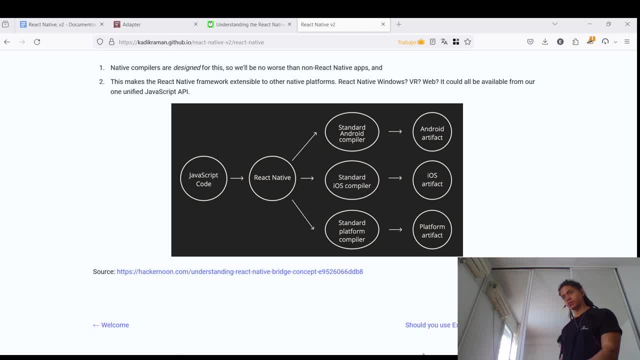 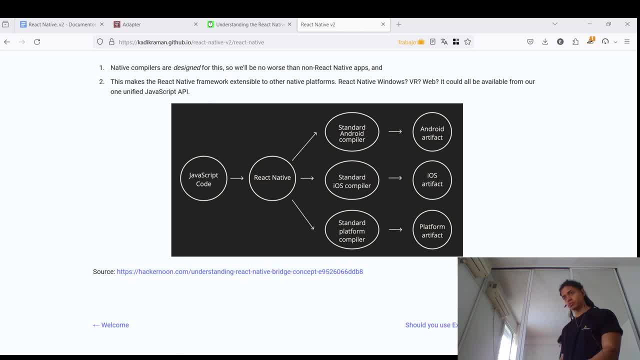 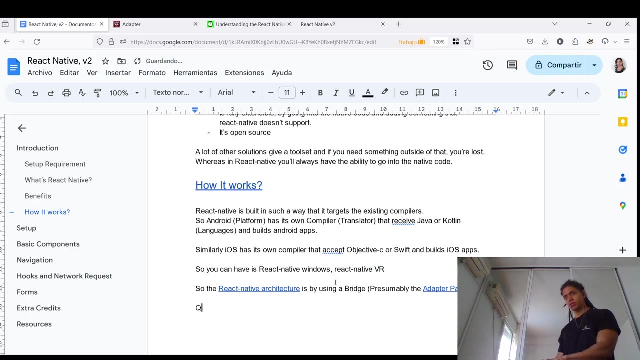 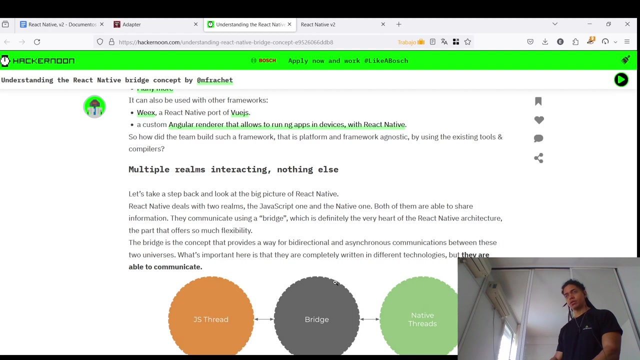 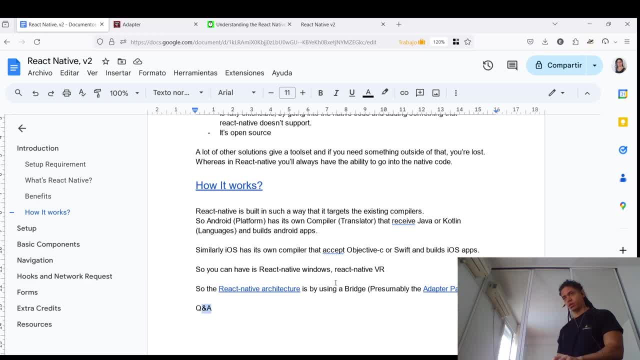 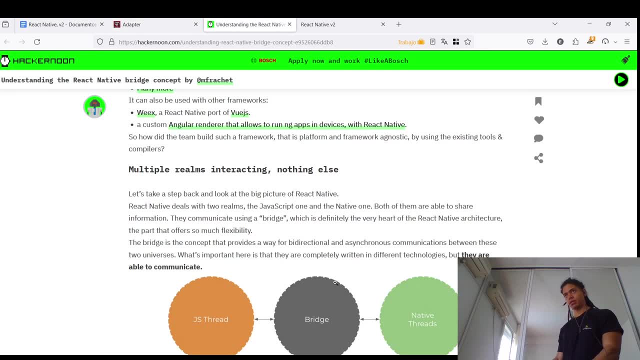 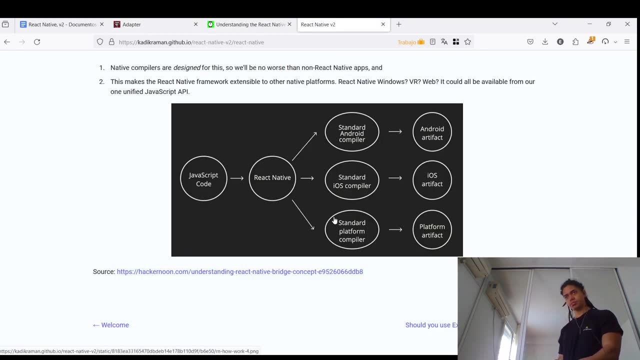 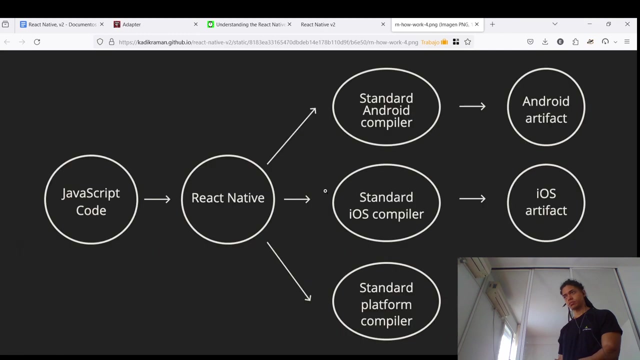 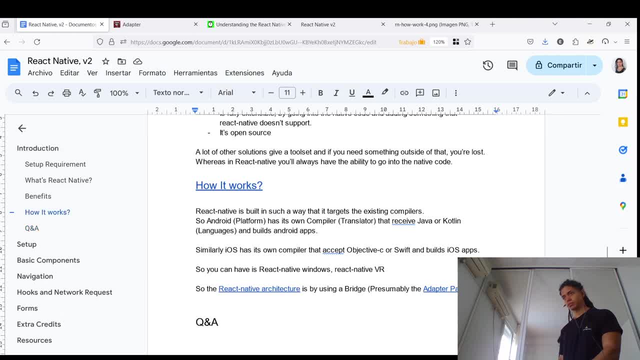 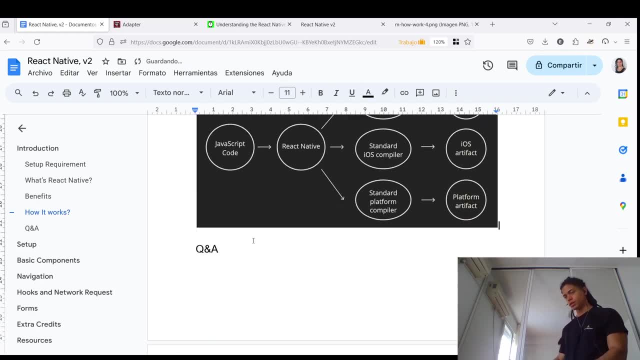 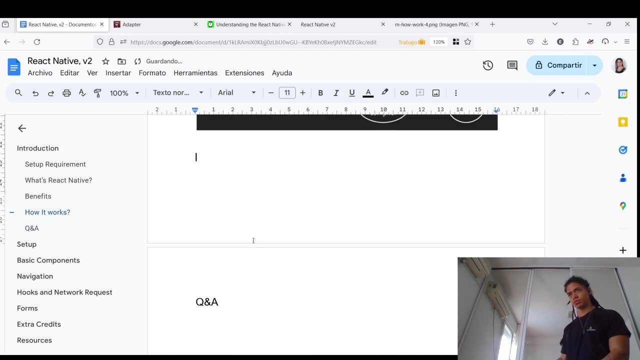 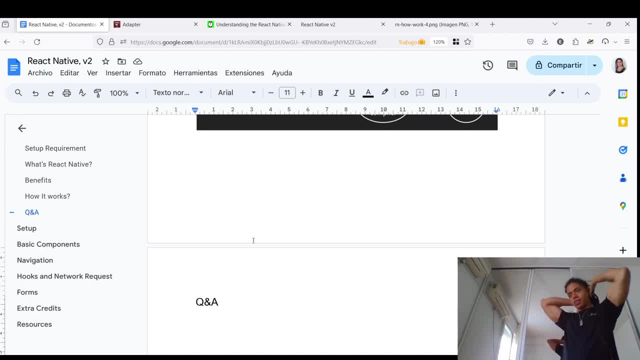 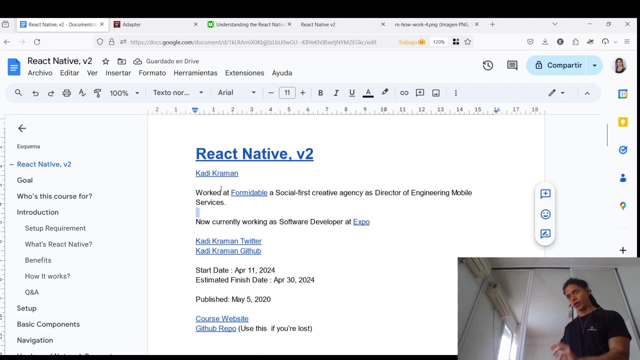 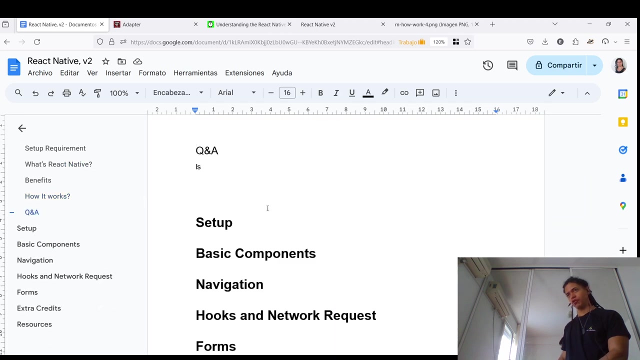 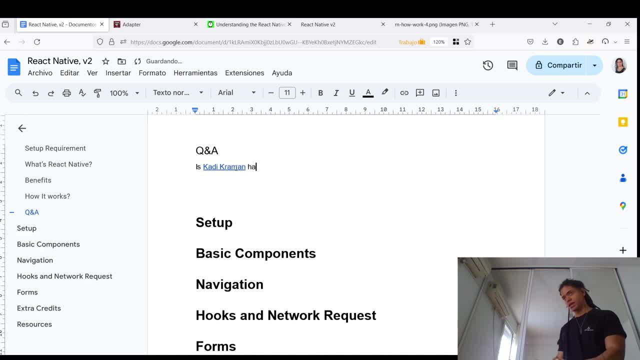 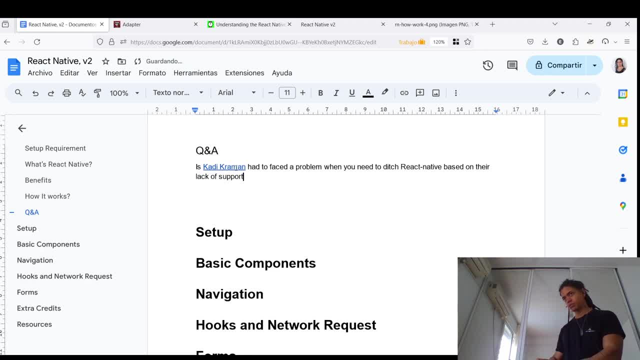 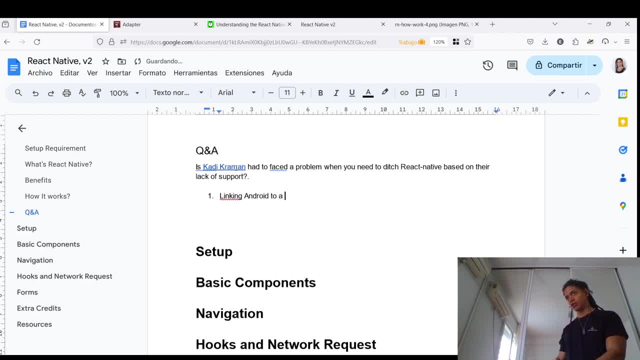 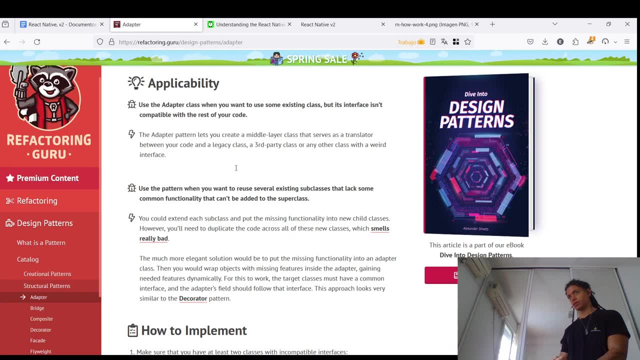 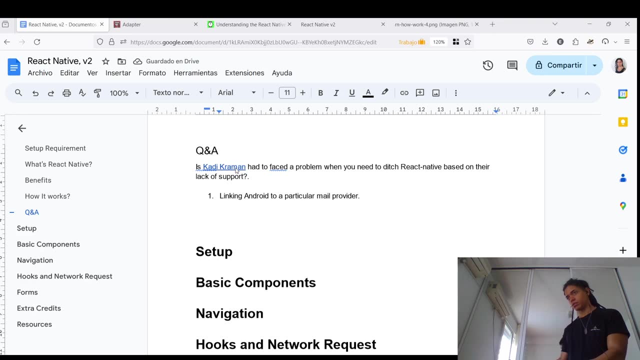 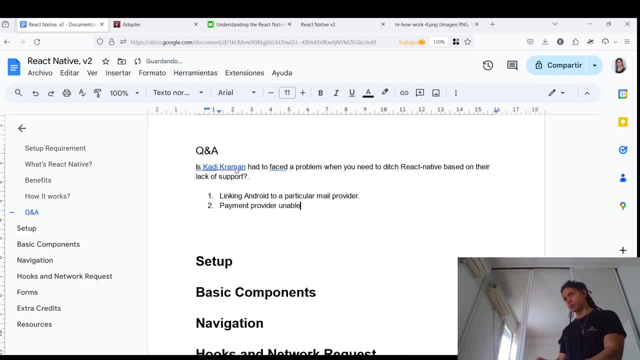 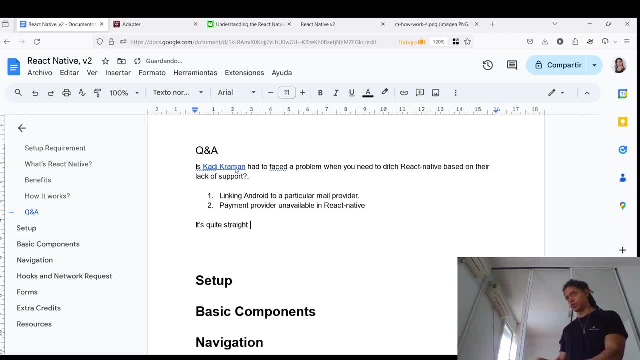 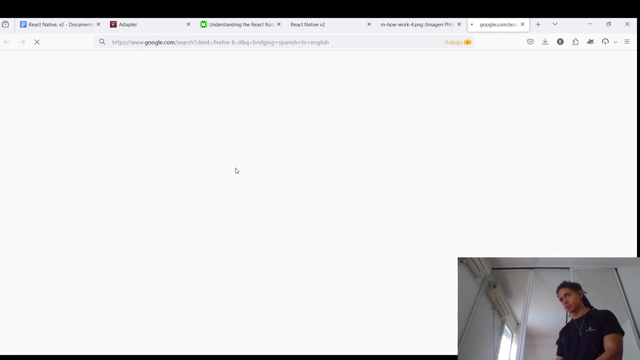 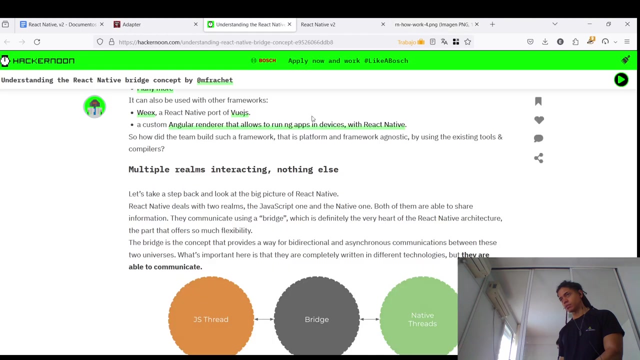 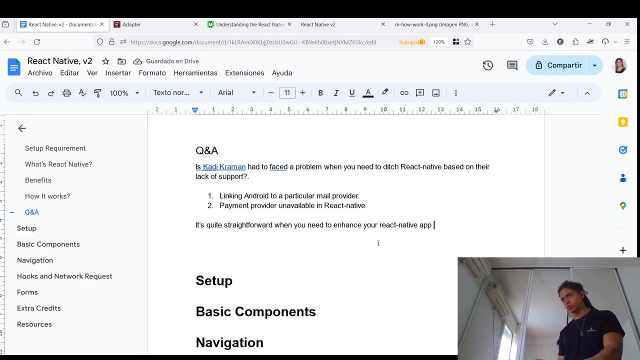 that it's completely. it's quite straight forward. when you need to enhance mm-hmm- your app, your react native app bridging, bridging mm-hmm- you react native code to native code. if you have the number, if you need to add a new module or add a new component or add some native functionality that interacts. 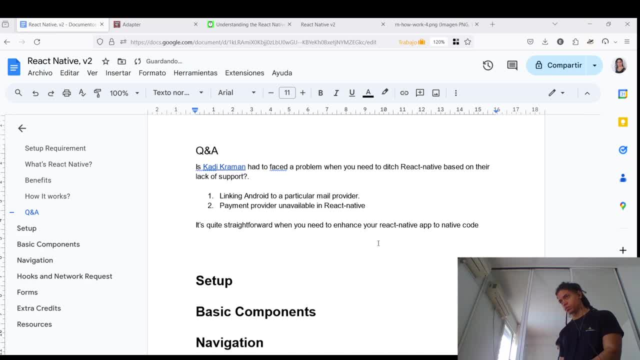 with the native Java or Kotlin or Objective-C code. there's a particular entry point and it's a really good guide to how to do it. okay. so, if you need, if you find yourself interacting with this particular code, if you find yourself interacting with this particular, with this, with- 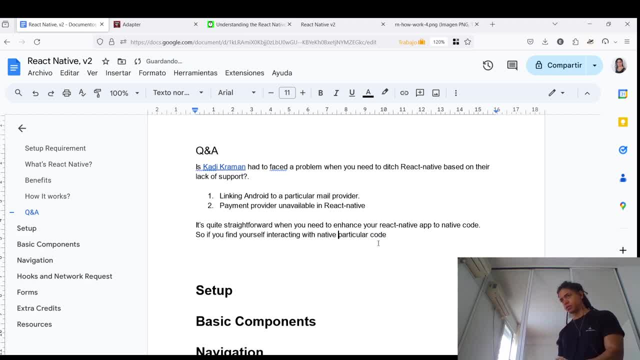 a native particular code that react doesn't support it. they are nice, they're really, according to her. they are. they're good guy on how to do it right now with the. so with chat, gpt, it's like we can do this fast. um, so it is fully accessible. it is a bit of like a hassle, like I always like to say that, like I. I 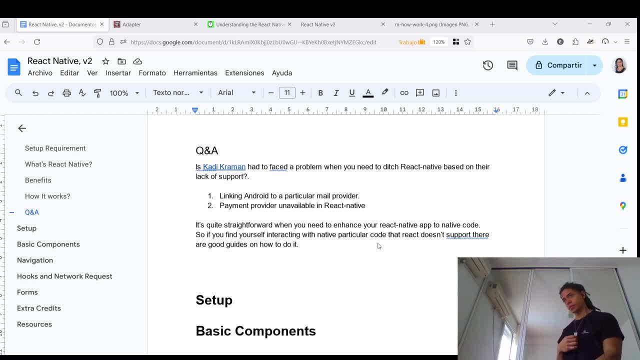 had written no Objective-C code prior to, uh, going to the app native. but now I wrote a scooter library. but that's the beauty of this. there's a beauty of this. it's like it is a bit of like a hassle. like it is a bit of like a hassle. 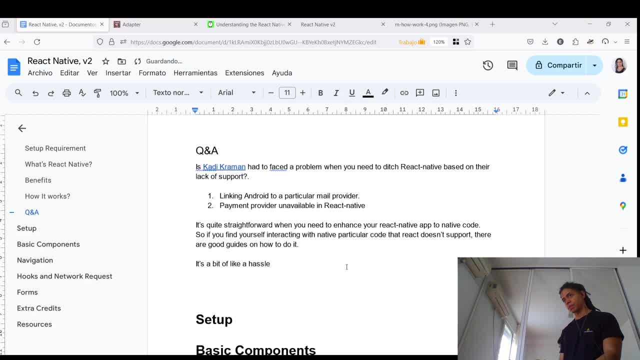 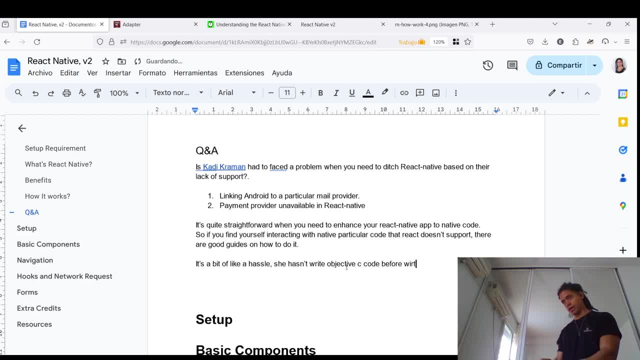 how, before writing, react native, then before writing, react native, so if they kind of know, you end with the promises of the scholarship and then you kind of start doing like, oh so you, you do, actually, you do actually going to learn those language. yes, it's a bit of a hassle. 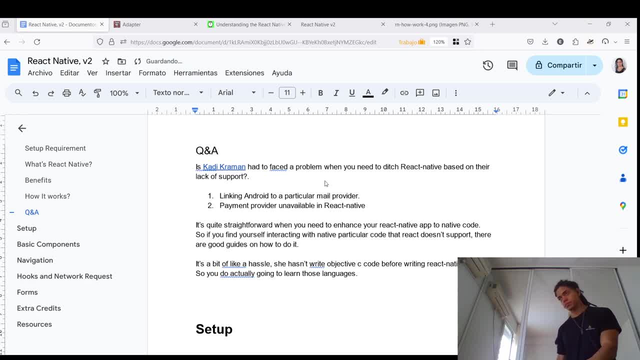 you try to stay in the back of the face as much as possible, but if we have to go outside of it, it's not very hard to recognize it. is there like a category, of a new sort of category, which which apps you might want to stay away from? the 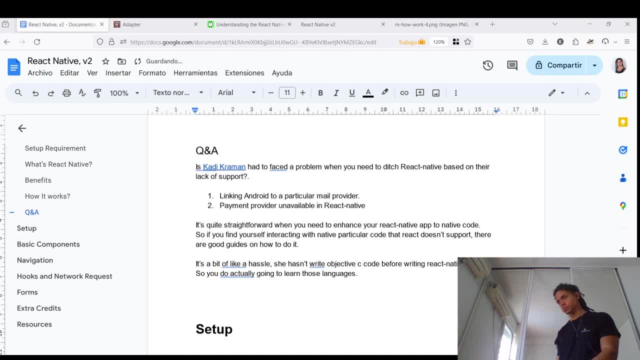 crack engine like, maybe highly graphical in terms of where is that? I'm right there, not sure what you can build anything react native. so, even though it's our ship, you actually hook into the late components that form so and where it's being? two years ago, there was a performing hits for certainly intensive 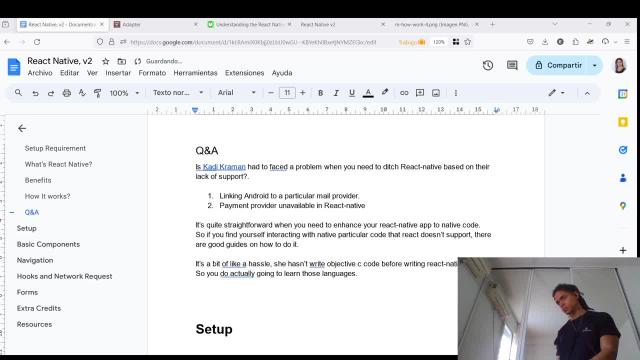 applications. as we progress, the, both the navigation libraries and Jags itself have grown more and more performance. you might have heard of hermes. it's a new Joseph compilers that are just a couple of years old. you can use the, the app to compiler that they are building, at least recurrently, which is optimized for javascript. exactly this is. 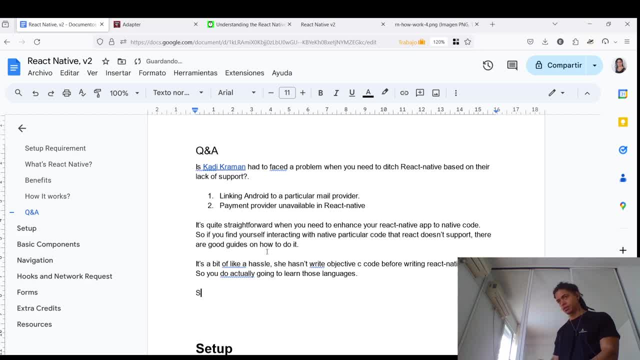 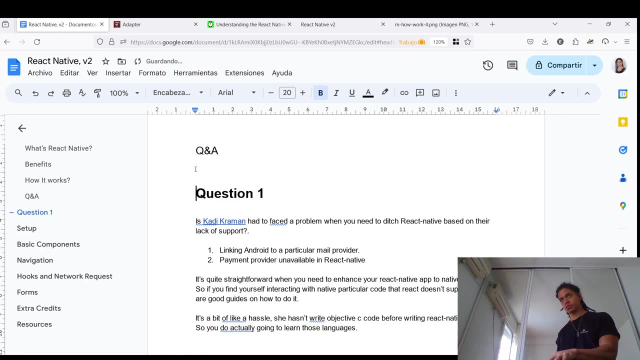 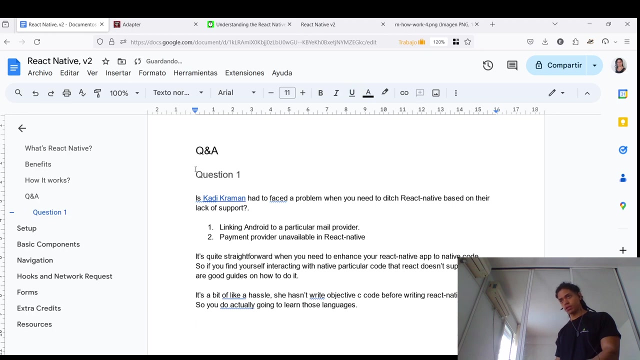 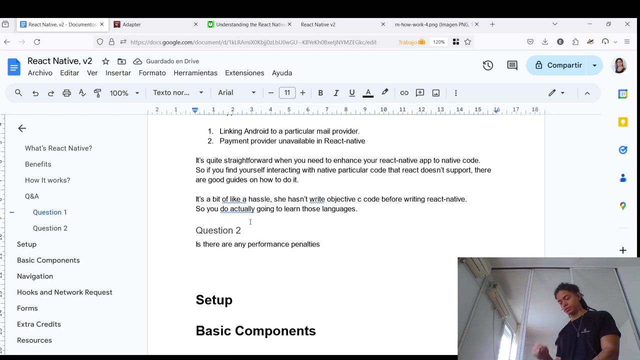 okay, hermes. another question is question one and the other is question two. is there are any performance penalty penalty? yeah, is there any performance penalty when writing? when writing applications, is there any performance penalty? or is there any performance penalty? or is there any models that that we need to stay away? 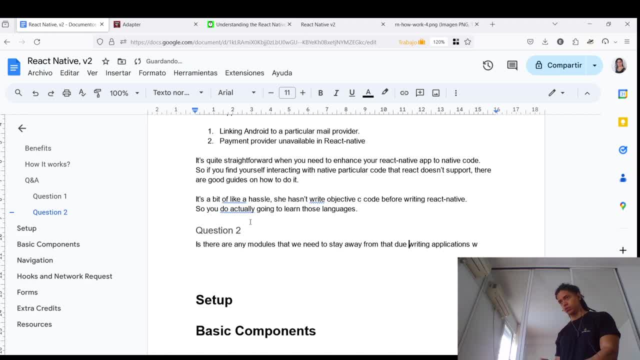 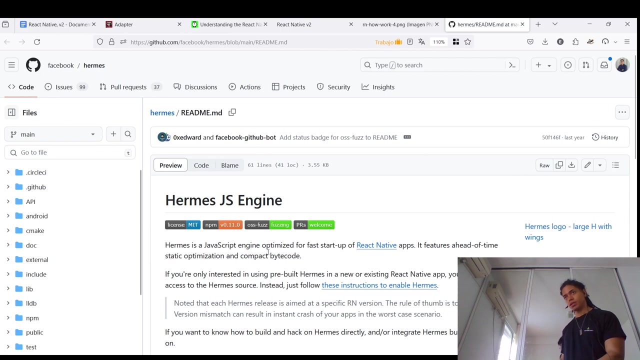 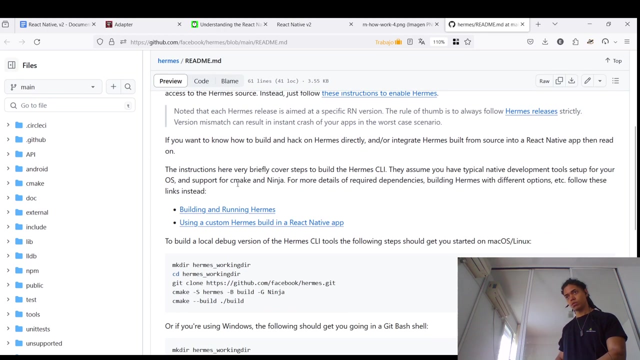 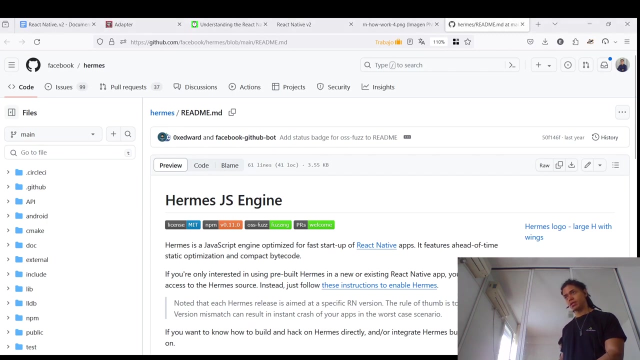 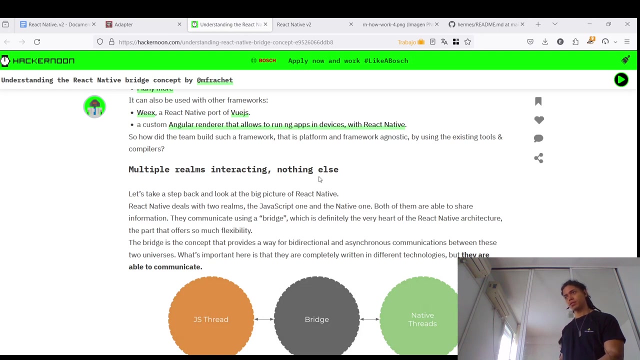 stay away from that. do performance penalty when writing application, when writing react application, and for what we're doing, since facebook is building a javascript engine specifically, specifically for react, react native gas, ding Whole thermos, Yeah, Okay, The fact Holy. And that's just an example of one example of the optimizations that they're doing. 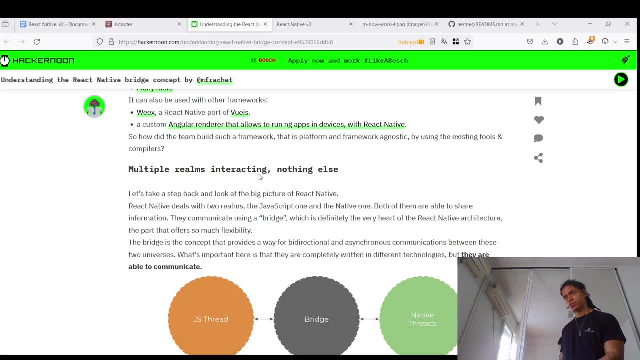 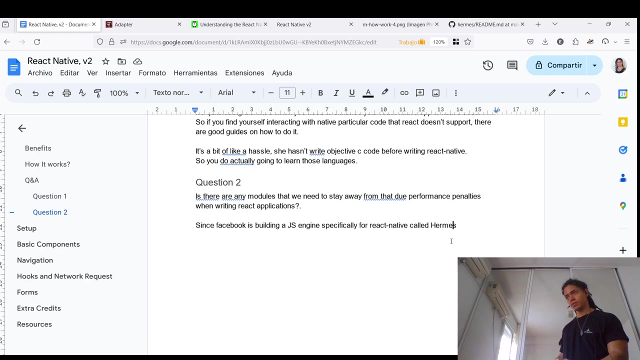 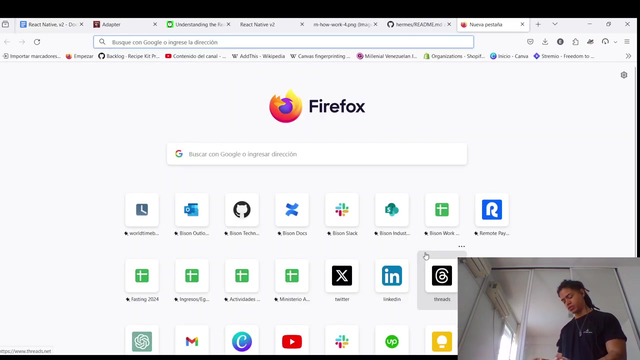 Yeah, I don't think there's anything you can do. According to her, holy moly, okay, You, You, Okay, holy moly, His facebook is building a javascript engine specifically for react native called hermes. There is no, even though we just When you take a look at the v8. 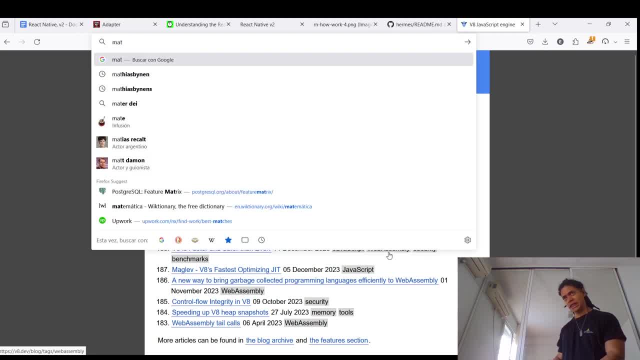 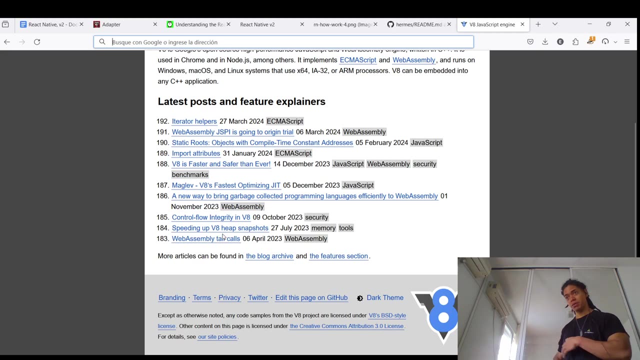 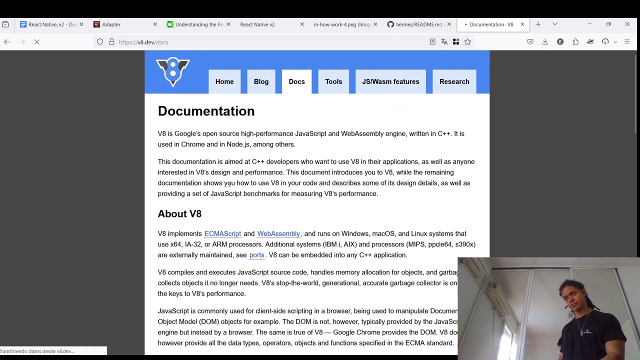 Death. here The thing is from matt Um. Holy moly this piece. No, it's like I i'm. the only way I can remember him is Um at the docks here. It's by looking at the v8 engine here. Uh, I think it is heating class. 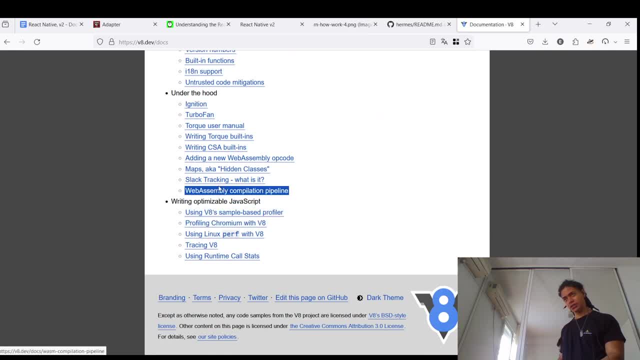 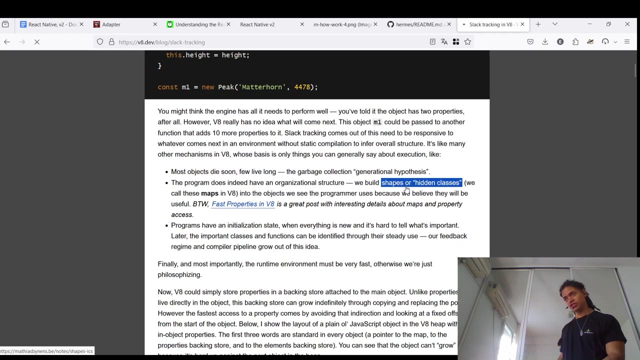 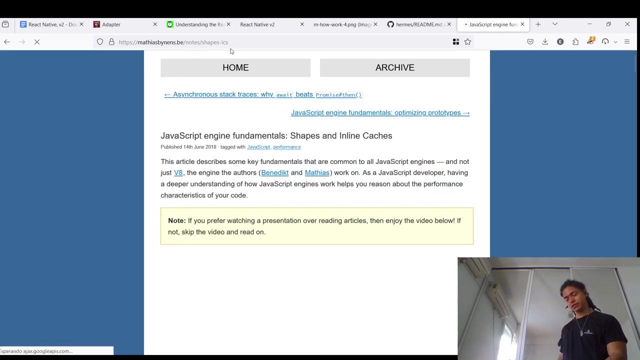 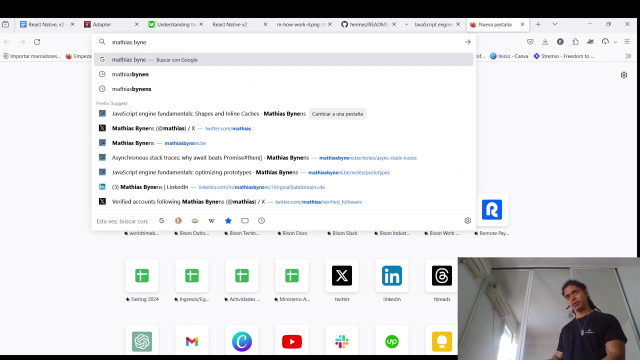 No, it's not hitting class. It's like tracking from Shapes or heating class Block From matthias Binds From Shapes or heating class Block From matthias Binds From Matthias. By binding Exactly from matthias. bind From matthias. bind From matthias bind. 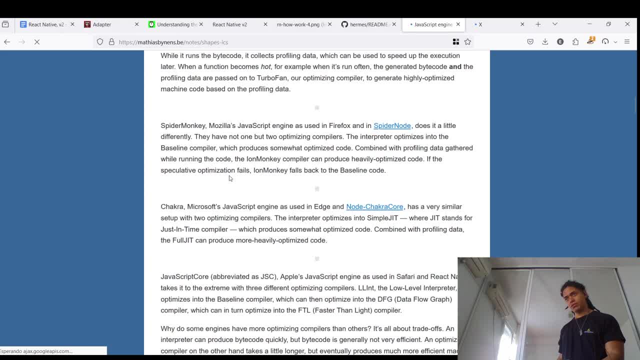 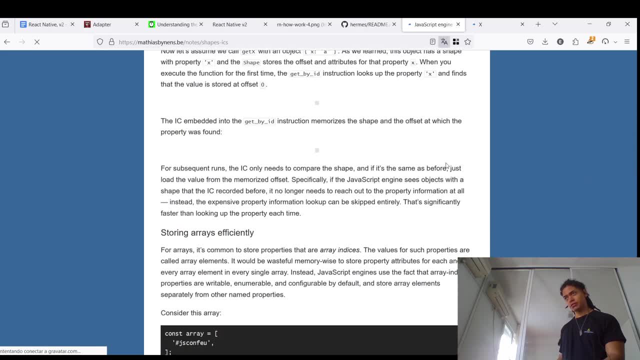 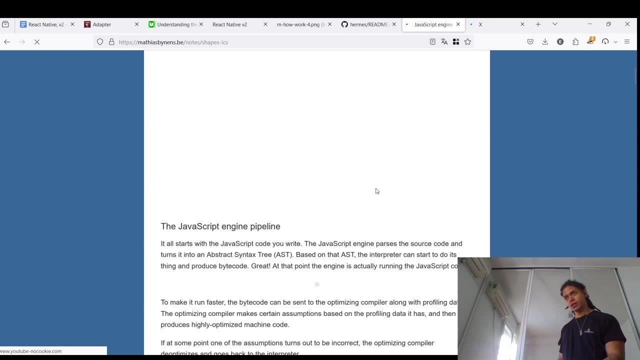 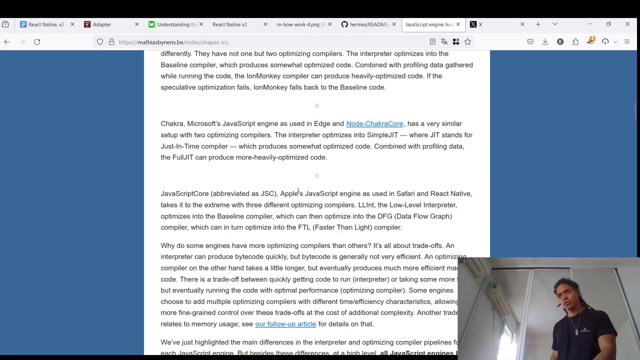